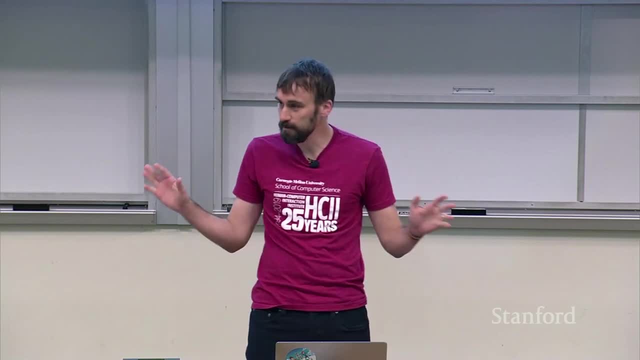 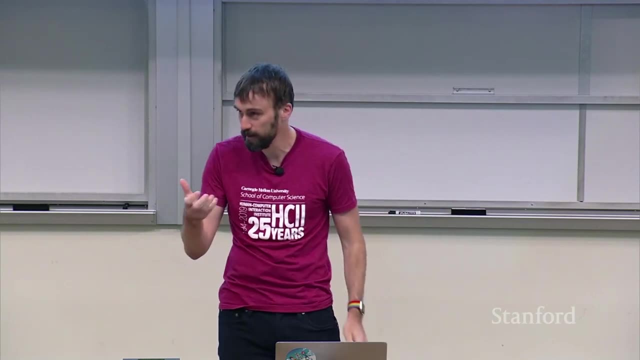 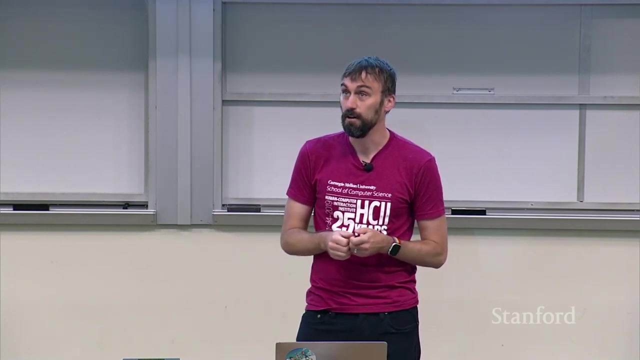 a disability And, having walked around a little bit on the Stanford campus, I can tell you that there's a lot of people experiencing what we would call situational impairments right now, looking down at their phone, walking, maybe, driving, riding the bikes with their phone, and whatever else you're trying to do. I think that's really. 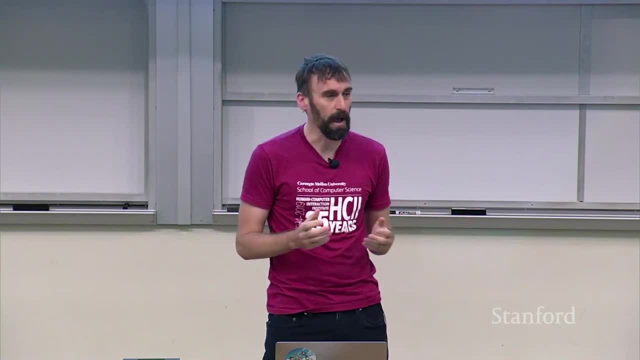 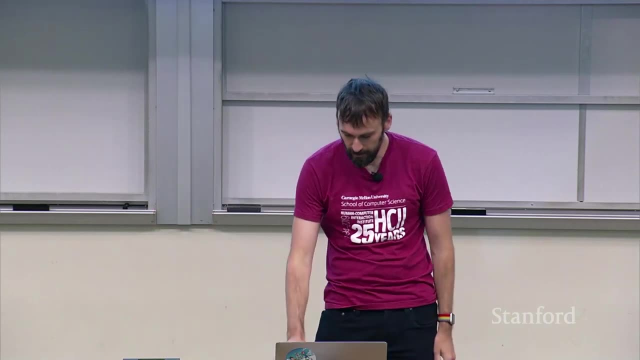 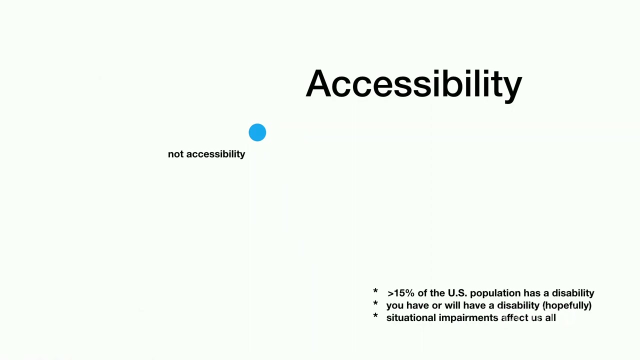 important too. but I really push back on this notion that accessibility is niche, that it's kind of this narrow thing. I think accessibility is very big and so this little dot, this dot which I just had there and didn't explain, is not accessibility right. So this is the 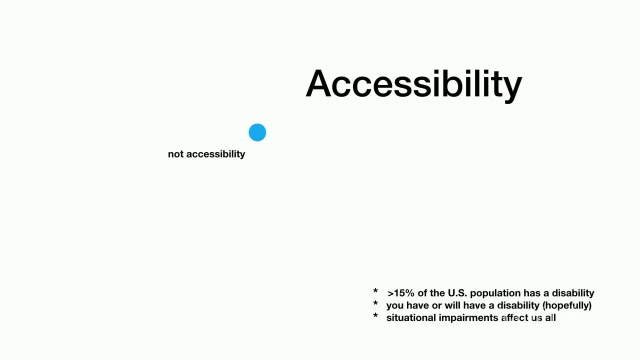 narrow set of interactions that we assume with our devices, that everybody has maybe high visual acuity and high motor dexterity and everything else is essentially accessibility, right? So getting you to be able to interact with any other set of abilities is kind of. 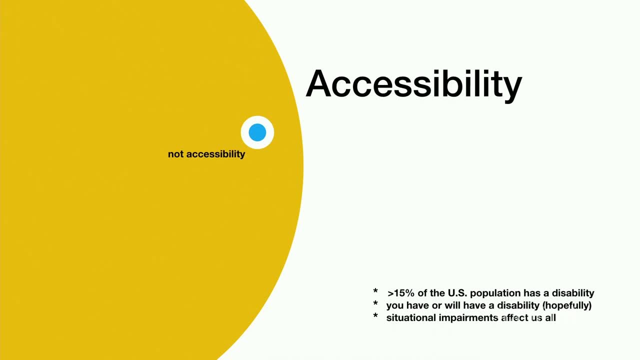 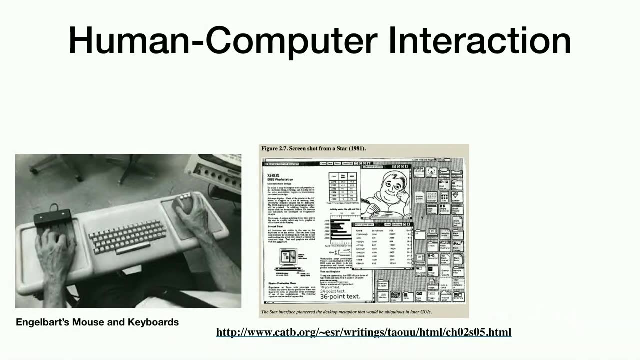 in this domain of accessibility, And so, for me, accessibility is very intimately tied to human-computer interaction as a field, right? And so if we look at some of the things that we're talking about, we're talking about accessibility, some of the really great, innovative, important developments in HCI over our history. what 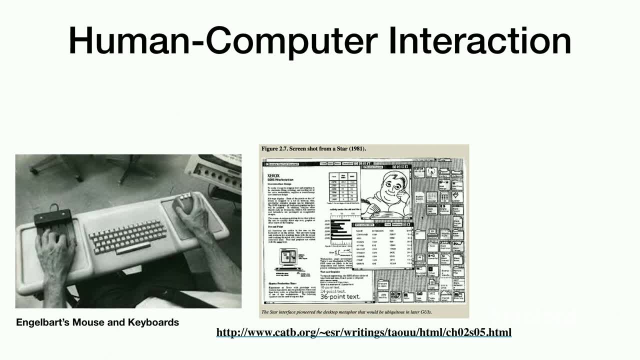 we see is not only the introduction of really amazing new interaction possibilities. so, for instance, you know Engelbart's mother of all demos, right? This is kind of what gets a lot of us in HCI super excited, and I'm super excited about it At the same time. 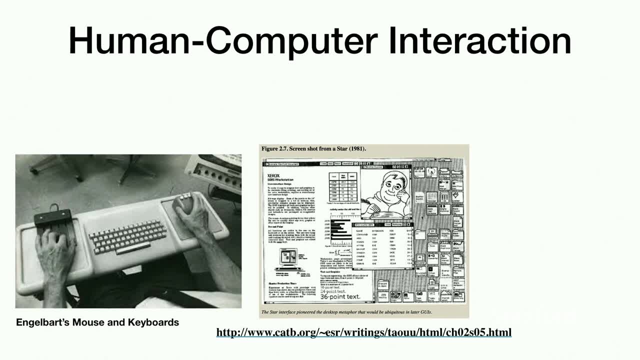 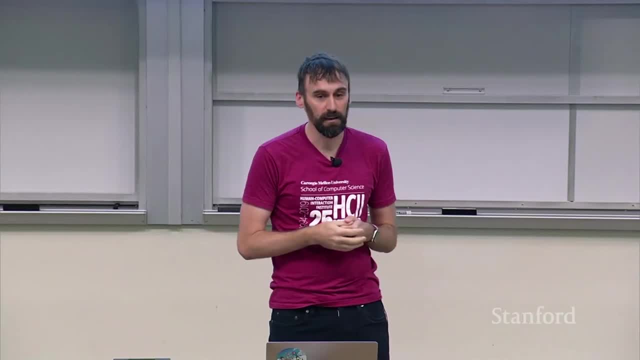 what happens when you introduce a mouse and you introduce a visual display and the graphical user interface. What you've done effectively is lock in a set of abilities that then we assume going forward, And that's really important. It was actually really important that we did that. 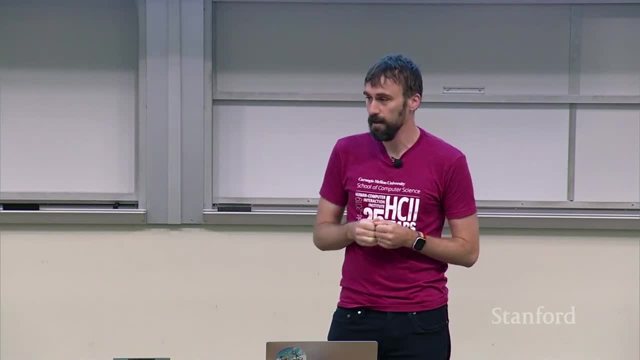 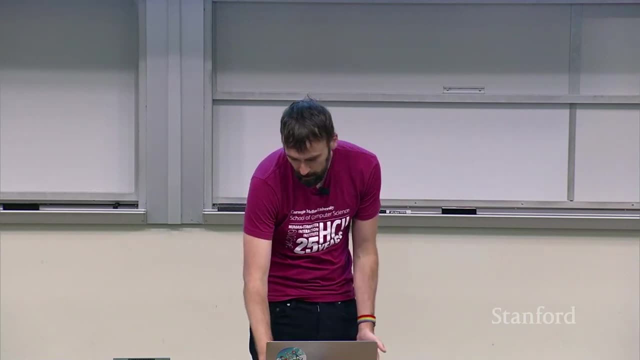 to make deep, sustained progress in HCI and it's been wildly successful. At the same time, these are ability assumptions that accessibility has to deal with And it keeps happening right. So you know. another really amazing development in HCI: introduction of the iPhone. 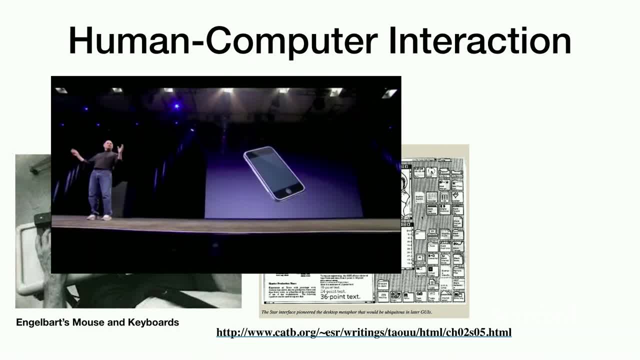 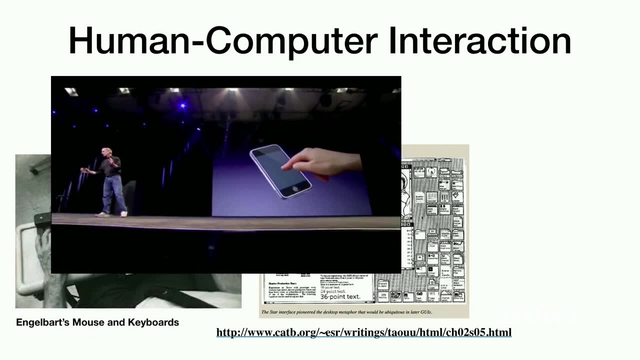 We're going to use the best pointing device in the world. We're going to use a pointing device that we're all born with. We're born with ten of them. We're going to use our fingers, All right. so introducing an iPhone, right? 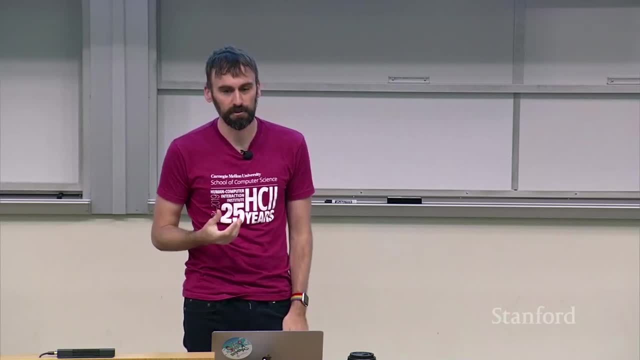 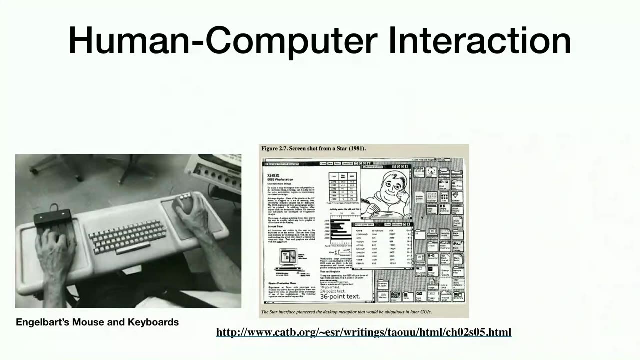 Use your fingers- Amazing new kind of interaction with our mobile devices. It works really, really well. At the same time, not everybody can do that, And so one way this has sort of been humorously illustrated is with this kind of- maybe you've seen this little figure or these kinds of figures before. 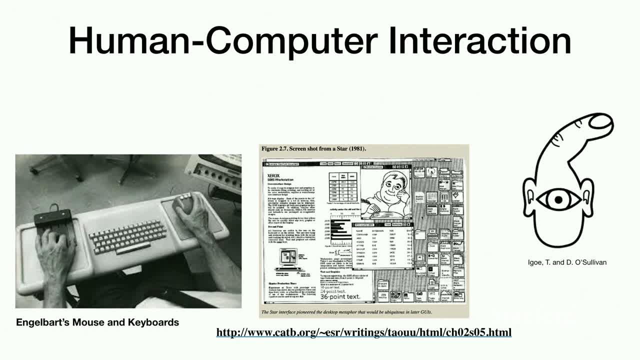 You have this. how does your computer see you? And like in this case, this is a little person here with one giant finger with presumably high motor dexterity, one eye that can kind of see flat surfaces, some ears that you maybe listen with. 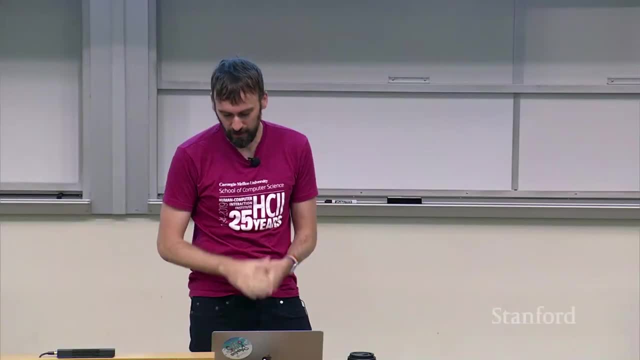 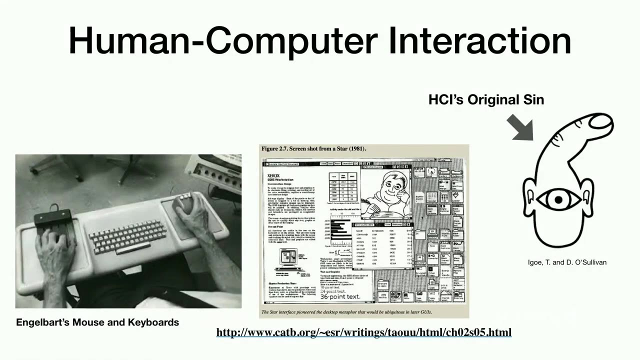 So one way I've started sort of jokingly but somewhat seriously referring to this is these sort of ability assumptions: are HCI's original scent right? This is what we've sort of been working against in accessibility now for years And so. 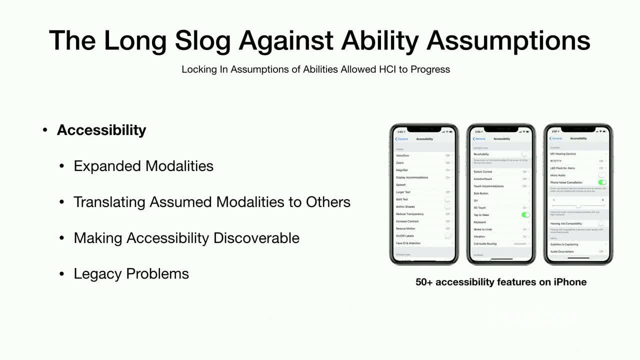 accessibility. one way of thinking of it is accessibility is the long slog against ability assumptions. So we've locked in this set of abilities. How do we develop devices that work in different ways? So some things that accessibility cares about. so the grand challenges of accessibility. 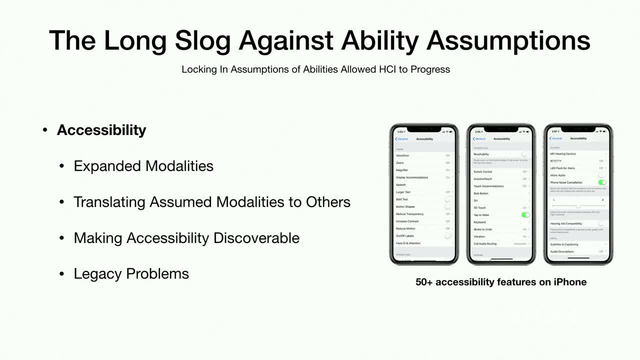 We care about expanding into new modalities, right, And there's lots of people working on. well, let's say we didn't. someone can't use a touch screen, someone can't use a keyboard, can't use a mouse. What other kinds of modalities can we use? 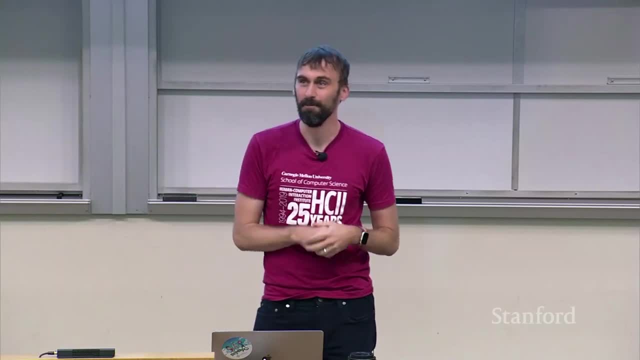 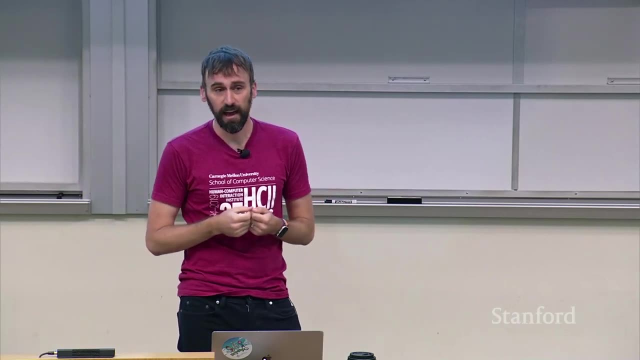 So tactile input, for instance, I got to see some really great examples in Sean's lab. The other is, for better or worse. we do have all of this stuff out there that assumes certain abilities, and so we need to be able to translate between it. 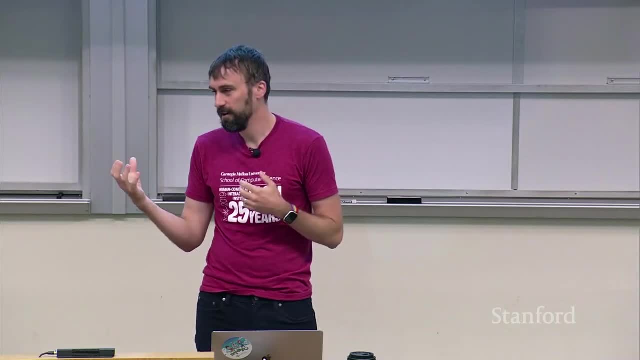 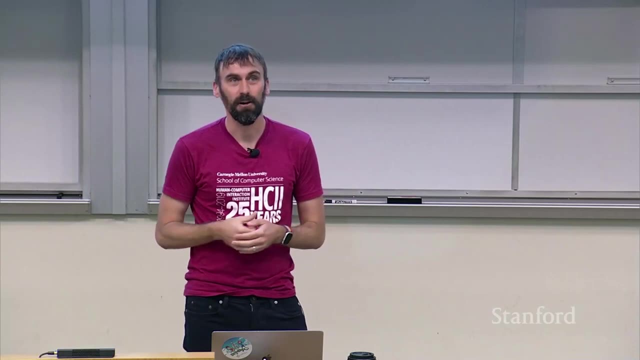 And I'll go into a little bit more about why that is. But if we have something that is assumed to work in one way, how do we make it work in a different way As we develop more and more features? so I think it's really great that a lot of 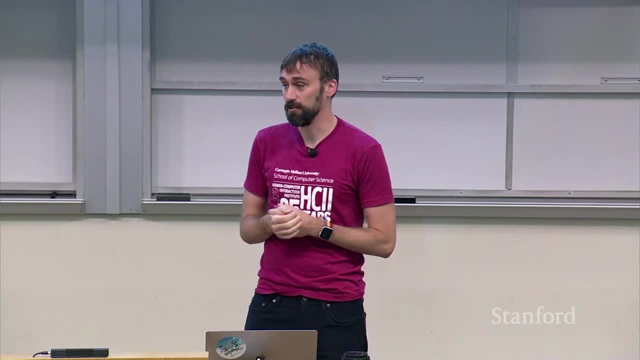 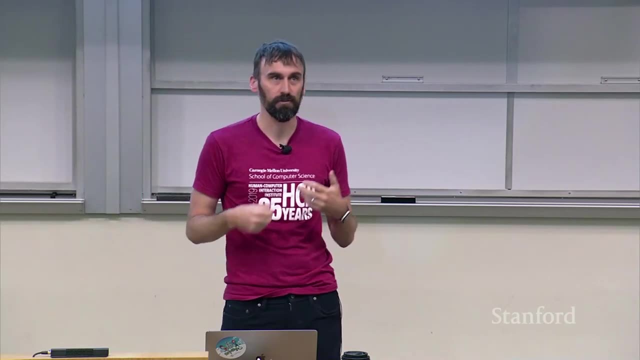 devices like iPhone has 50 accessibility features that change in all kinds of different ways How you use it, But how do people know about those right? Do people know what set's gonna work for me? And then even if we come up with really great solutions, 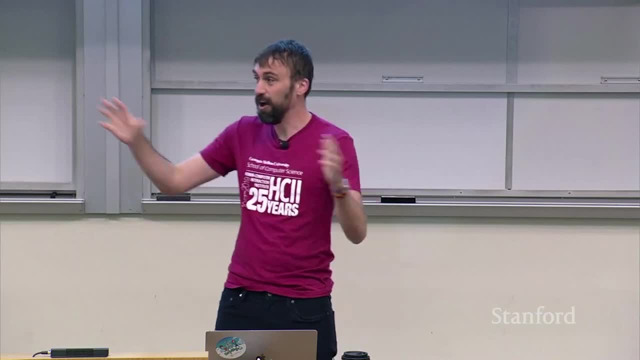 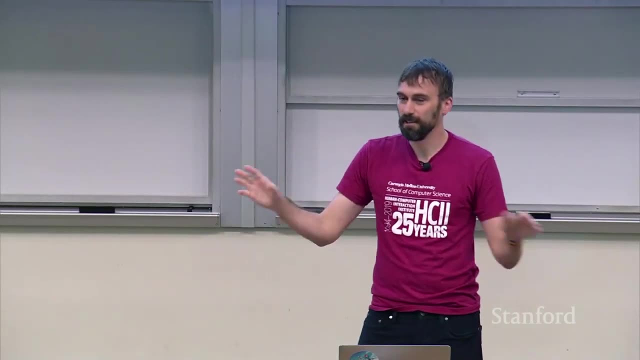 there's this immense legacy problem, where all this stuff is just out in the world. I don't even know, I haven't actually played with it, but there's a whole panel in front of me, right? This almost certainly isn't accessible in all kinds of ways. 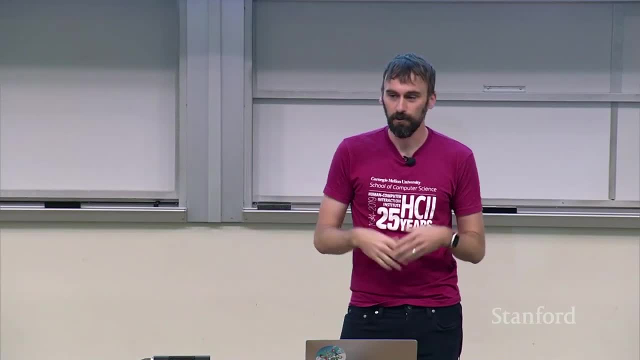 Are we gonna replace every single panel, replace this panel, replace all this stuff? There's all these books that are printed, that everyone's lost the digital version of. There's lots of legacy problems out there, so how do we deal with that? 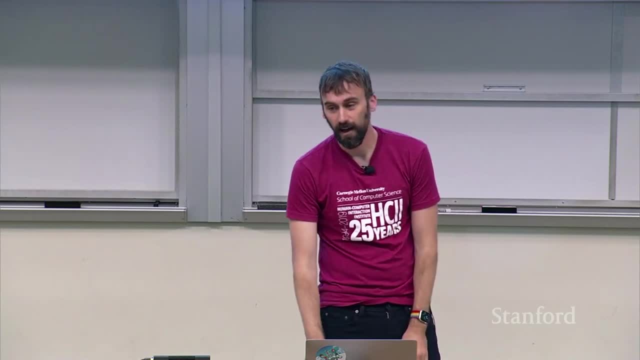 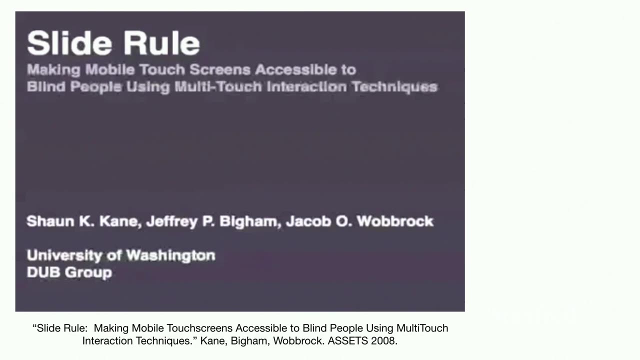 So when new technology is introduced, one thing we do in accessibility is kind of race to figure out, well, how are we gonna make that accessible? And so this is kind of an old example, but I really like it. It's a project that I worked on with Sean Kane and 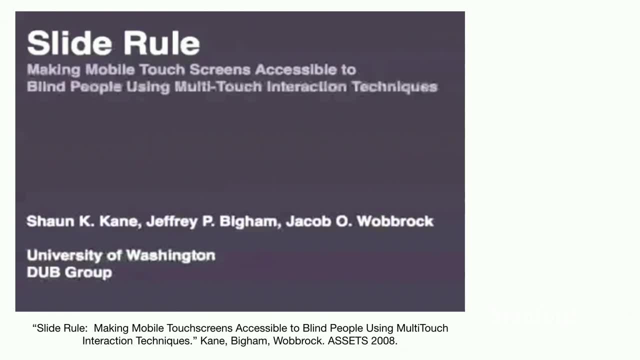 Jake Wobrock when I was at the University of Washington about 12 years ago, And the idea here was that, you know, the iPhone would come out and we really wanted to be able to use it non-visually, right? So at the time, 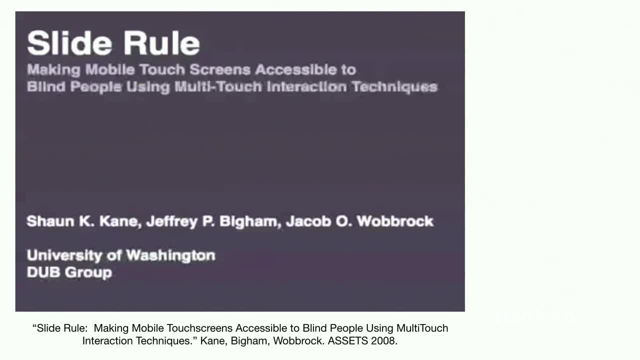 there was no screen reader on it. This has all changed now, but how are we gonna do that? And so we developed this system called SlideRule. I'll play a video of it working. Takes a second. I think We're gonna open up this SlideRule app and 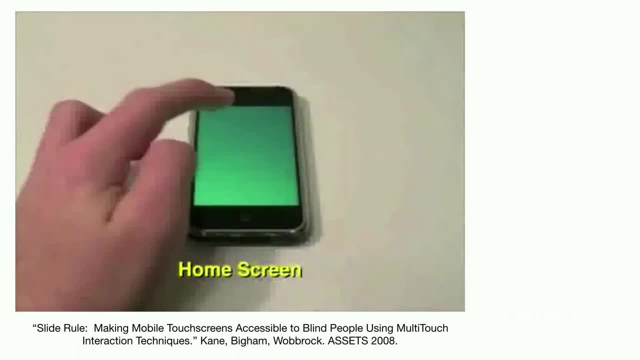 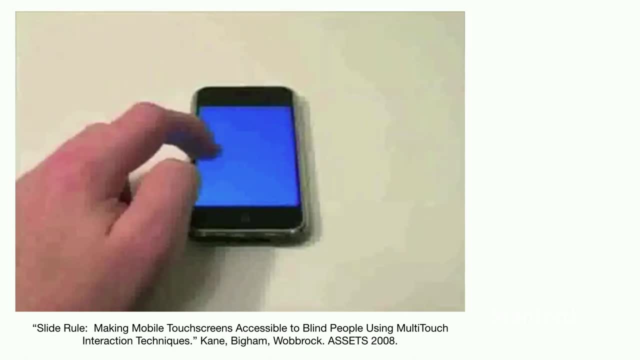 Hey, I'm paint half up Uranen: two B Bill Cosby. three F, Frank Sinatra, Jay Jay, Jay, Jason Jay, Nicole T Dom, Made out of 10 calling Woody Allen. So the couple of things that this does. 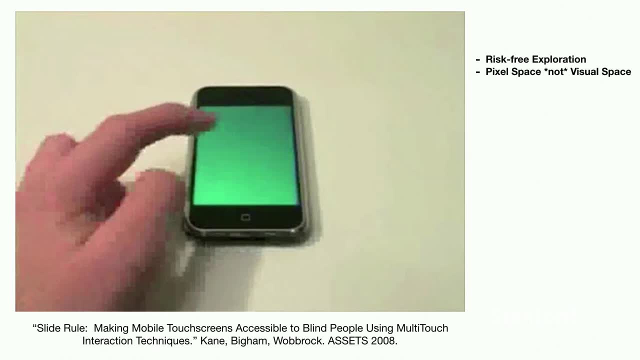 right. So it repurposes this touchscreen as a touch sensitive surface. It allows you to explore with your finger and, importantly, it introduces this idea of risk-free exploration. So now, moving your finger around doesn't activate things. It allows you to hear what's under your finger. 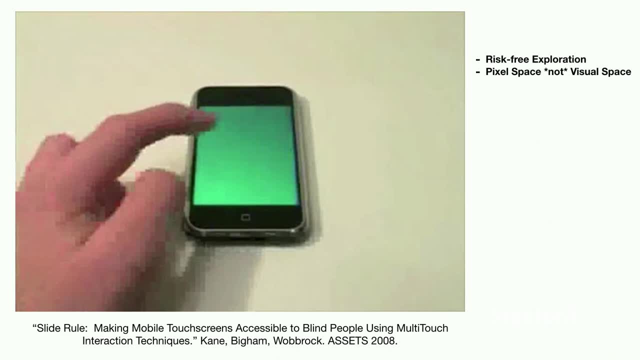 and that makes you the reader. So now, moving your finger around doesn't activate things. It allows you to hear what's under your finger, And then we use a second tap to actually select that thing. One of the other things we noticed is, once you are freed from this visual space, 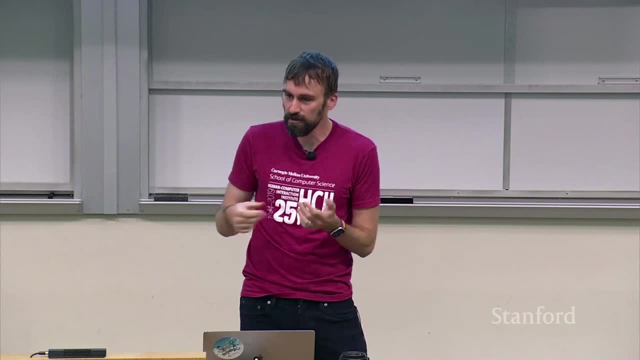 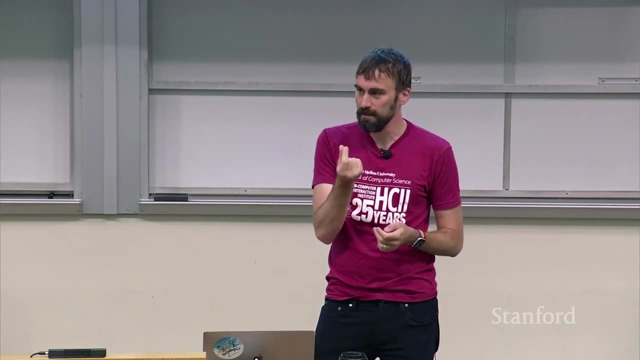 of the existing graphical user interface. you can actually fit a lot more stuff on there. So I don't know if it was obvious, but when he was going through the phone book, each item in the phone book is now the pixel or the input resolution, as opposed to the visual resolution. 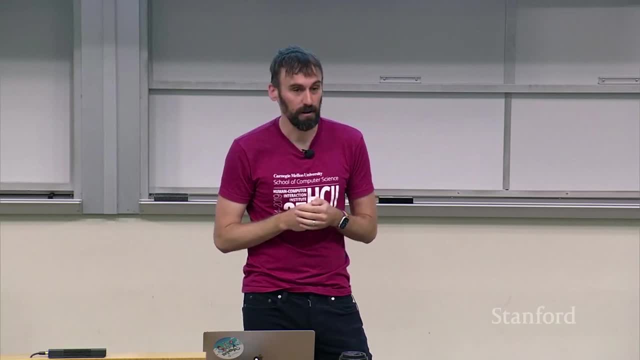 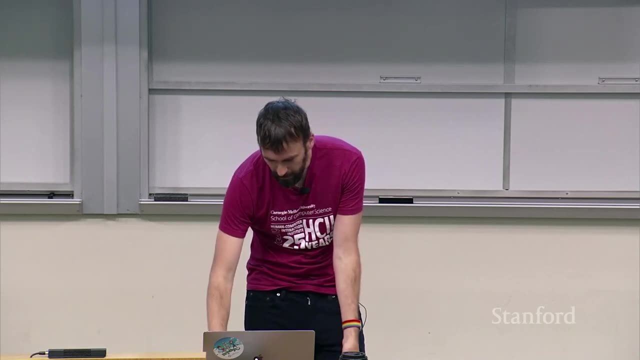 So you could actually fit a huge phone book on a single screen as opposed to having to scroll around Anyway. so this was really fun, And it's just an example of how do we adapt or how do we think about using some of these devices in different ways. 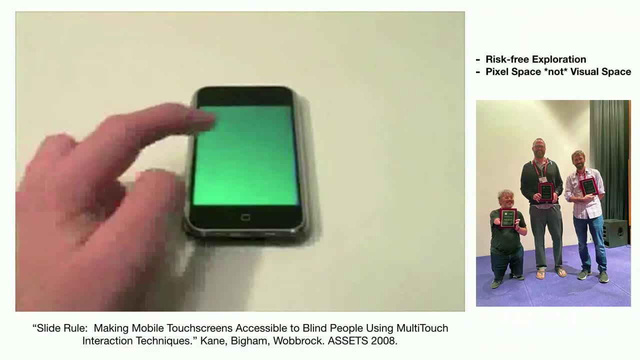 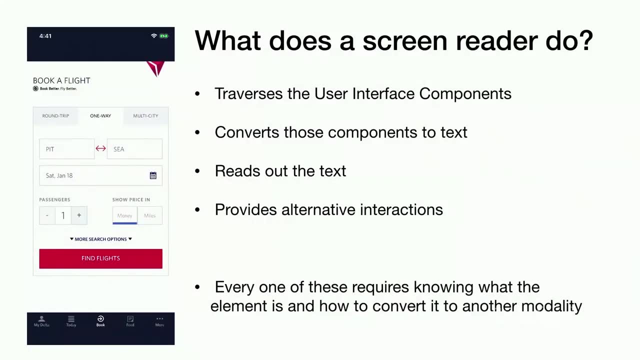 I have a fun little picture. We just got the Impact Award, the 10-year Impact Award, at Assets, And so this is Sean, Jake and me holding up plaques, Anyway. so now this sort of interaction, or some of these ideas from this sort of 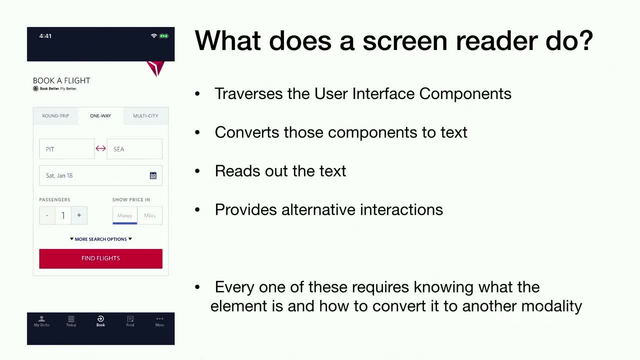 interaction are available on your iPhone, on your Android phone, And it's embedded in in a program we call a screen reader, which allows non-visual access to an otherwise graphical user interface. And so it's got this name: screen reader- Because at least initially in the development of screen reading, 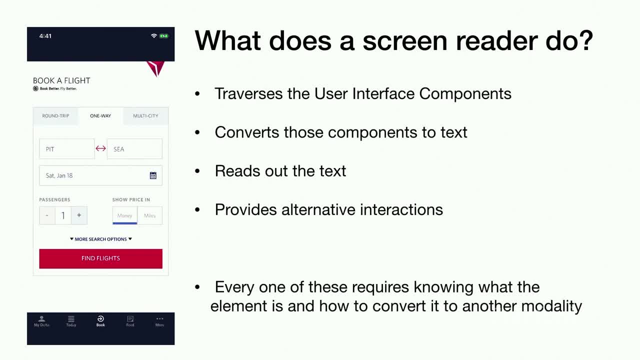 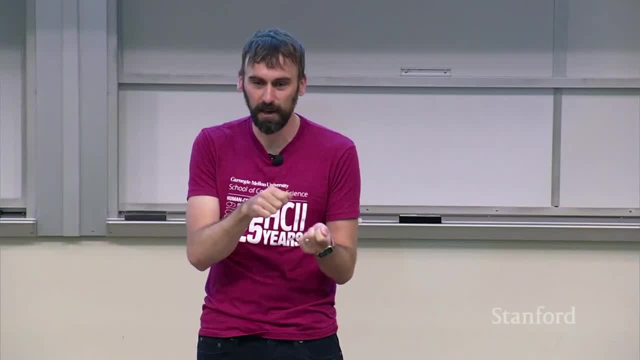 technologies. the idea was that software- people would build software And it would literally intercept the pixels that were being written into the screen and sometimes into the screen buffer. Sometimes they were able to get it before it was turned into pixels, like text, before it got turned into pixels. 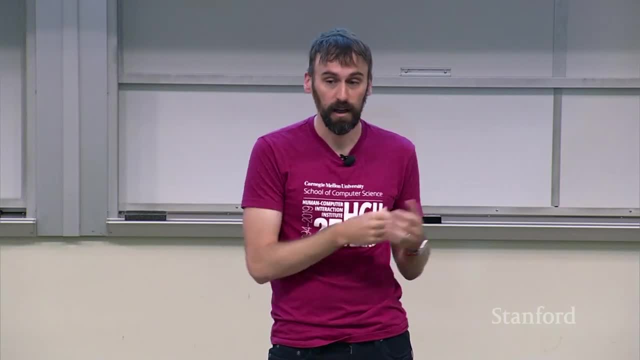 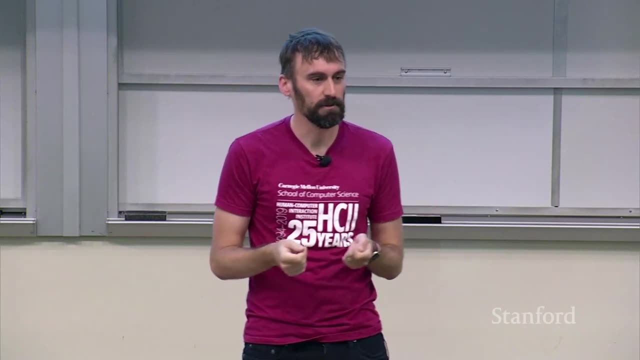 And it would then convert it to speech, as you'll see here. see her in a second or refreshable braille. So not all assistive technologies are screen readers, but I do think it's really helpful to think about, well, how does a screen reader work? Because 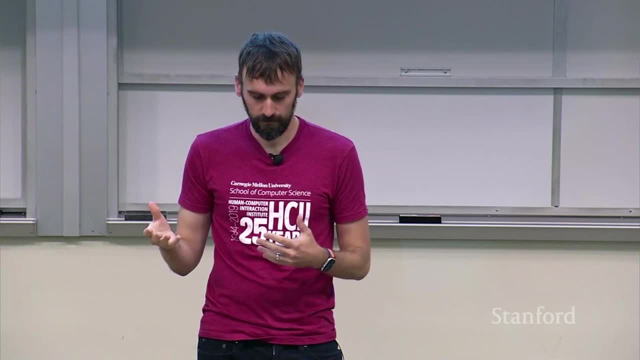 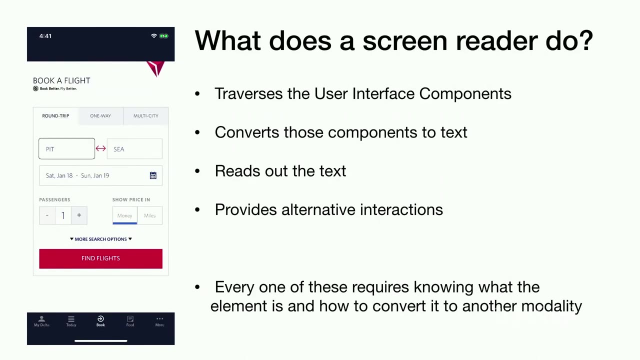 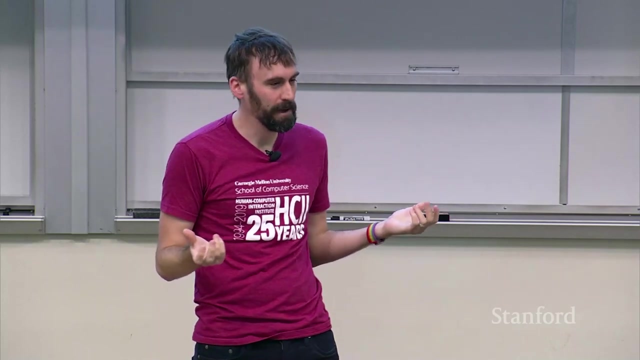 some of the ideas translate: Oh, it already points to it. Okay. well, here's a screen reader reading this Delta app, which I use a lot. So, at a high level, right, it comes up with some sort of- you know- representation of the graphical user interface. If you've ever built a web page, 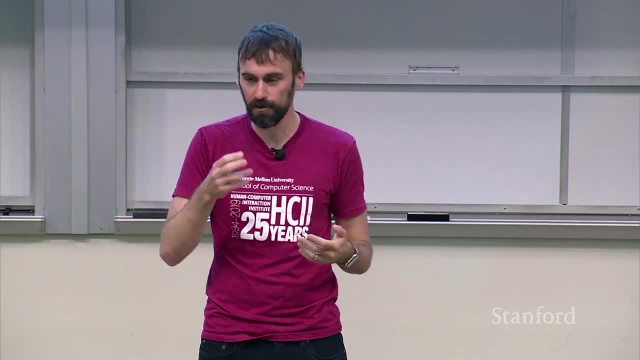 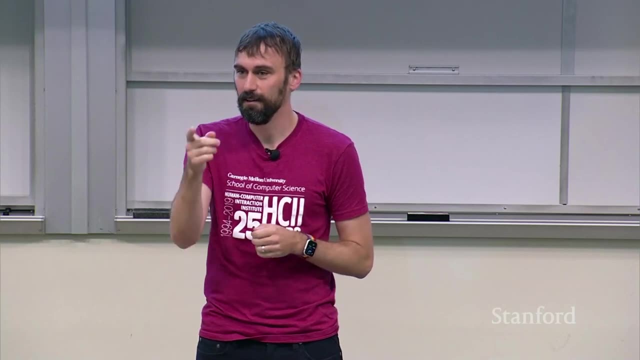 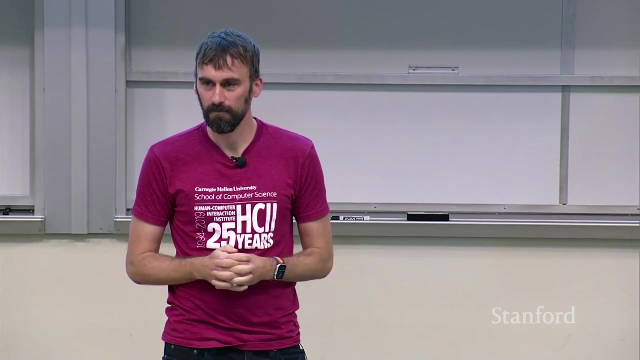 you might think of this as sort of the DOM of the user interface, and then it traverses it. If it's a tree, then it's a depth-first traversal of the tree. Who has a question Shows the focus of not all assistive technology but a lot on, you know, changing the GUI to voice. 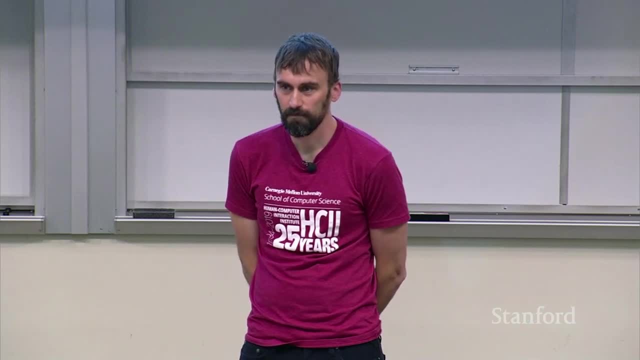 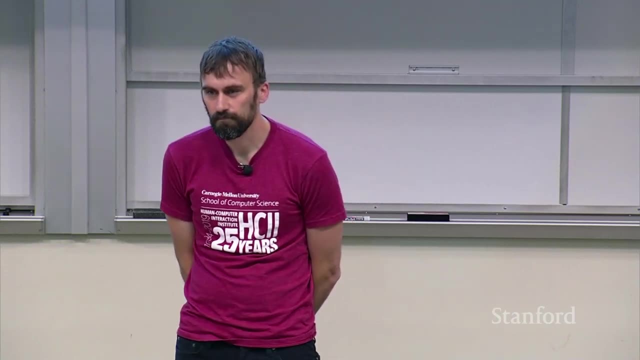 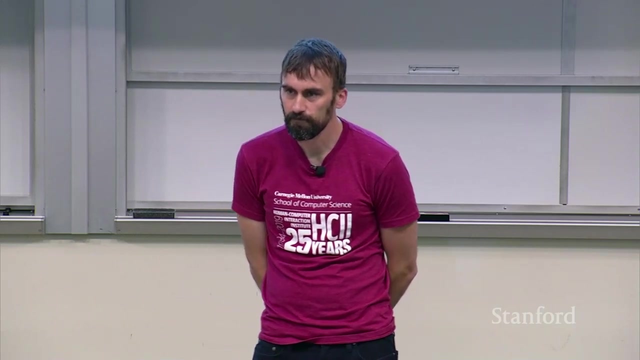 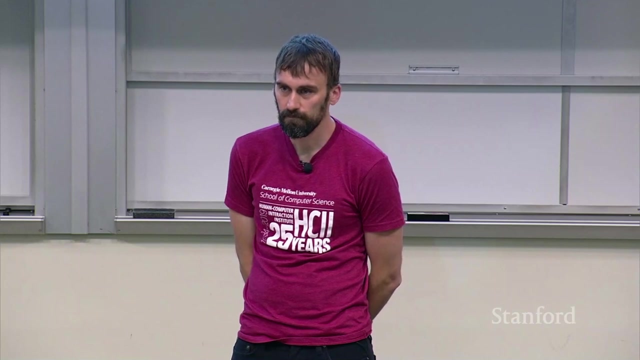 a result of just. I guess that transitioning from a textual interface to a GUI cut off a lot of visually impaired people who had found employment in that area because it actually fit some of their skills better. Or is it due more to this? is the biggest different ability in the population, or easier? 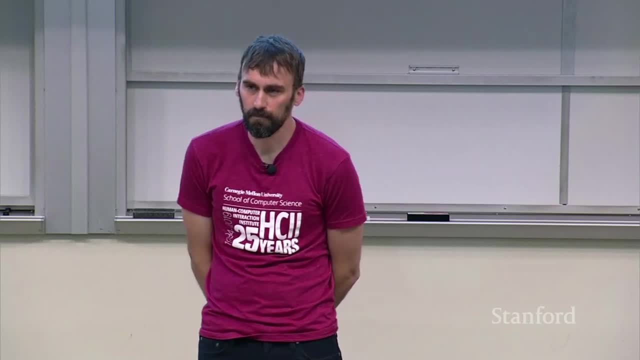 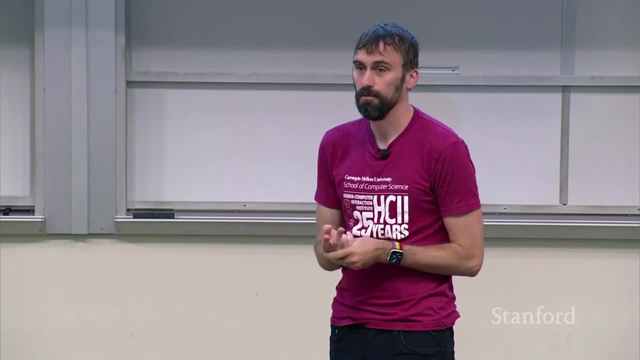 to attack. Like I'm curious whether you know. obviously, as people age we start to see people getting worse, So it's kind of broader than just, let's say, low vision, blind people, or are there other you know? 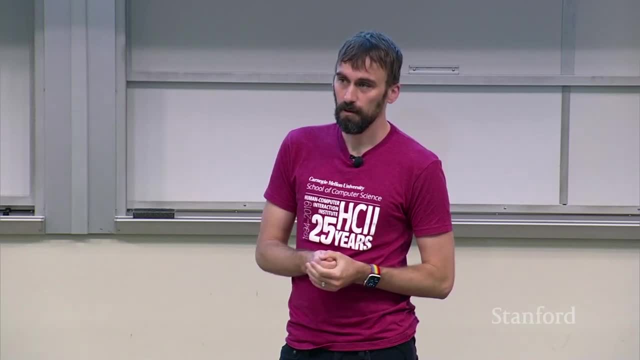 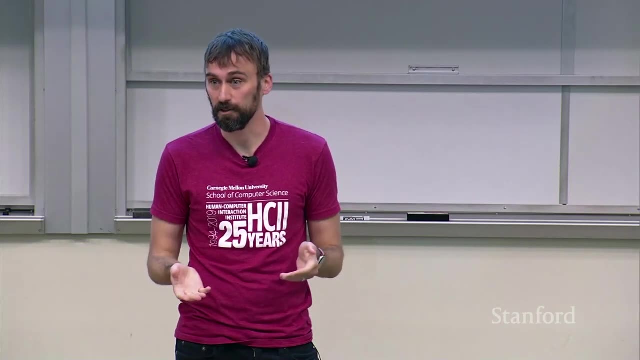 motor and other impairments that are bigger. Yeah, so these are really good set of questions. So one is: why do we focus, or why am I talking about screen reading? One reason is because I think it's one of the quickest to understand of. 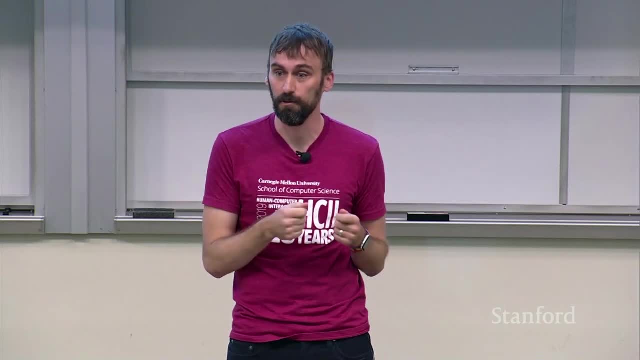 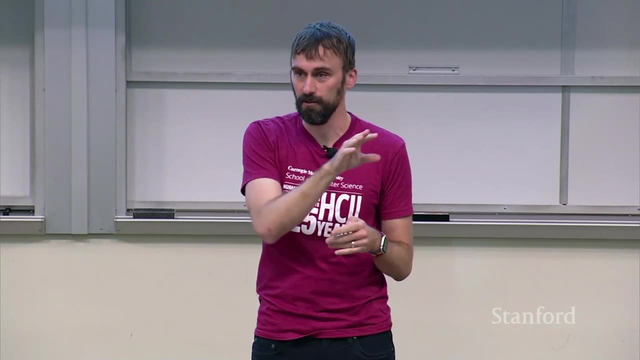 you've got this graphical user interface- usually you don't have to convince people too much that a person who's blind can't see that- And then thinking about: well, how do you convey that information? And you've got this underlying representation and you have to somehow convert it to voice. 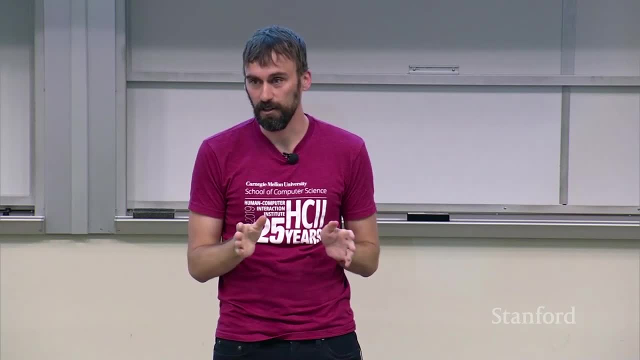 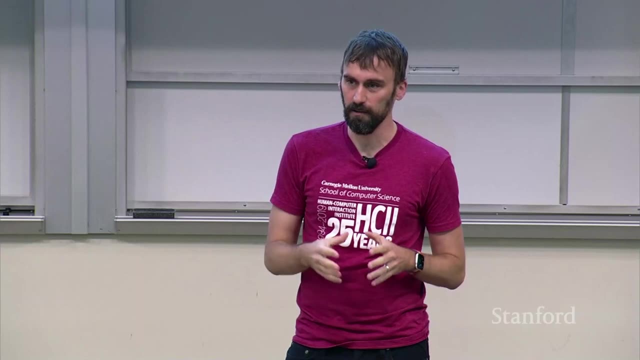 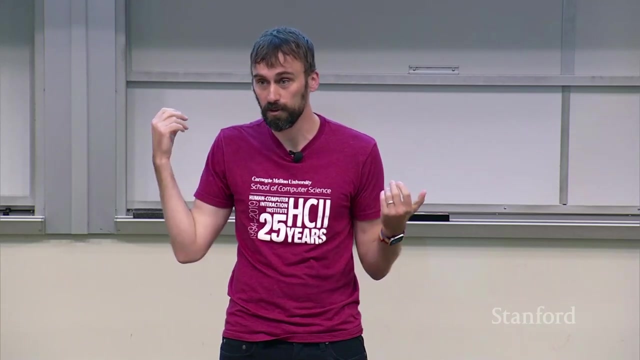 Many of the other kinds of accessibility features that you might have. so I mentioned, you know, however many on all your devices work using many of the same underlying things, right? So if I am somebody who is a switch control user, for instance, who I have a set, one or more, 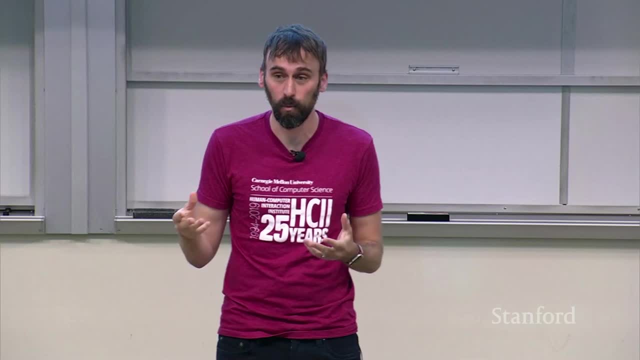 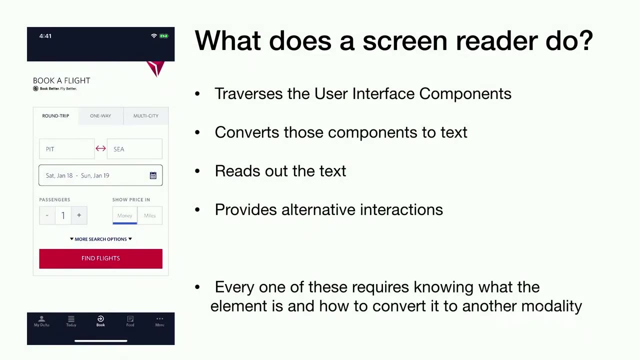 switches that allow me to go through the user interface. it works actually in a pretty similar way where, instead of you know voicing things, it visually shows me I can see a progression across you know different possible user interface elements and then I can. 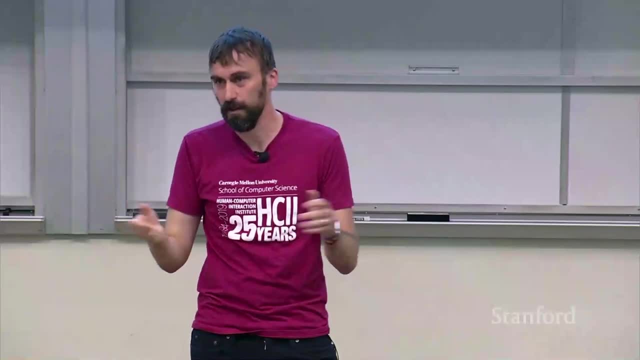 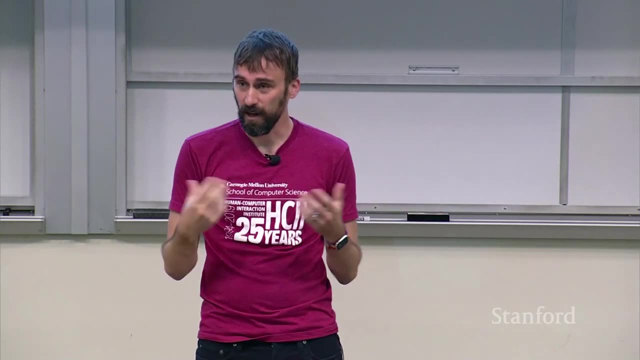 choose how that progression goes and I can choose which one I want to select And there are others right, So we obviously there's ways to change how touch works, how, what kind of motor dexterity assumptions there are. there's endless features for magnification, for changing colors, for doing 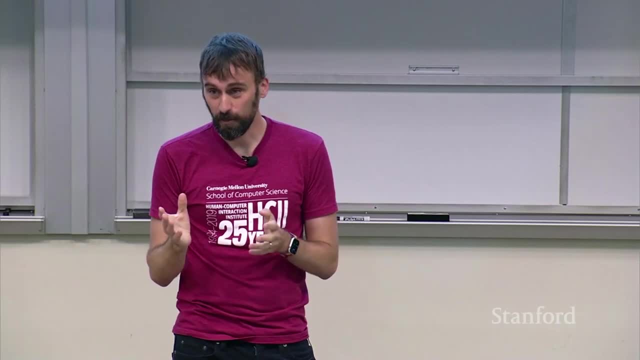 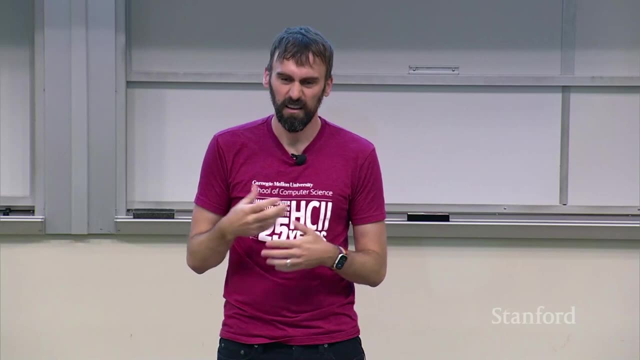 all of these sorts of things. So there was a big switch from when there were text-based- you know, text-based, you know text-based things, There were text-based interfaces like command line interfaces, where it was at least there. 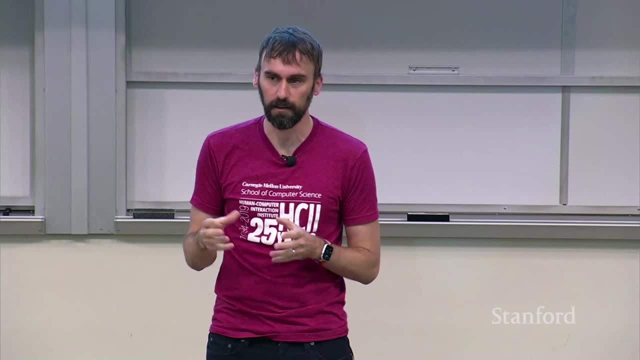 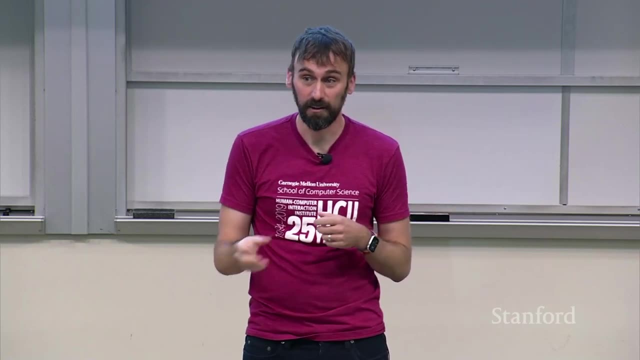 was obviously still some problems, but it was a little more straightforward to create like a screen reader experience for a text command line interface. When you go into graphical user interfaces, at least initially, a lot of the semantics were just gone in pixels, right. 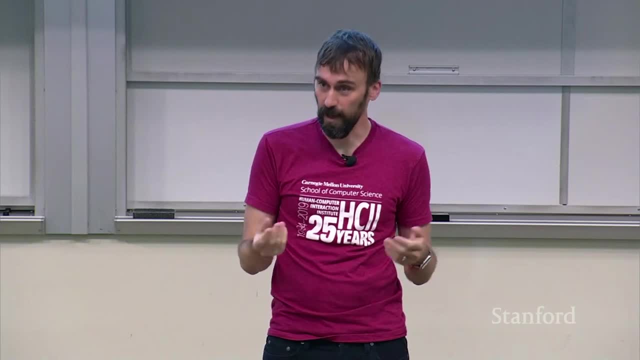 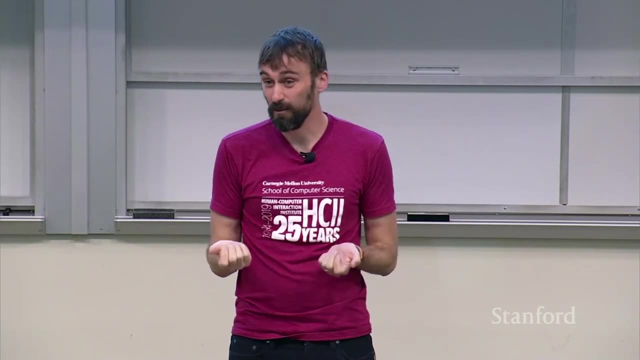 And then there's been decades now, I think, to reverse some of that, where you have access to a better representation of the GUI that you can convert to different forms. I think the reason why we focus on text-based interfaces is because you know there's a 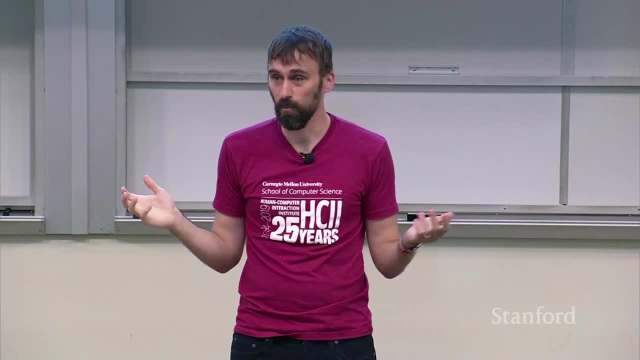 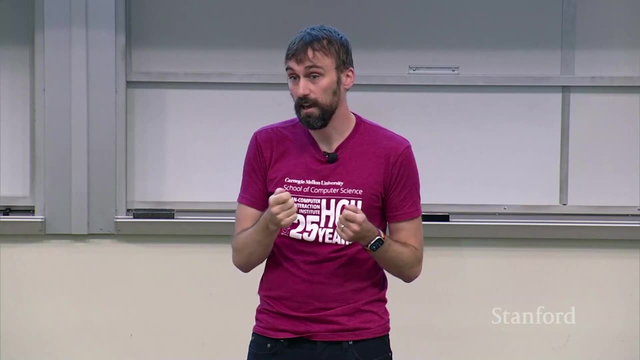 lot of. we focus a lot on GUIs is because this is still the dominant way that things are represented, right, And you find a number of examples out there where you could imagine: well, let's create a whole separate web page, and people do this, and it's always a bad idea to create a whole. 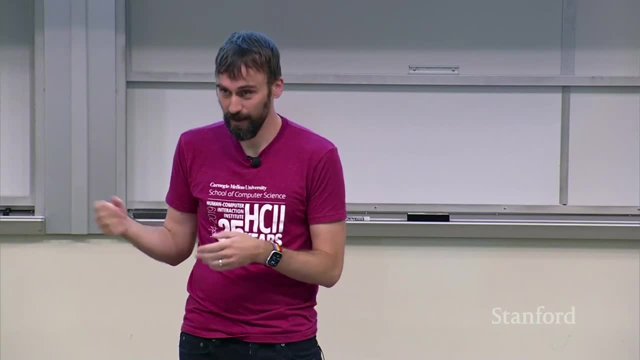 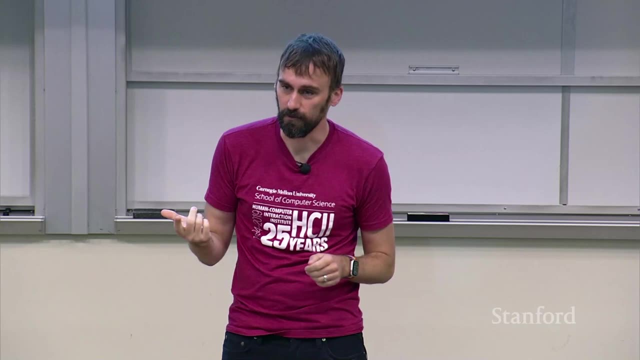 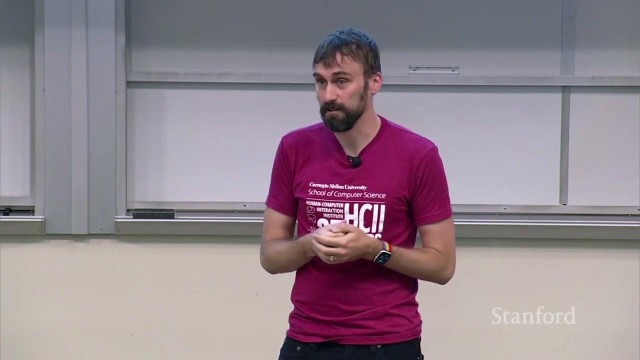 separate website for people who are using screen readers, for instance. This happens actually. this is Blackboard's solution for accessibility. Almost always, it works differently, you have access to different stuff, and so the trade-off that people have been willing to make, and I think it's important and it makes sense. 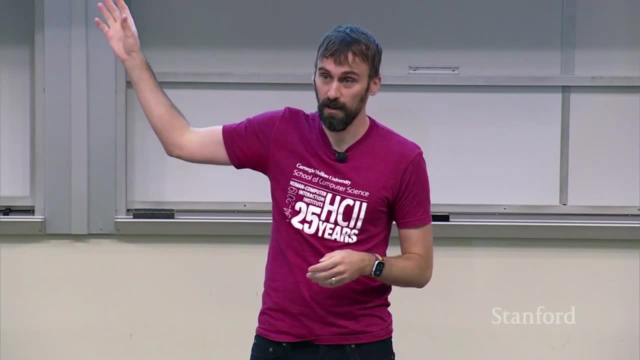 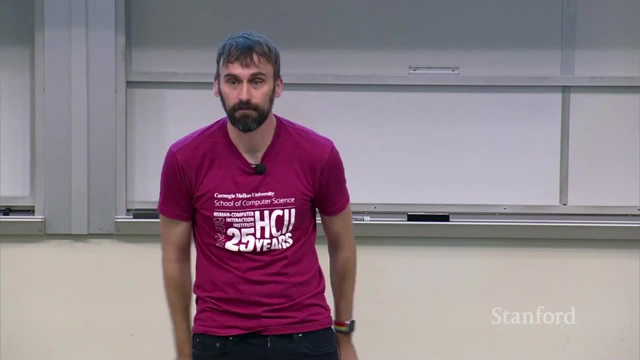 that they make it is to put up with these transformations, because at least that gives you access to the thing that everyone else has access to and that most of the focus is put on. Yeah, I'm curious: has anyone ever tried to sort of discuss or measure like what you? 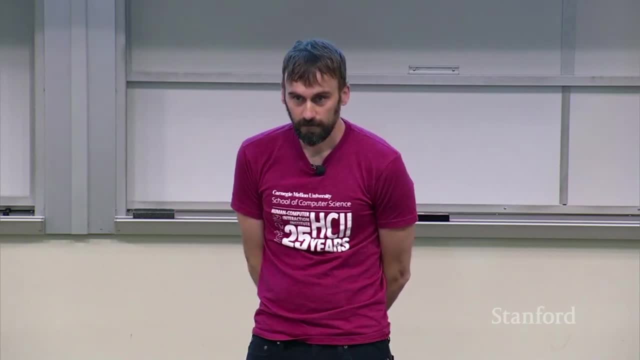 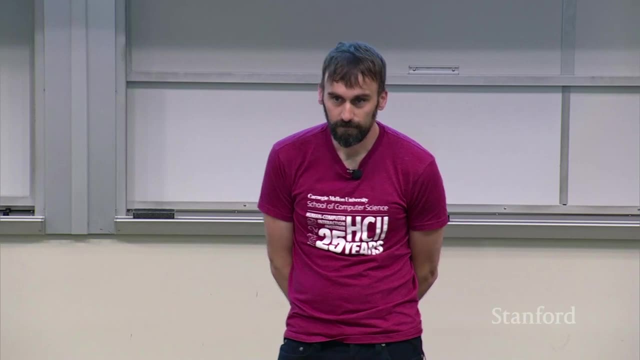 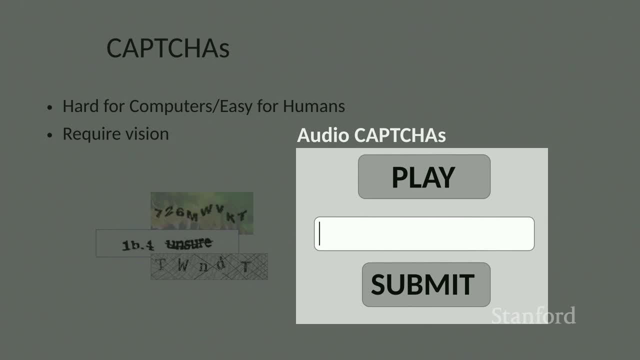 into a parallel world where you give me this app and then you also, you know, split me. Okay, How many numbers were there? Uh, I think there's more like 10.. I'll play it again. I'll play it again with the visuals. 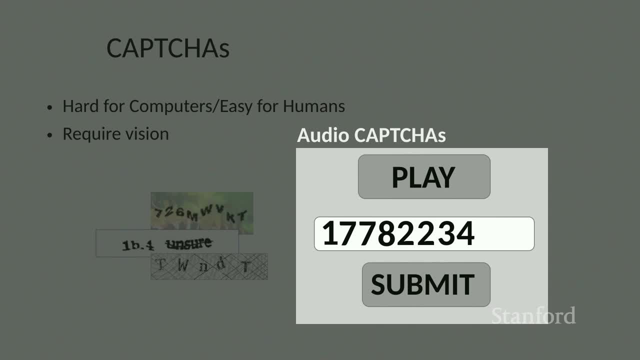 Showing I got behind a little bit, but anyway, I've been playing the same captcha for like ten years, So to me I just I know this one. So I'm always like, well, they can clearly hear this right. 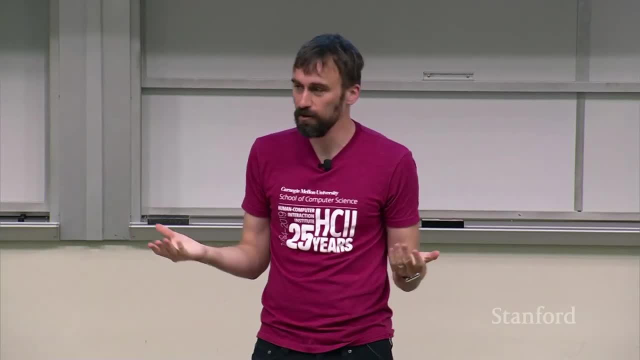 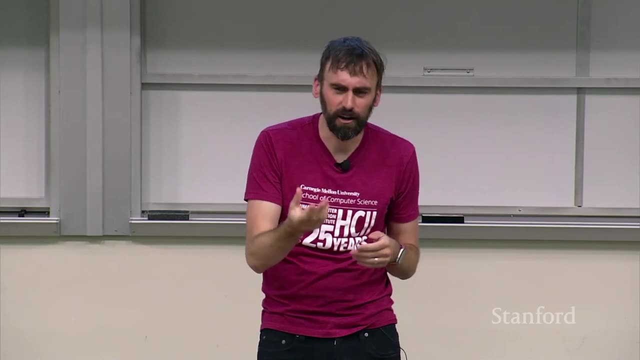 But anyway. so this and this is not an unusually hard audio captcha. Obviously, the modality change makes it different though right? So like I can't just keep staring at, like the particular part of the captcha I'm trying to figure out, until I reason with myself about what number it is right. 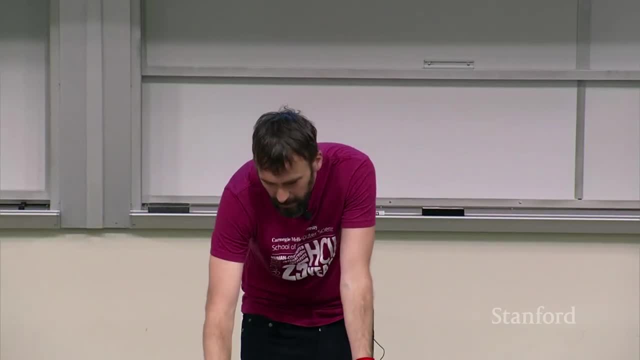 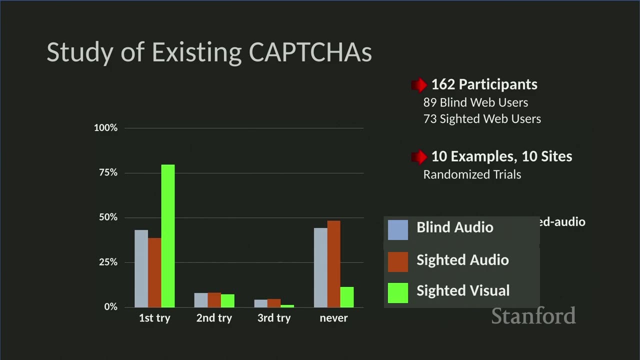 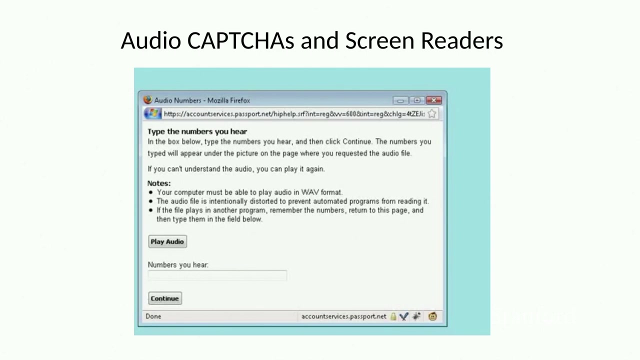 It goes by right, Anyway. so we did this study and basically the audio captchas are a lot harder, not surprising. One trick, though I thought it was really interesting: the interface provided makes it even worse on people. The audio file is intentionally distorted to prevent automated programs. 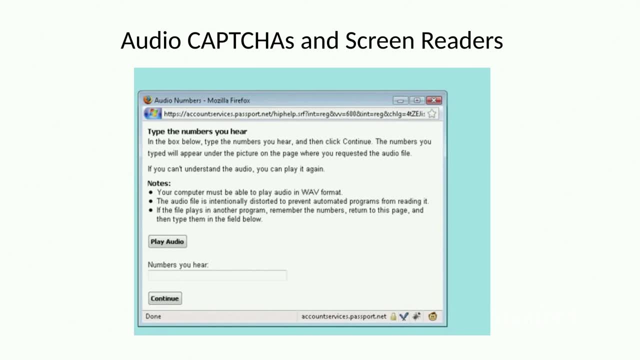 from reading it If the file plays in another program. remember the numbers, Return the file, Head to this page and then type them in the field below. Play audio button. Browse off Play audio button. Audio number: edit box. So anyway, just remember those ten numbers that you can't understand anyway. 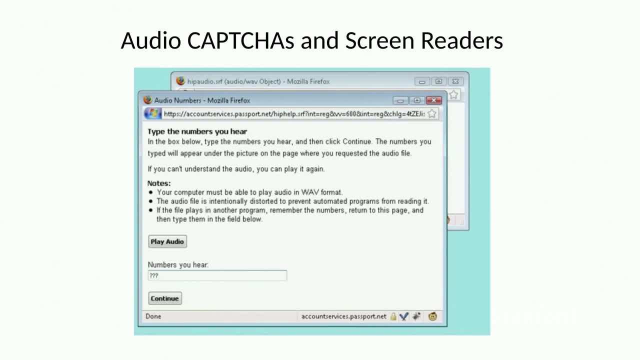 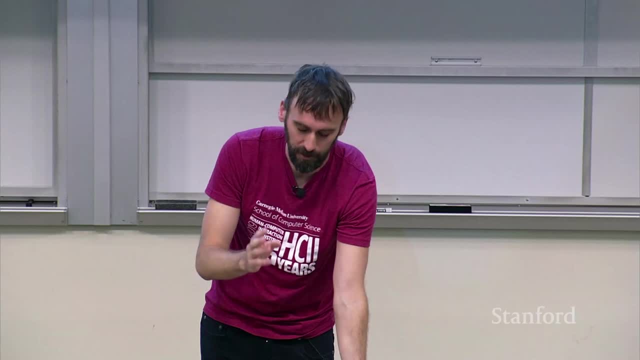 and then type them in the box later. Anyway, we were able to improve this a lot just by changing the interface. Basically made it- so there's not a different audio player- that you could be in the same box to control the audio playback. 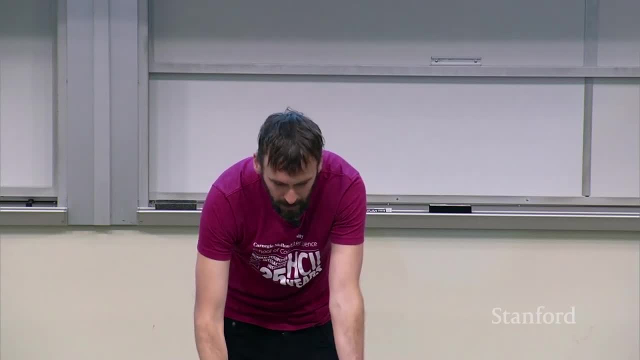 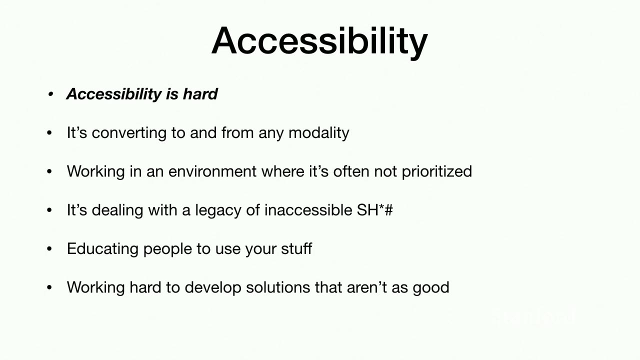 But anyway, it just kind of keeps coming up these things. So takeaway here, right, Accessibility's hard. It means a lot of different things. It's this huge space And I think it gets less attention than it should. It's converting to and from any modality, right? 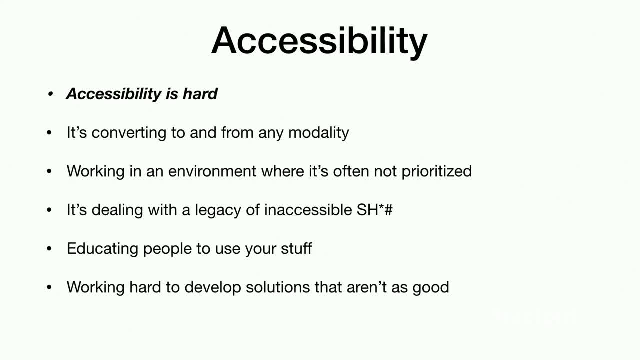 So, basically, if you want to accommodate any ability that people come with, you need to be able to convert between modalities pretty fluidly. It's working in an environment that's often not prioritized. It's dealing with a legacy of inaccessible stuff. 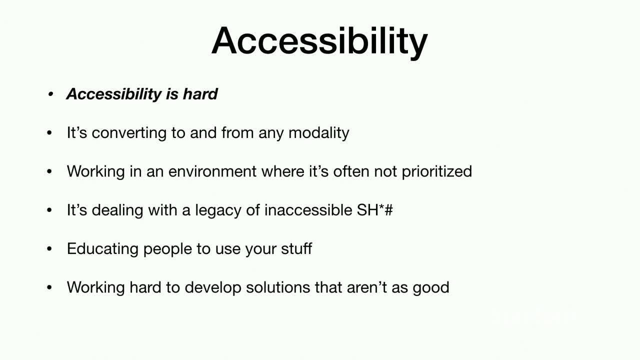 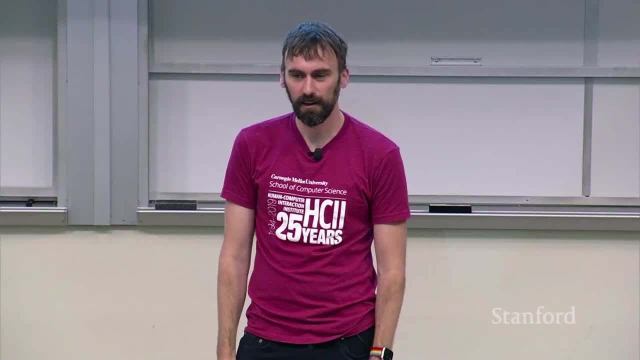 Educating people to use your stuff. How do people find it? And then sometimes it means working hard to develop solutions that aren't as good as what you could develop if you targeted the ability that you're converting to in the first place, which is tricky. 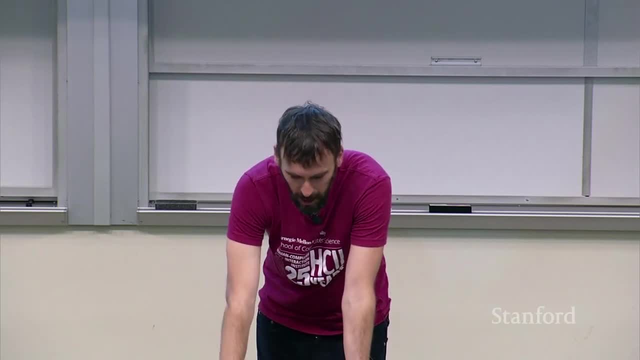 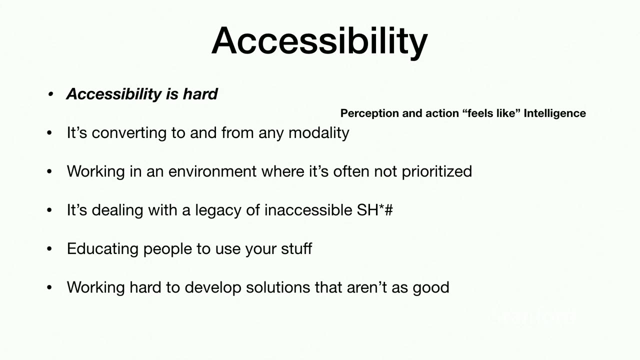 So if we now connect this- I'm trying to bridge over to AI here- Perception and action feels a lot like intelligence, and so there are actually a lot of connections between accessibility and modality changes. If it's not prioritized, you need to get everything out of the little bit of. 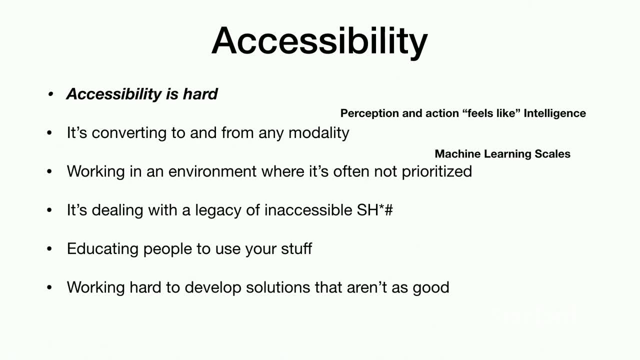 input you have, And so machine learning that scales is actually pretty important. Again, legacy: there's a huge amount of legacy stuff. Even if we made everything accessible from now forward, there'd just be so much out there, And so scaling with machine learning is important. 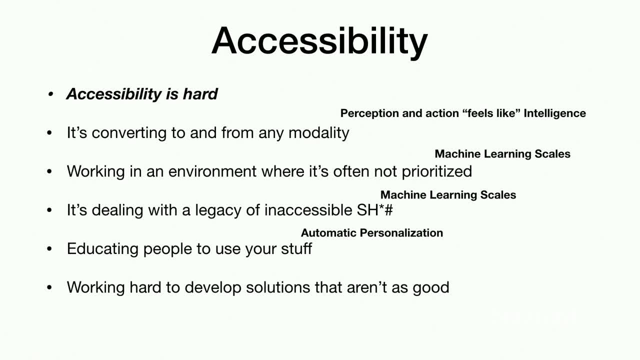 Potentially automatic personalization and working hard to develop solutions that aren't as good. Well, AI is magic, so it'll be great. A little bit less sure about that one. All right, so just a few points, and I don't actually have that much time. 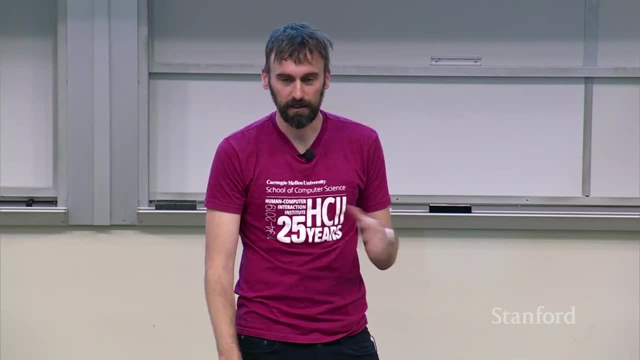 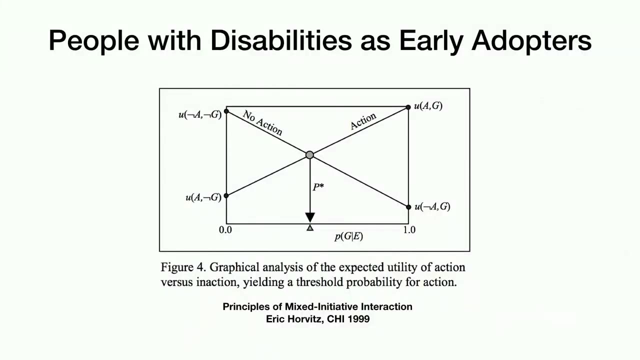 So I'm just gonna run through Some of these points about where I think these things intersect. So one I like to say that people with disabilities are often early adopters, The earliest users of technologies that are in kind of AI, ML, space for. 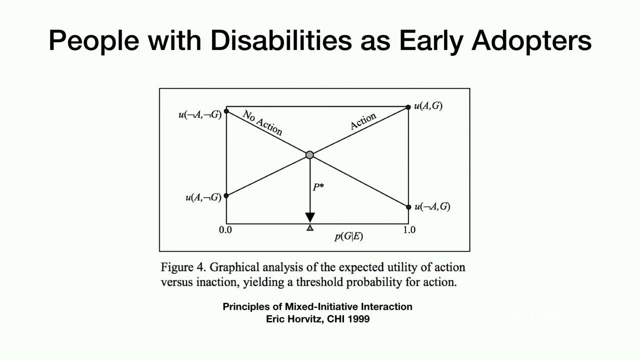 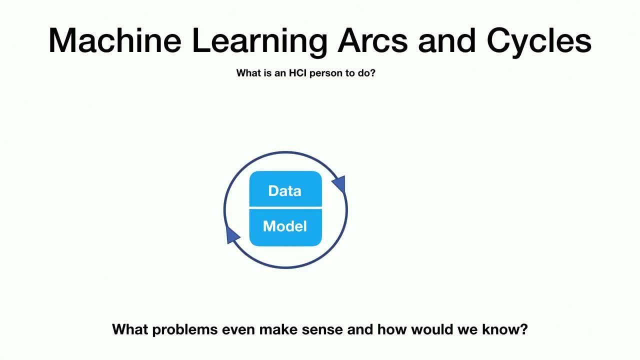 real are often people with disabilities. So the people I know who have relied on speech recognition for the longest are, say, people who can't otherwise type. I think that one of the things that accessibility has really taught me, and I think it's a broader 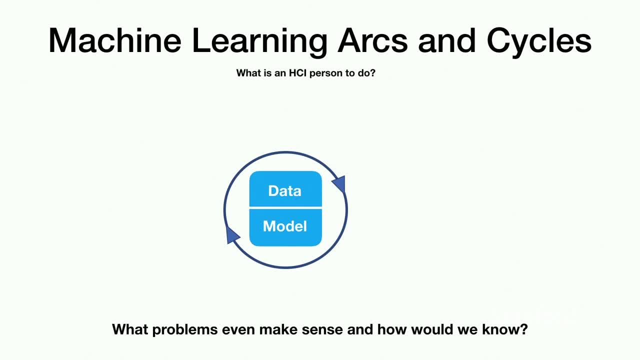 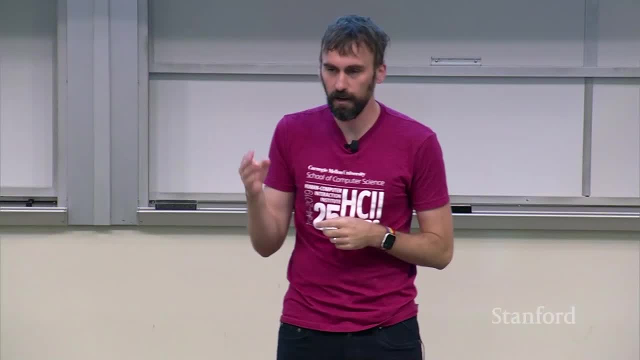 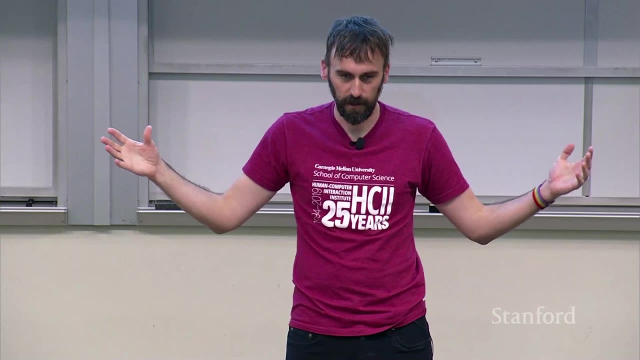 broader point for HCI is that for lots of reasons, AI, ML- people tend often to be focused on kind of iterating with a fixed set of data and then trying to improve models, see where they get out of things. I think there's a huge space that goes beyond that. 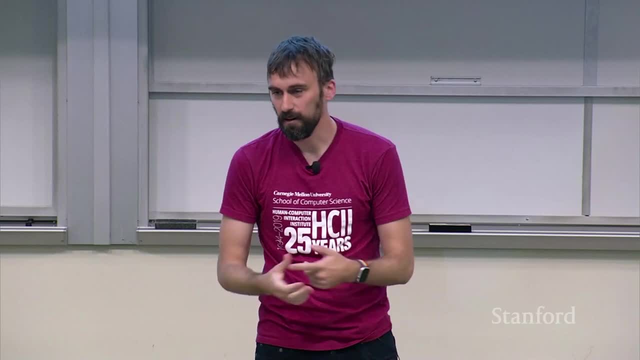 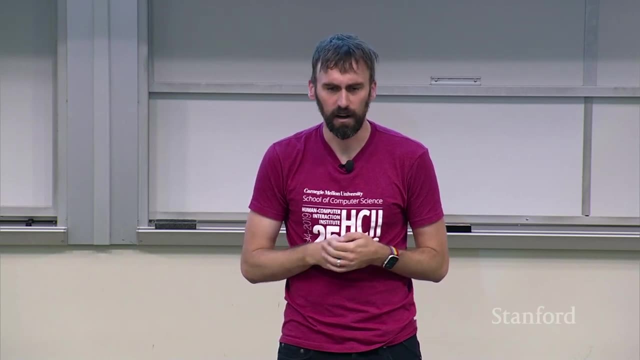 And a lot of that is not fixing on a particular problem, not fixing on a particular data set, evaluating alternatives, figuring out interaction flows Where, yeah, this might work for some subset of people, but what's the fallback if it doesn't? 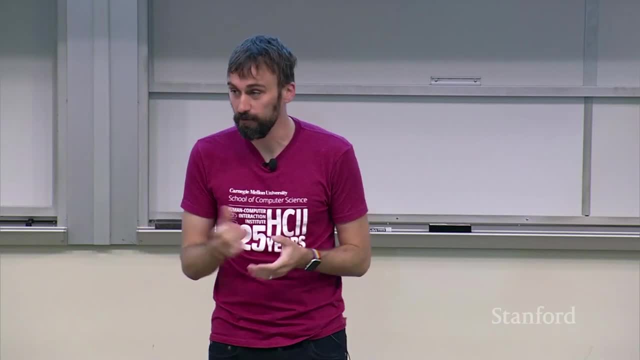 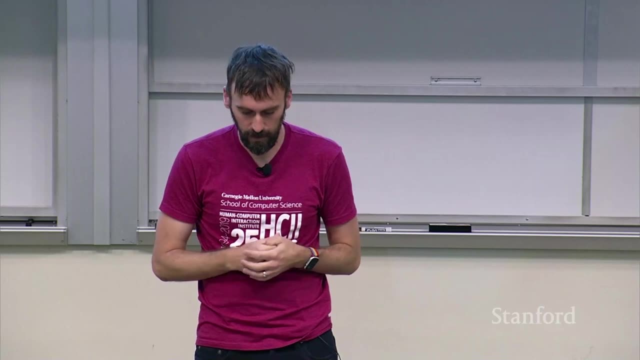 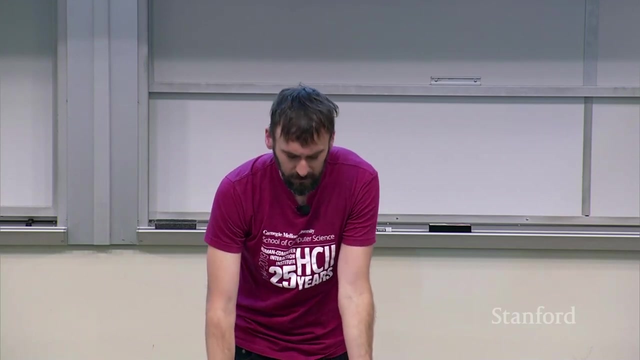 And considering all those things kind of at the same time And then ultimately figuring out if what you produce is even something that is worth having right. Maybe the limitations are so great that it's not. And so I think I somewhat facetiously, but ML HCI right. 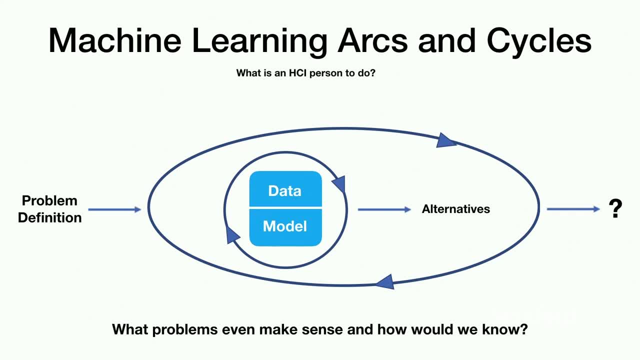 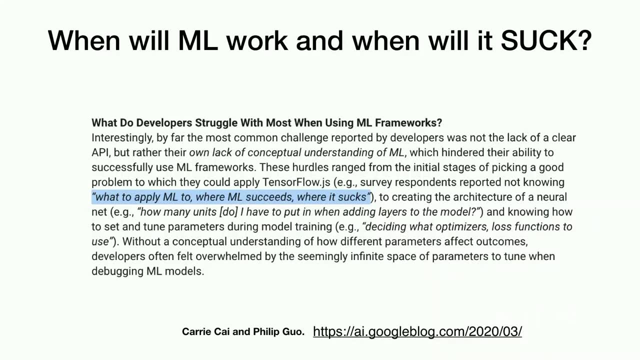 I feel like this huge part of what it means to really develop and deploy real ML systems Is really HCI problems. You know there's some recent work by Kerry Kai and Philip Guo Talked to people about what do you struggle the most with when using ML frameworks. 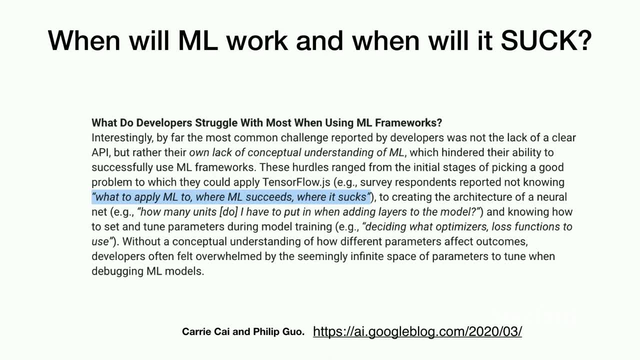 There's a lot of stuff that is, like you know, parameter tuning and all this stuff. But one big thing is: you know, when should I apply ML to what? When will it succeed and when will it suck right? I think that's an underappreciated, but 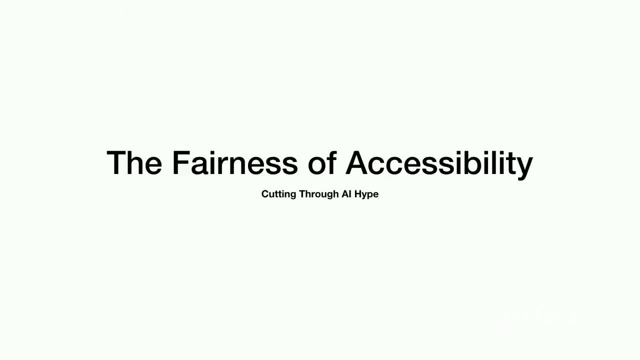 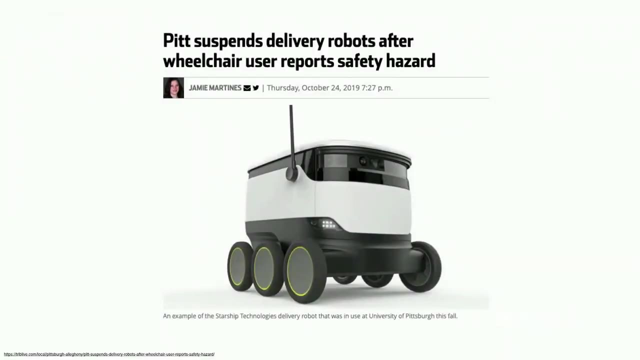 huge part of developing real ML systems. Accessibilities really taught me about well. what does it mean to develop fair ML? Lots of ways to think about this. I like to have concrete examples. Example: in Pittsburgh we had those little driving robots that were delivering food. 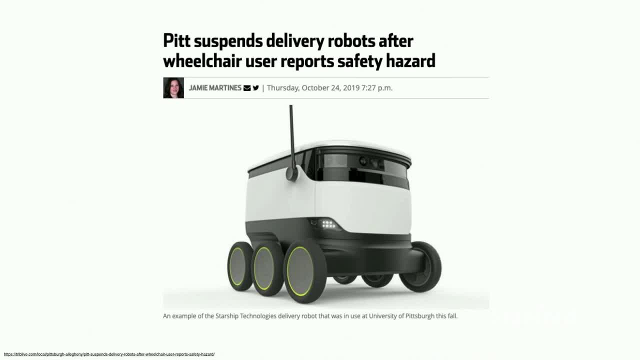 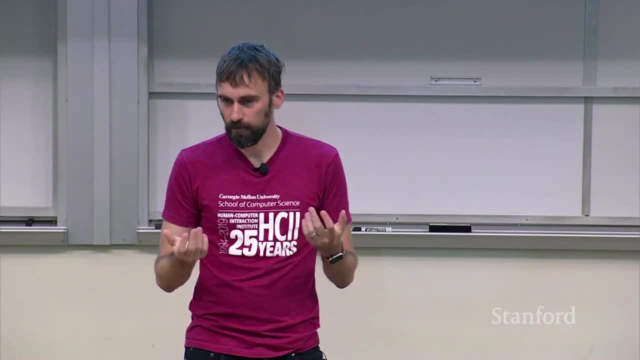 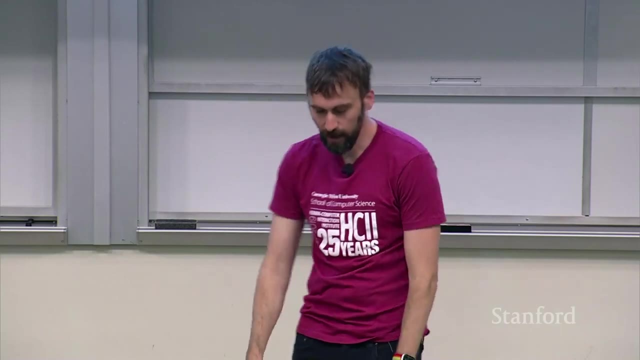 In Pittsburgh and they had to be pulled off the road Because they failed to do something that you know an intelligent human could do: They could drive to wherever they were going. That was not actually the hard part. The hard part was if they got to an intersection, you know. 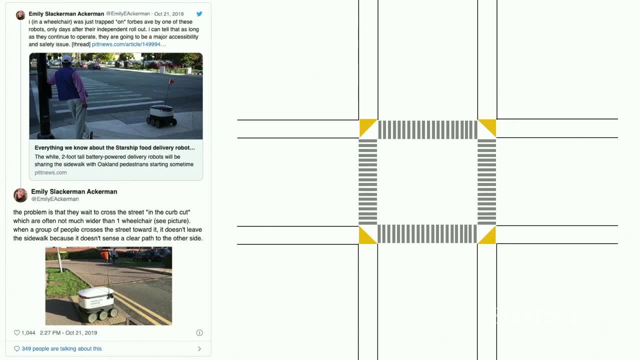 they just sat in the little curb cut here And so other people need to use the curb cut right And they didn't realize. That's just one of the many, many different, like little problems you could run into in the real world that accessibility sort of you know brings to the fore. 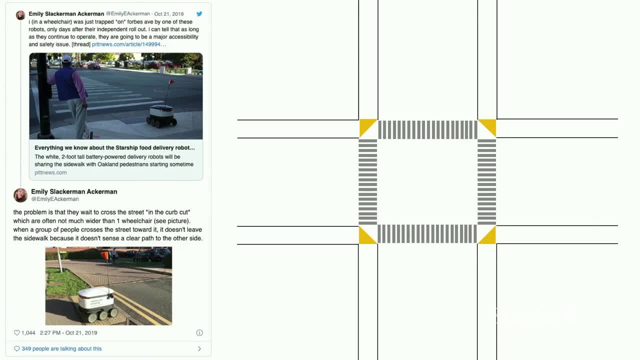 So there was a wheelchair user who was trying to go across the road the other way And they couldn't get up the ramp because, you know, the robot was there. The robot didn't. it doesn't move out of the way. It might stop if it's concerned it's gonna hit something. 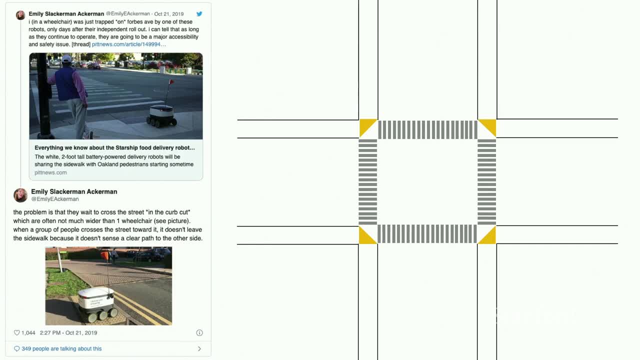 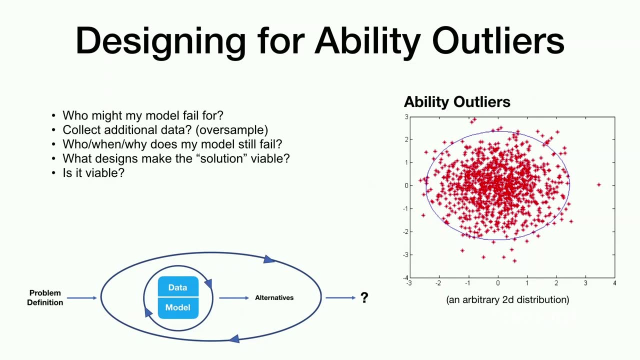 It's gonna hit somebody, but it doesn't move out of the way. And so this left me thinking like I think one of the big challenges in developing systems for real is: you know, how do we design for ability outliers right? 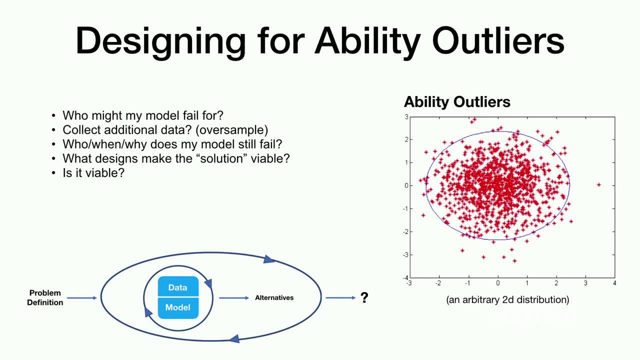 So this is just a random distribution, but there's a lot of people out here, right? If you imagine this somehow is people and it's hard. It's hard in an ML world to do that, right, Because you don't have enough data, right? 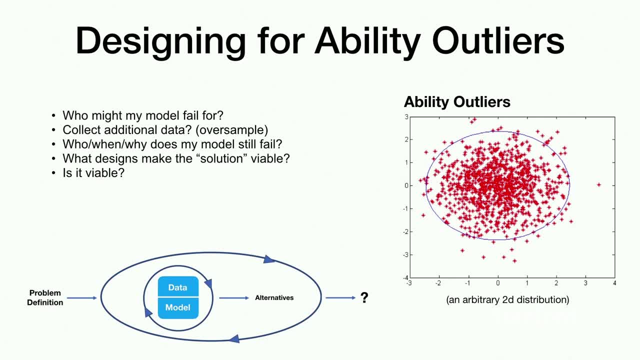 So how do you do that? Well, maybe we could collect additional data, We could oversample And trying to predict in advance. you know, the unknowns is obviously really hard. The unknown, unknowns. And so what do we decide then makes a solution viable, right. 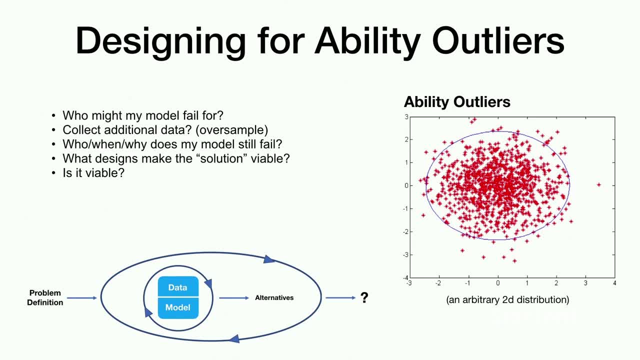 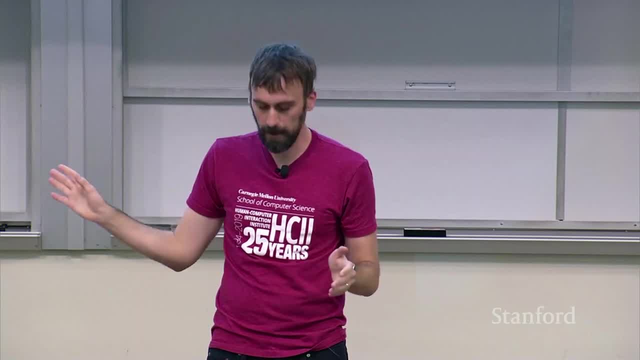 So how many people does it need to work on? How do we avoid those mistakes of the past where you know we've locked into a certain set of abilities that matter and a certain set that we'll deal with later? Yeah, so, anyway. so some concrete ideas here. 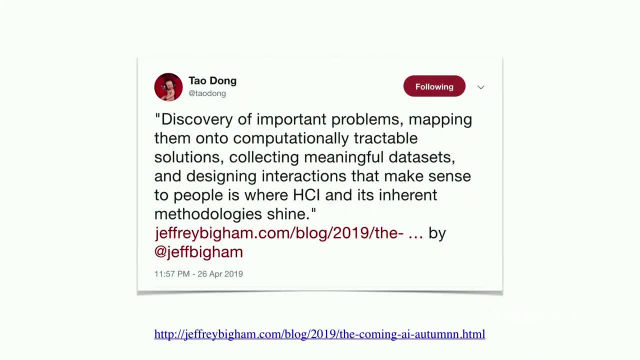 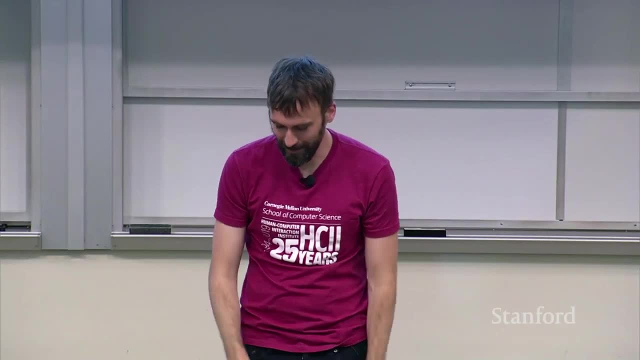 You know, I think that discovering these important problems and mapping them onto something that's computationally tractable, collecting meaningful data sets, designing interactions that make sense, all this sort of is in the purview of HCI right. At least I think so. 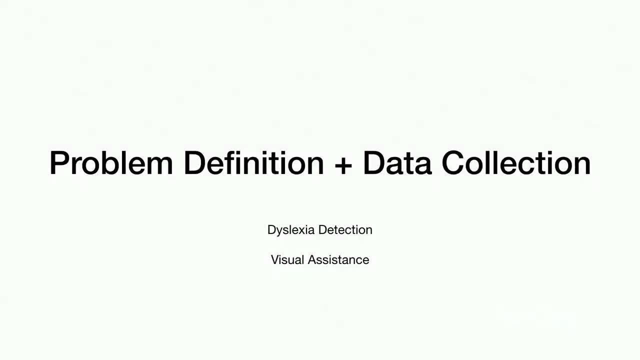 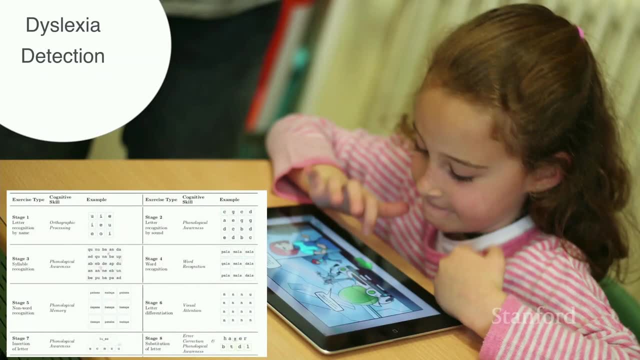 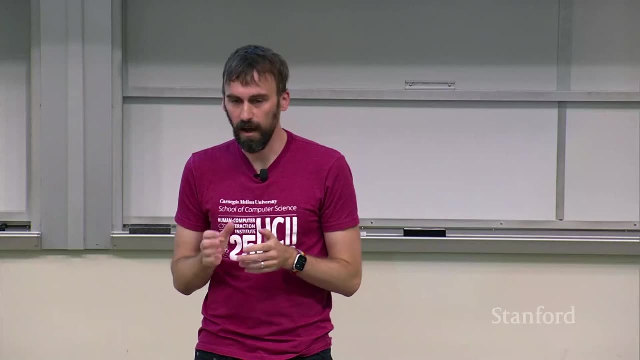 So here's some examples of problem definition and data collection. So this will be in dyslexia detection and visual assistance. So a project I worked on with a postdoc, Luthrello, was dyslexia detection. Problem here is that there is a huge amount of kids, especially in schools, that have 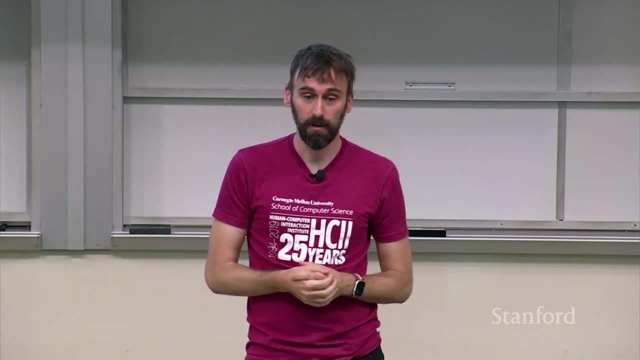 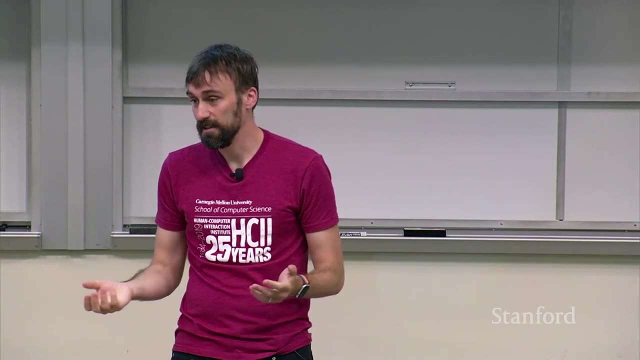 dyslexia, who don't know they have dyslexia And, as a result, the most common way they find out is they start failing in school. That goes on for a while And then eventually someone maybe says: hey, I wonder if you have dyslexia. 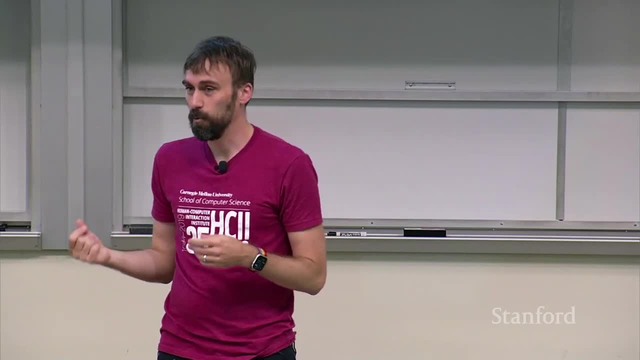 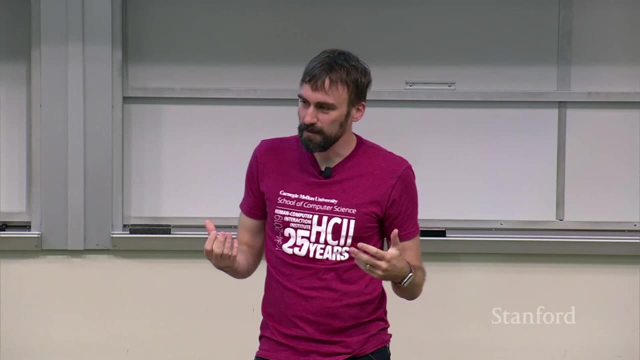 And then they go off, maybe to get a $2,000 test, And so we wanted to kind of reduce that burden. Why? I think this is not. Yeah, This is a really hard problem, but at the same time, most of what was hard about. 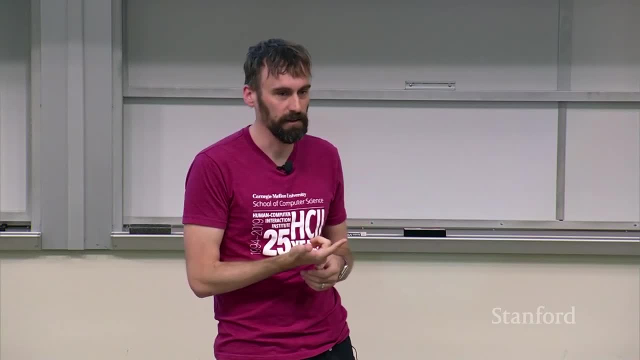 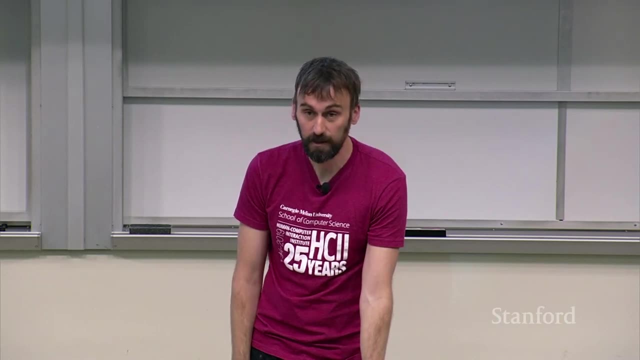 it was figuring out what data to collect and then actually collecting the data, And so we- Luth mostly, who has a linguistics PhD and knows a lot about dyslexia- designed some exercises based on a bunch of prior work to elicit differences that she thought would. 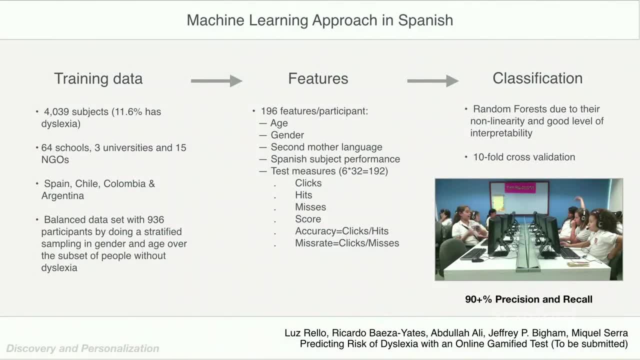 elicit differences and then collected a huge amount of data from about, yeah, a few thousand people, Many of whom had dyslexia, based on diagnosed tests, which is really hard to find right, Because the whole problem is that you don't know for sure, and so you have to do all this. 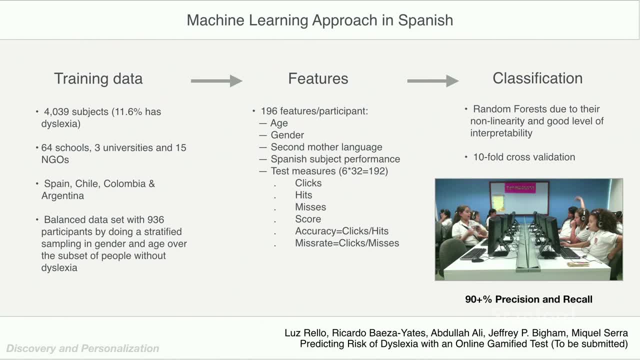 careful screening to make sure you don't have people that actually have dyslexia, who don't think they do. Anyway, lots of different things there And built a classifier that used pretty simple machine learning to get a reasonably good precision recall for a test. 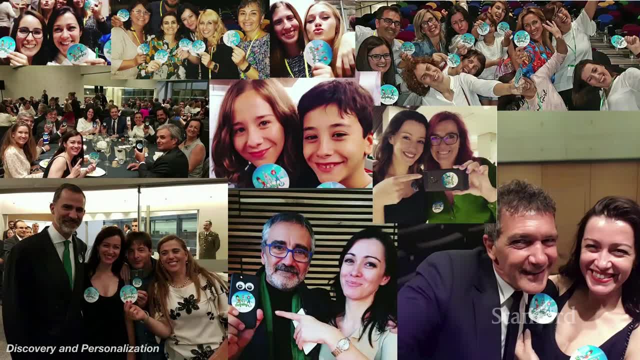 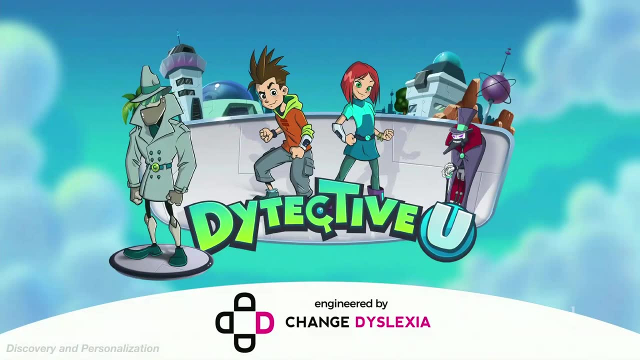 And that test is now out in Spain. It's been used by A couple hundred thousand people. There's Luth with all of some very famous people. You have to do a quiz about whether you can know who all those people are, And developing it into a training program as well, so that we can not just kind of detect. 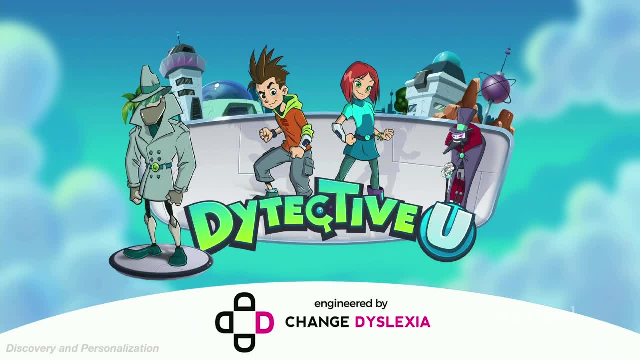 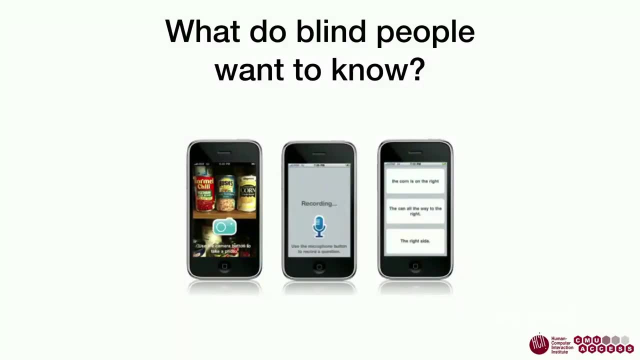 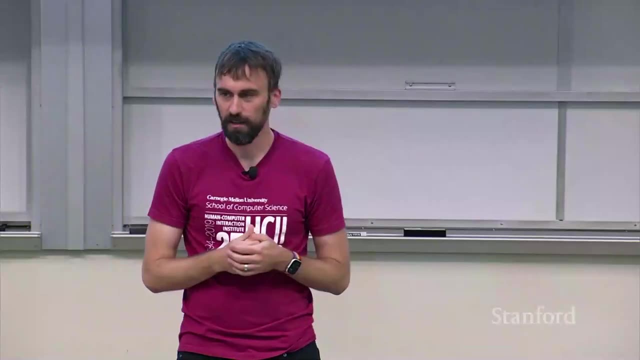 but also kind of use the detected strengths and weaknesses to then customize a learning program. Another dataset collection, which I didn't even think of as a dataset collection at the time, A project where we We released this iPhone app that crowdsourced visual question answers. 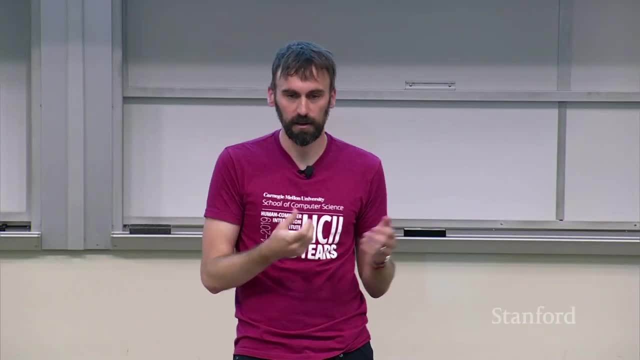 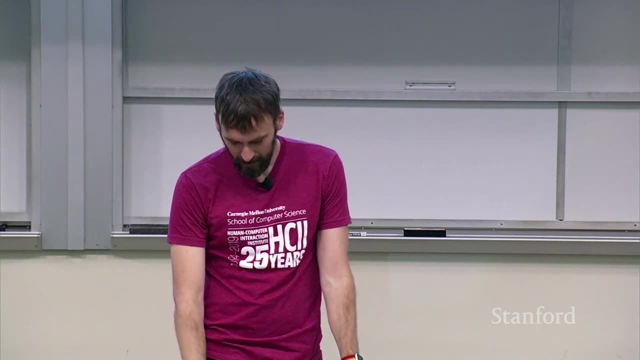 So a blind person could take a picture of something they wanted to know about, speak an answer or speak a question and then get an answer back from the crowd pretty quickly- And I'm just going to run through this. We got so many. 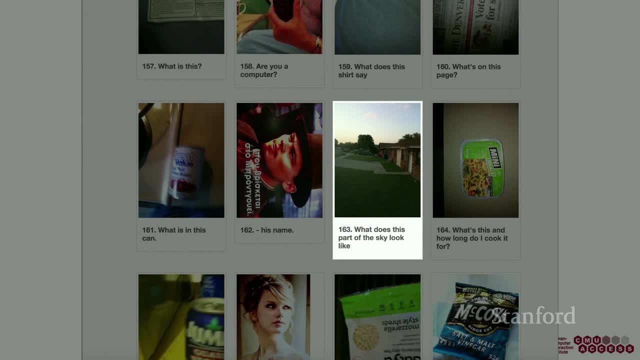 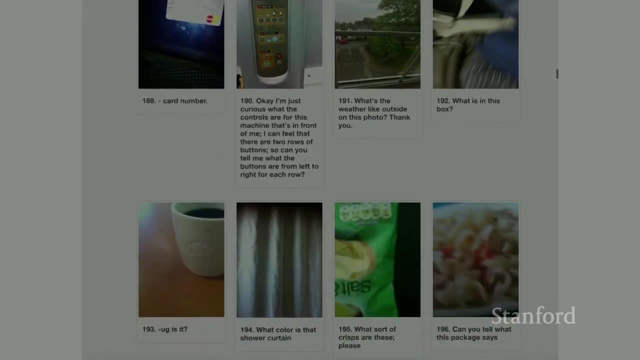 We released this. We got- I don't know, I think it was. It ended up- 180,000 questions or something And it's all over the map. You won't. You can ask me later if you want to see more examples. 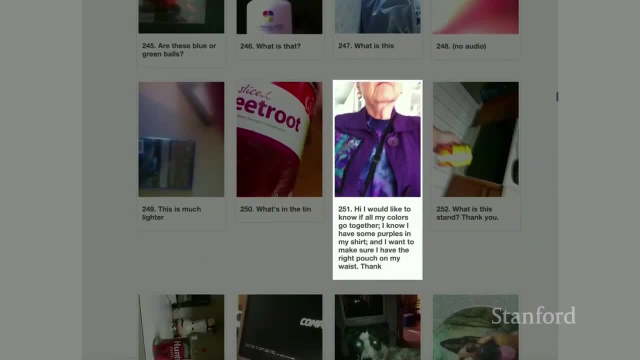 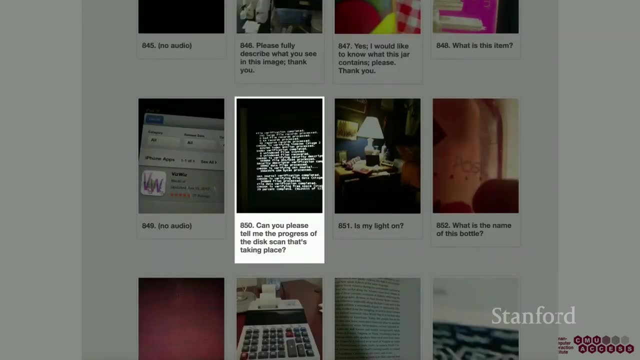 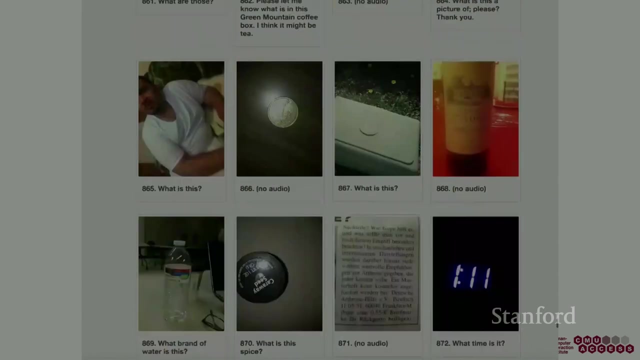 We got interfaces that don't work. We got fashion advice. We got broken computers. It's like, what does this thing say? My computer's broken and now the screen reader doesn't work Right. So lots of stuff. We got a pregnancy test. 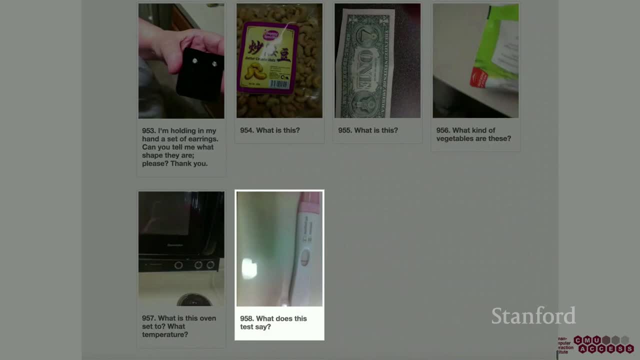 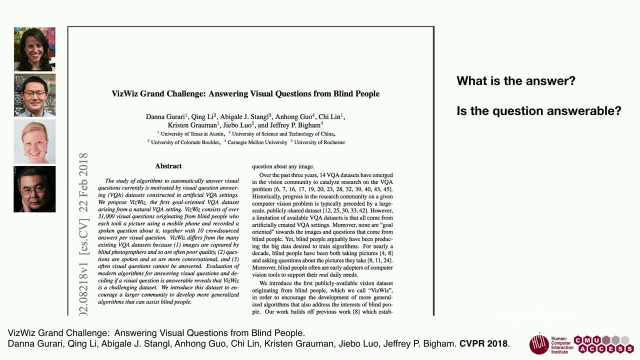 So apparently there's not accessible pregnancy tests out there, And so after a while- and it took some work again here dealing with some of the privacy concerns- we were able to release this as a data set. We had a CVPR paper and now we have a series of workshops at CVPR where we're challenging. 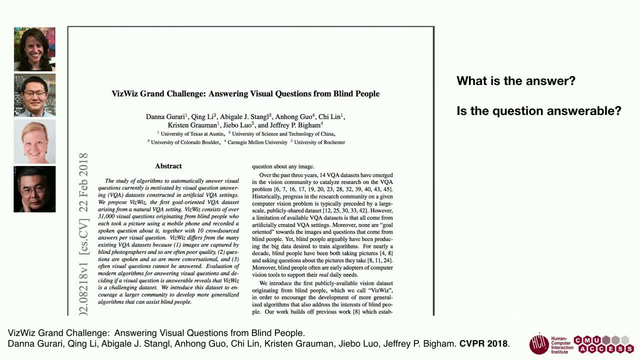 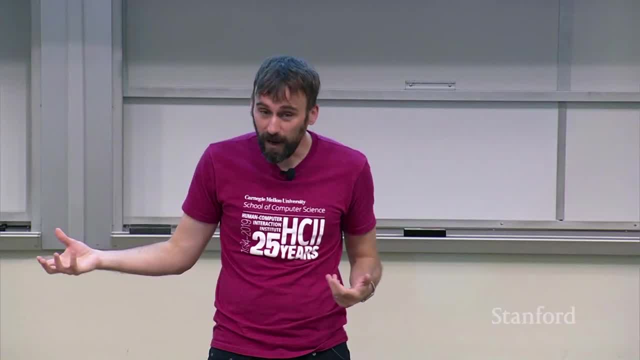 people. So there's already this really active community in visual question answering in the computer vision space. but now we have a real task for them And it turns out the pictures are different, Like half the time. the thing they're asking about is an in-the-frame, you know the blurry. 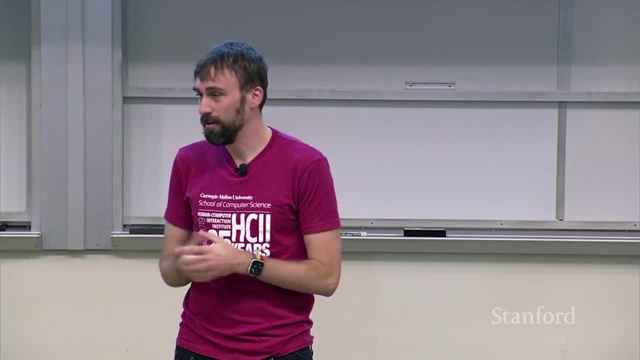 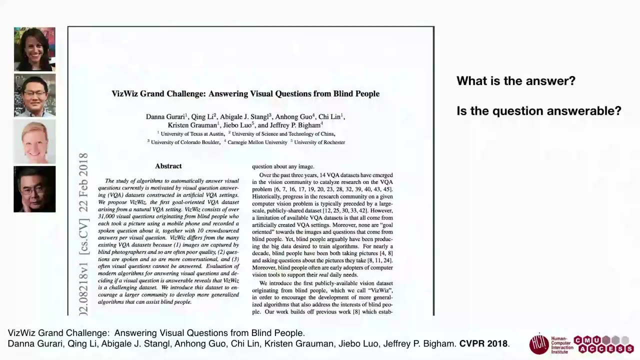 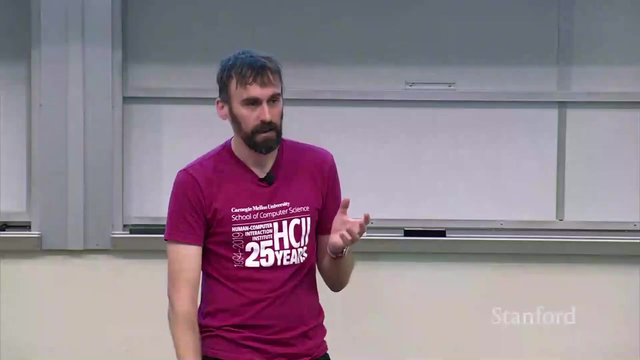 It's really, really challenging And, to the community's credit, there's actually been a lot of interest in this, which has been exciting. We also realized that one of you know, in basically preparing this data set, one of the challenges is for making something like this work is helping people better understand. 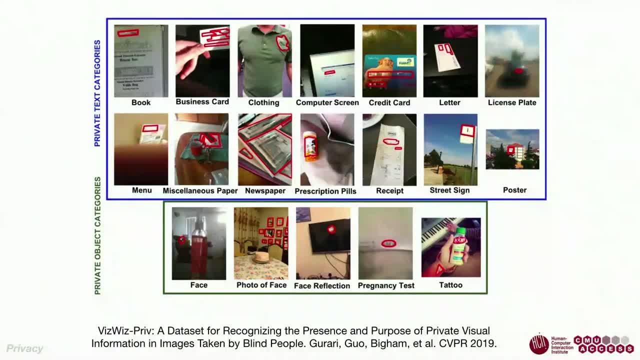 whether they're revealing private information. And so we were able, again with a lot of work, to be able to go through and create a data set of images with private information stripped out, so that then you could set up, we could set up a second challenge of: can you predict whether this image has private? 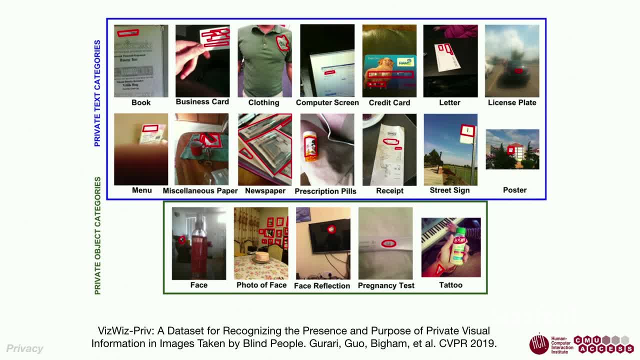 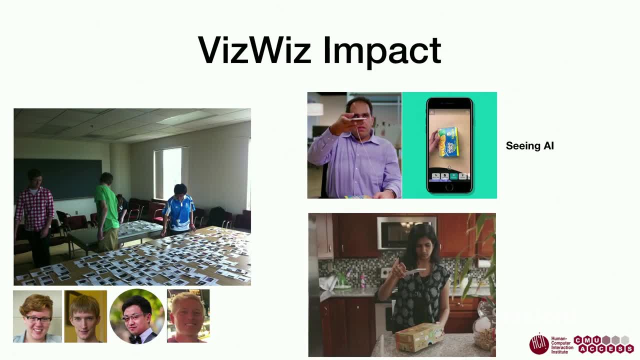 information in it, or not? Kind of interesting, This ended up getting into a couple of products, So Microsoft Seeing AI, Google Lookout used our data set in part to train their models. One of the things, though, that it revealed to me is: I think that there's a. I think that 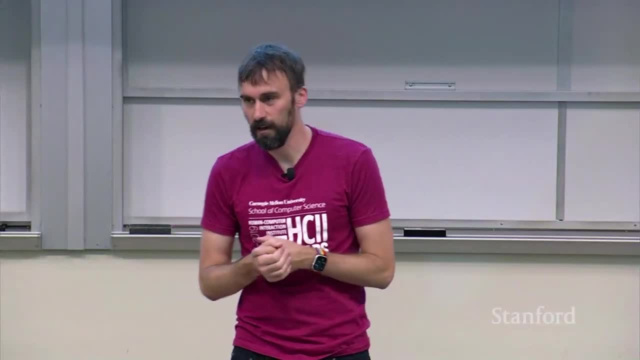 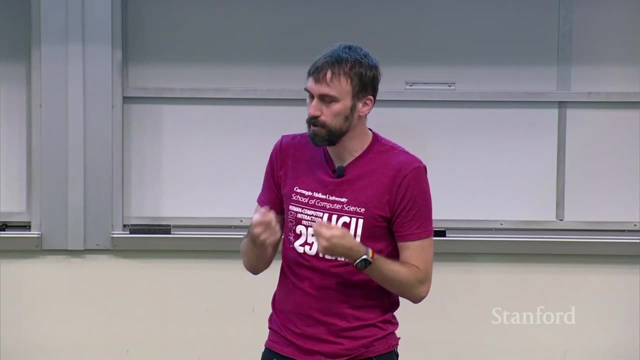 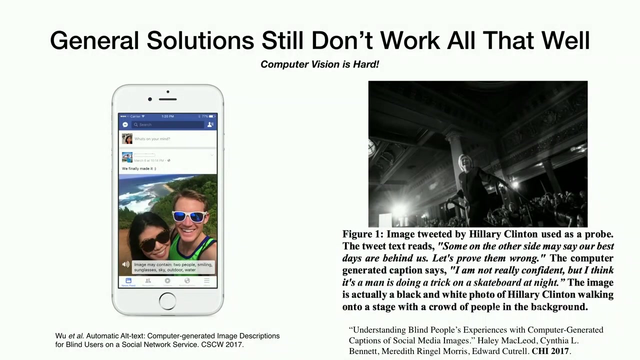 in our rush to do all of these fancy things with AI, sometimes we fail to find the kind of limited scope But practically really important problems that we could really make work. And so you know general solutions for visual question answering or image captioning still. 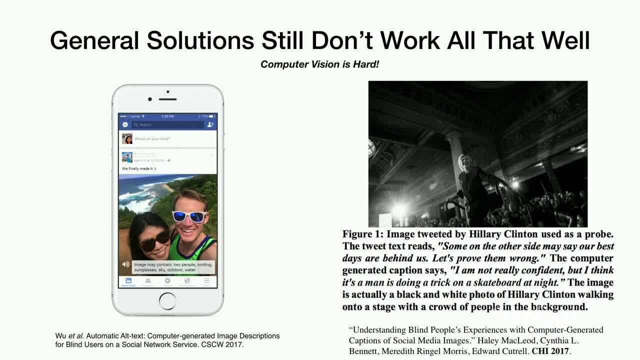 don't work all that well, right? So, like Facebook releases, which is pretty cool, they released it. you know, every image now that gets put on Facebook has some tags associated with it, so you can kind of understand maybe a little bit about what's going on. 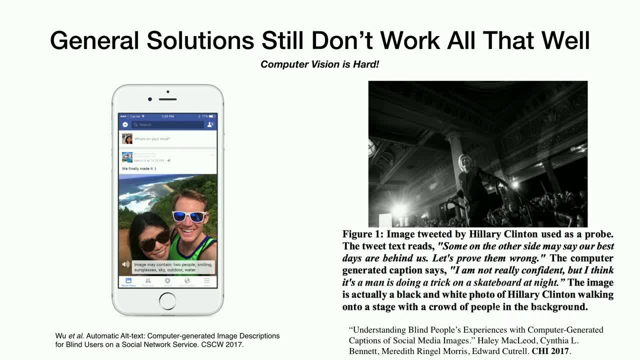 You know two people smiling, sunglasses, sky, outdoor water. obviously you're missing some stuff. You're missing some context, But it's interesting when they make mistakes. So Mary Morris at Microsoft has this great example of you know, it's Hillary Clinton. 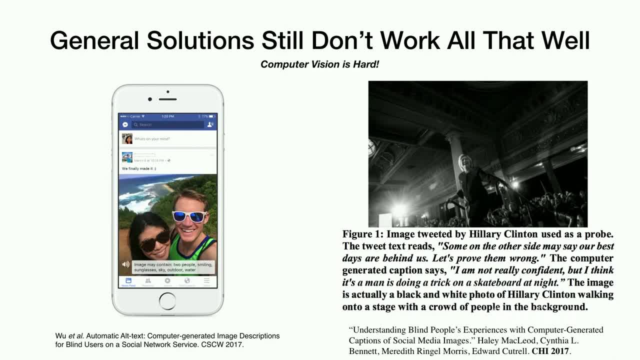 getting onto the stage and it says: you know, I am not really confident, but I think it's a man doing a trick on a skateboard at night. And then they interviewed some people who are blind and they said: well, why do you think Hillary Clinton would put that on her web page or Twitter feed or whatever it was? 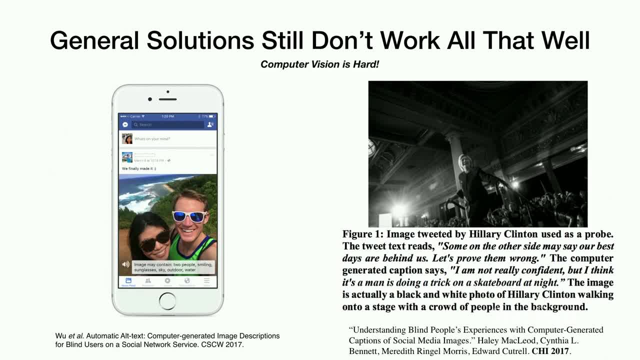 And they said: well, you know, she's probably trying to appear young and hip and whatever, So it can be very confusing, right, Whereas some other problems, I think we can actually pick them out so that they can work very reliably. 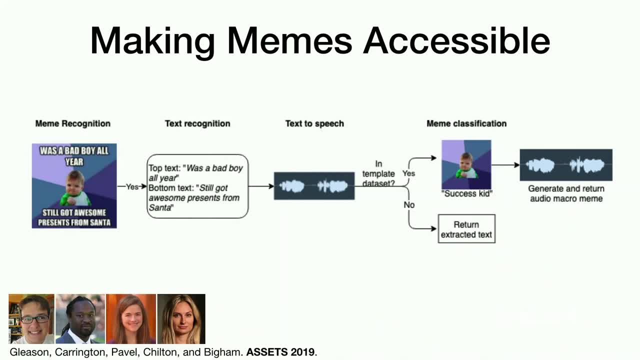 So one thing we've been looking at- which even I was surprised by how much attention there was about this- but making memes accessible, and this is kind of the old school memes We're starting there, you know, moving forward. What's really nice about this is it's a very narrow problem. 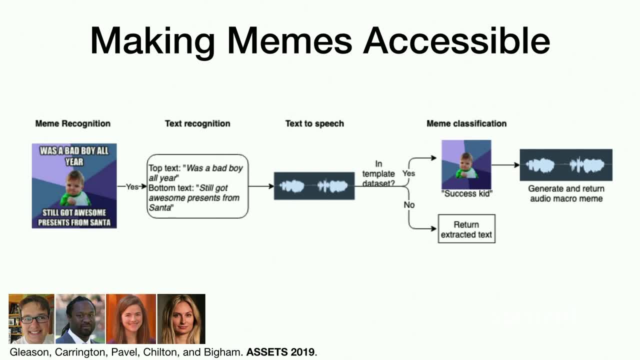 There's only so many meme templates. The text is always impact, bold, right, So you can make this work. You can make this work very, very reliably right, And so one thing is to just, you know, make it accessible in the sense we describe the. 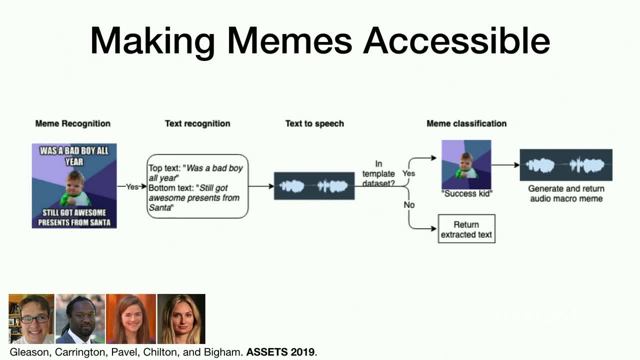 meme template and we say what text it is. We've also been working with you know more of a design process with participants about well, what would be a more first-class version of meme accessibility. So I think I have an audio clip. 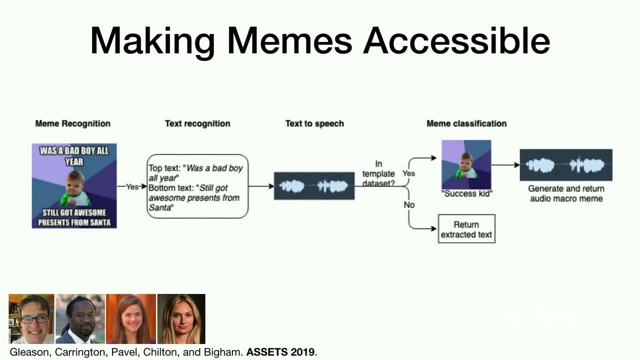 If I don't, I'll be really sad. Put candy bar in shopping cart without mom noticing. Yay, Yay, Yay. So that's sort of like Success. Kid made audio with a little you know some audio sound effects. 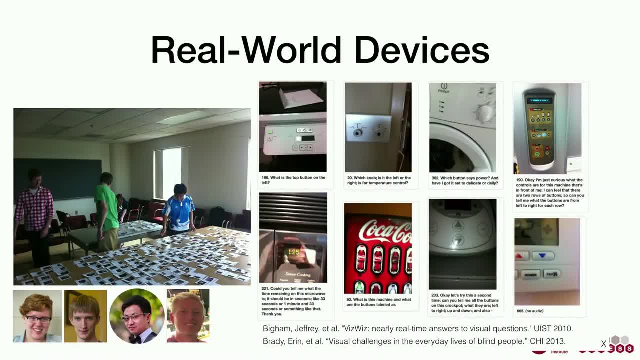 Other thing: even from the VizWiz dataset like it seems very large and it was very large in scope, but we noticed some patterns. right, There's all these real-world devices, So there's like all these appliances, but none of them have accessible interfaces like 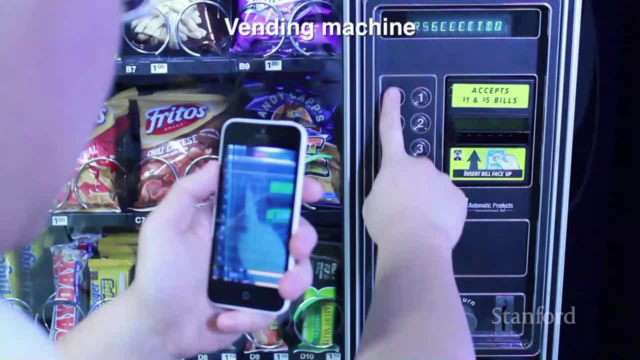 I, you know, mentioned this, but So we made a system that you know uses some crowdsourcing, plus then computer vision to give feedback, And we're able to, you know, make vending machines, Yeah, And make vending machines and things accessible. 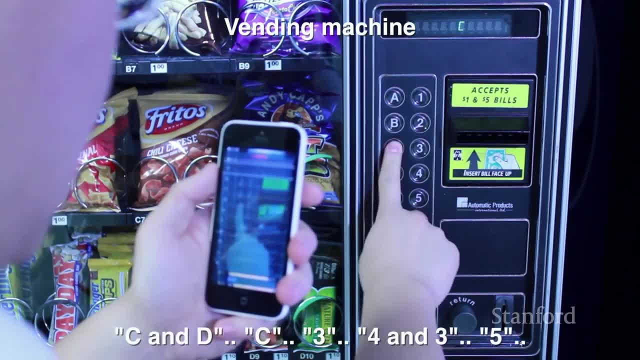 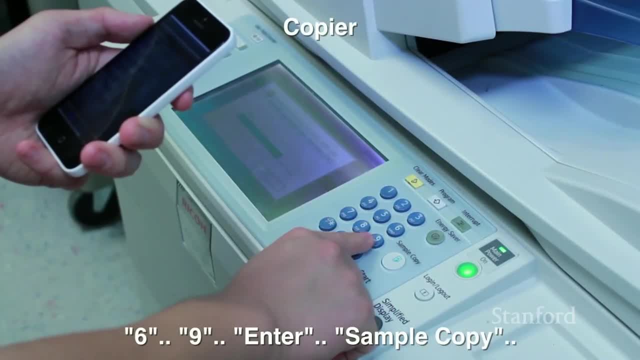 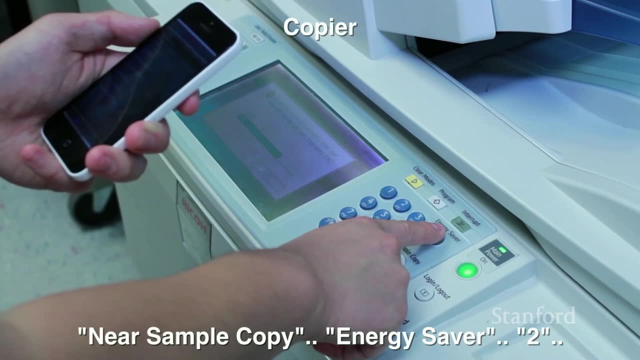 You can imagine replacing some of this with OCR Energy saver. Energy saver Two, Yes, Yes, Down, Down, Down, Down and yes, Down, Near seven, Near back, Seven, Eight and seven, Seven, Eight, Seven. 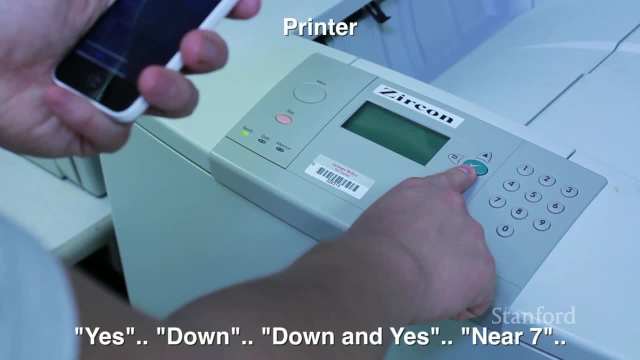 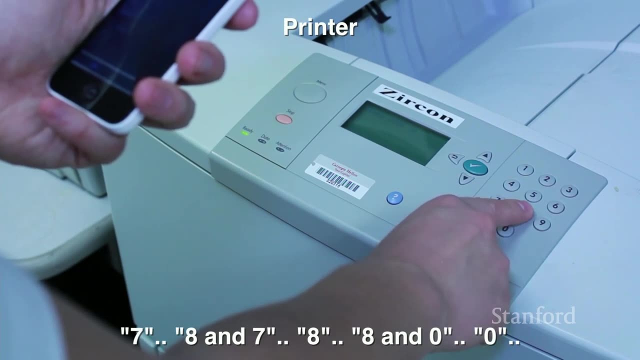 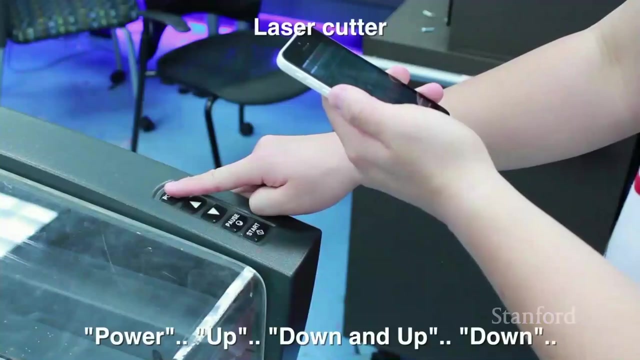 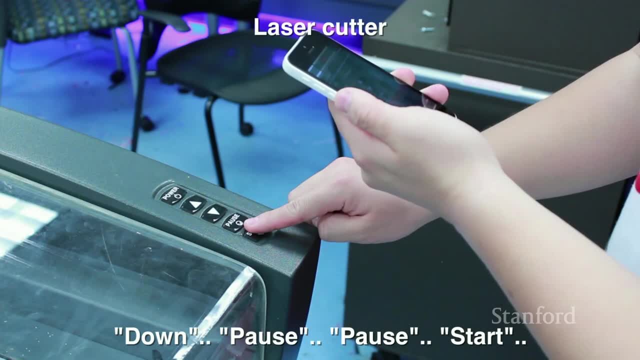 Down, Down, Down Down. I always like to end on the laser cutter Because I'm like blind person using a laser cutter. I'm like, hell yeah, blind person using a laser cutter. With a little bit of extra work and some, we actually put a dollar bill next to the interface. 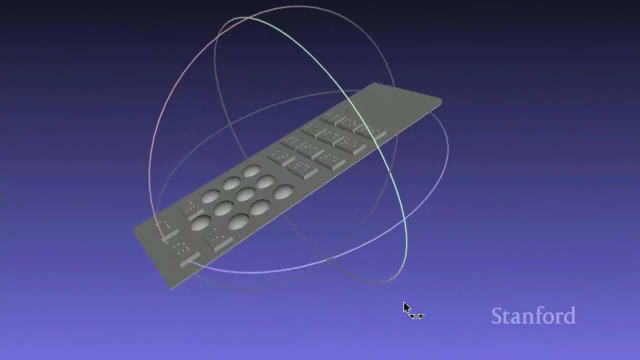 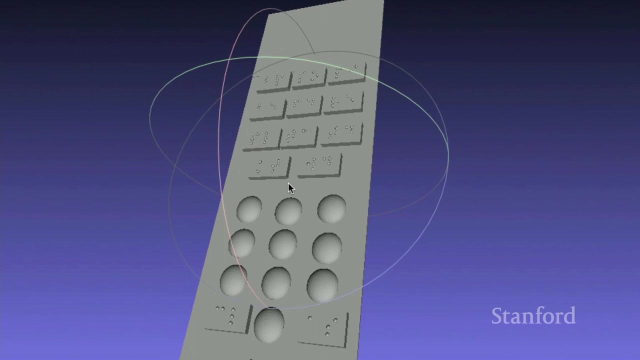 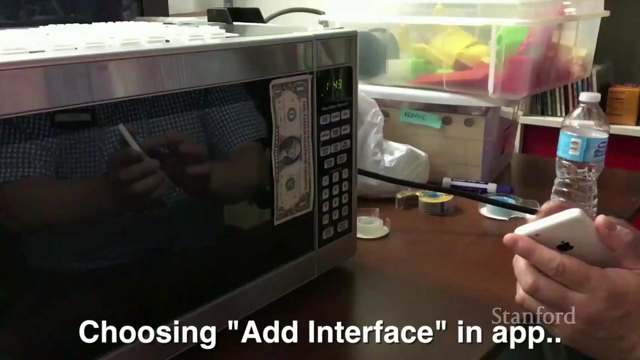 to get a real size. we're able to compute a 3D model of this and so- again kind of the spirit of translating it to new modalities- we're able to go into a fabricated tactile version of the interface. We send this off to 3D hubs, we get printed, and then here's a blind participant going. 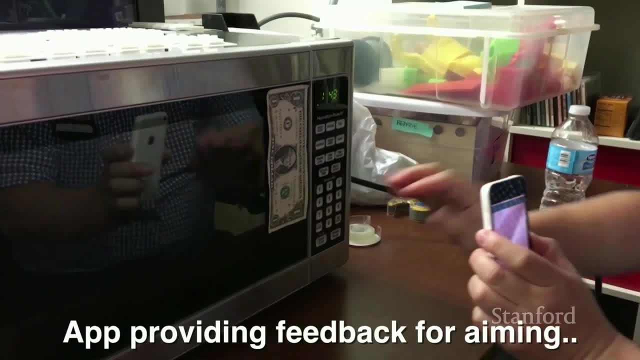 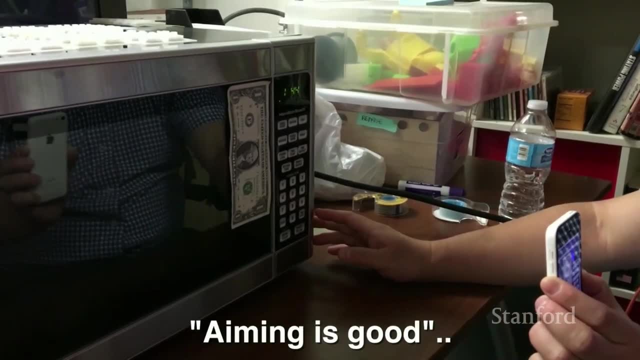 through the process of actually using this, So you take a picture of the dollars there so we get the right size stuff. They get a little bit of feedback about that's a whole other problem. How can we assist people who are blind with photography? 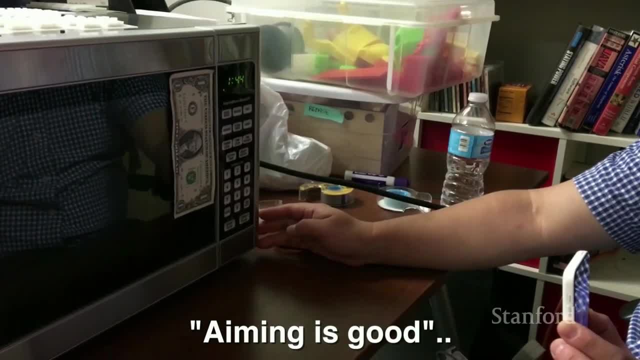 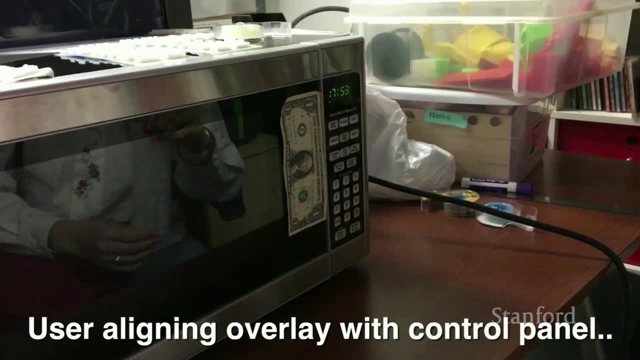 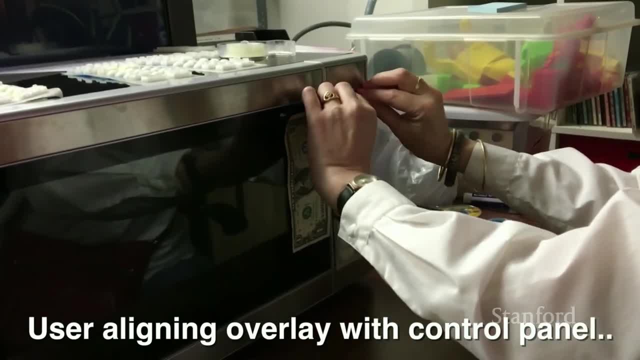 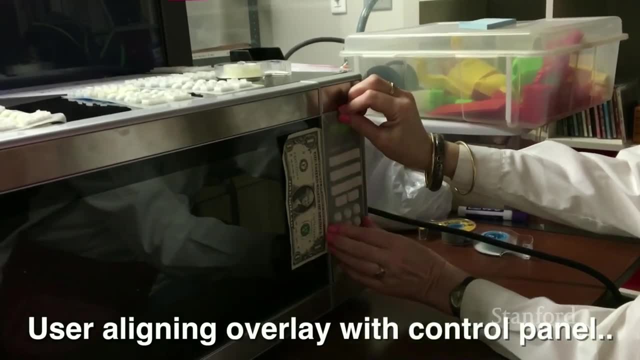 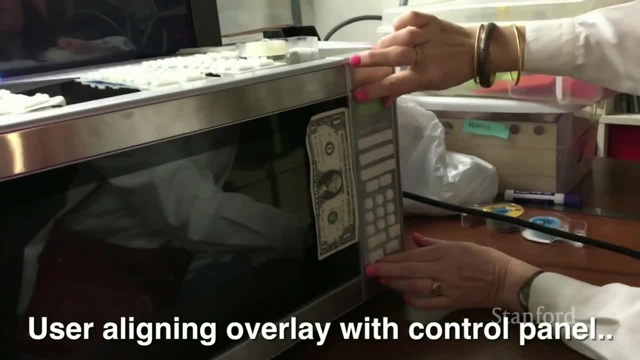 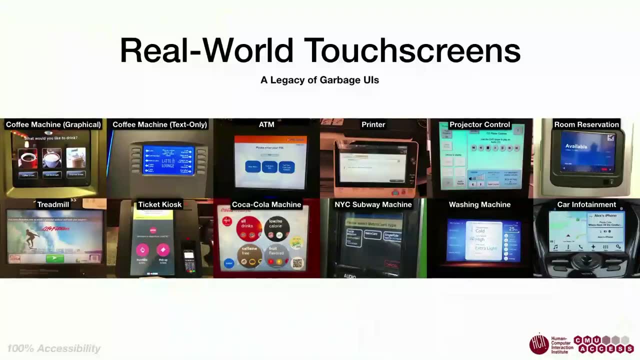 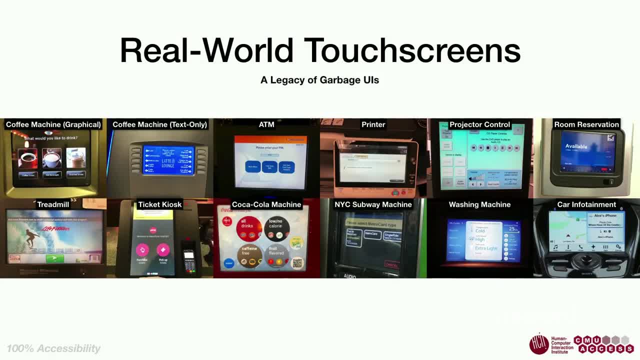 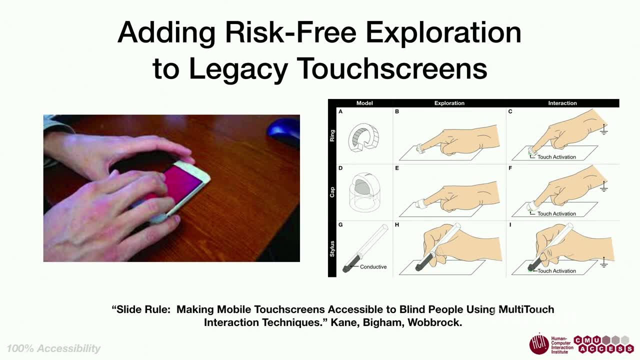 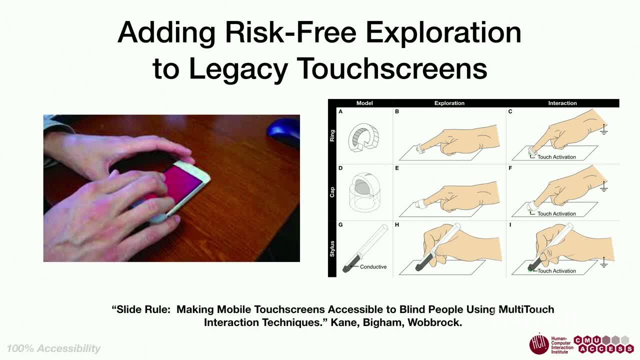 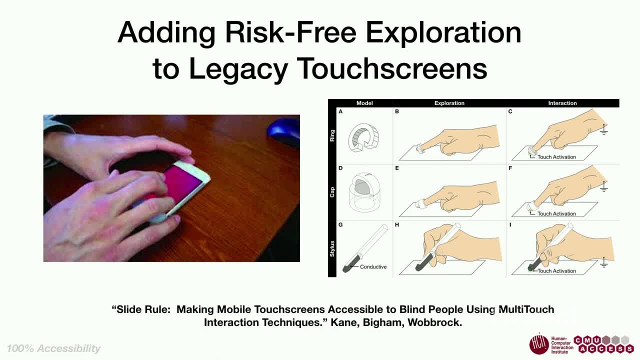 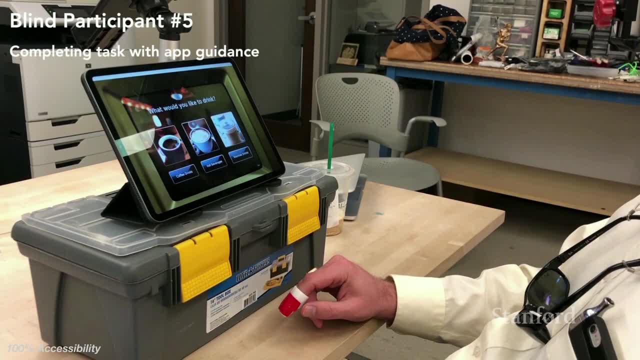 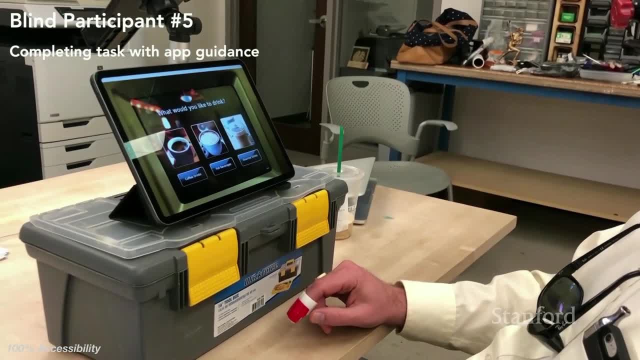 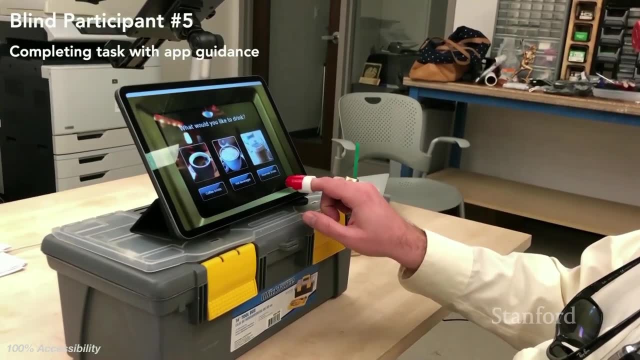 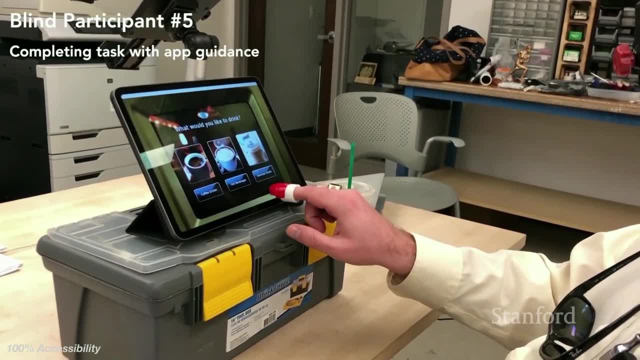 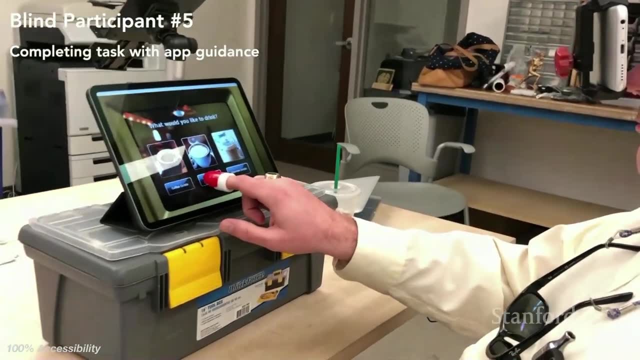 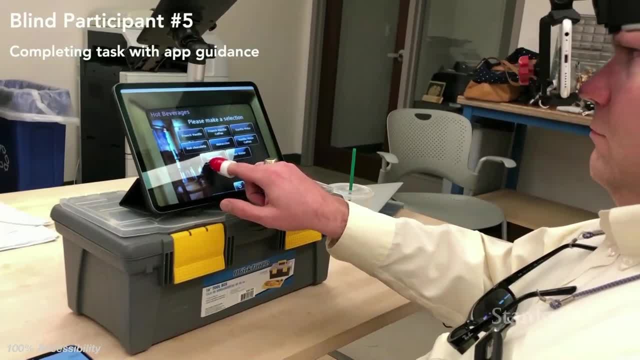 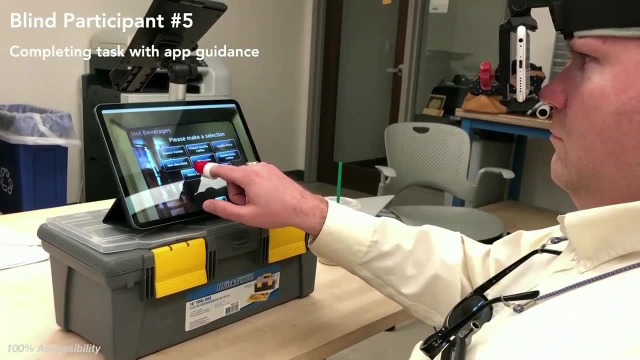 Aiming is good, Aiming is good, Aiming is good. There's also this dialogue system that's working behind the scenes, that was built up automatically from videos. Anyway, lots of stuff happening to kind of get over this legacy problem, whereas if you 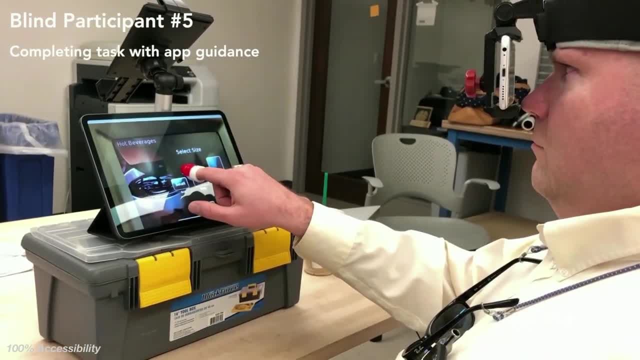 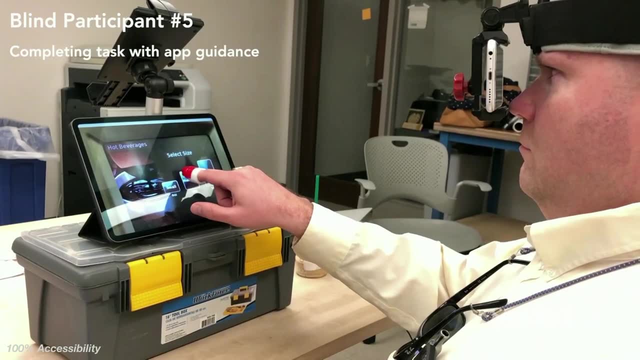 imagine the coffee machine. if the coffee machine was accessible from the beginning or used a platform that was accessible, if it was Android-based or iPad-based, it would just be accessible. But because they're not, then there's all this work. It's an interesting tension. 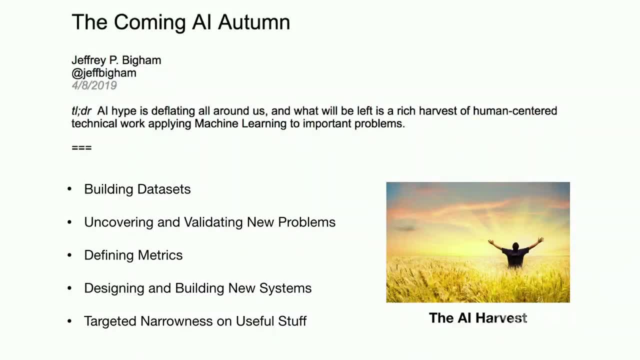 Okay, so I'm out of time. So I really think there is this huge potential. though- and I don't think it's the hypey AI that sometimes gets the most press- I think that the hard work of using the tools we have for machine learning and applying 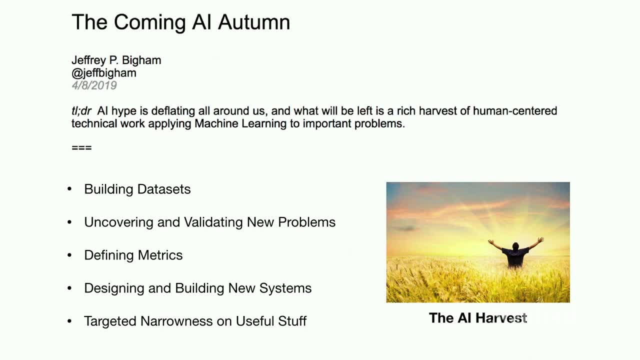 them: discovering real problems, applying them to real problems. I think there's just this huge harvest, right so the AI autumn harvest of things that we can do And hopefully we can actually get over some of these hugely hard, long-standing problems. 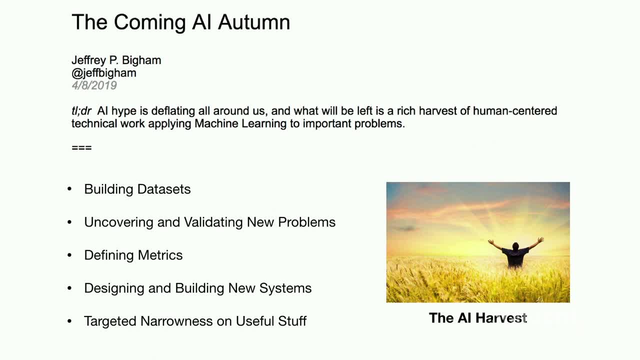 in accessibility and otherwise right. So without machine learning we're not going to, I think, get past the scale problems, the legacy problems, some of these fidelity problems of translating between different modalities. But I think there's a huge opportunity to make progress and so I'm really excited about. 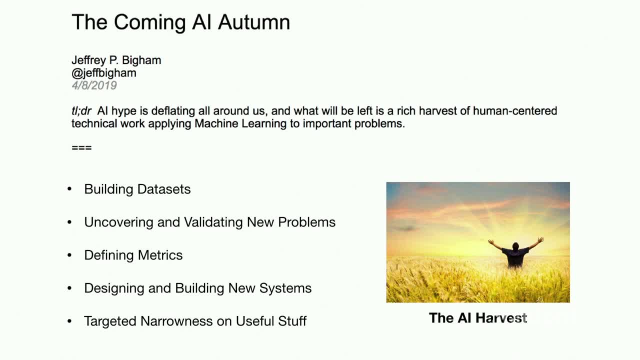 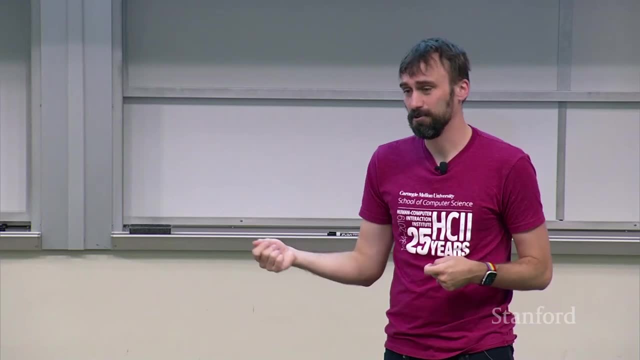 that, And so I have some ways that maybe HCI people in particular might contribute to this through building data sets, right? So building data sets is hard, especially interesting, new, novel ones. Sometimes it means having a whole bunch of things. You have a whole project designed just to get out in the hands of people so that then 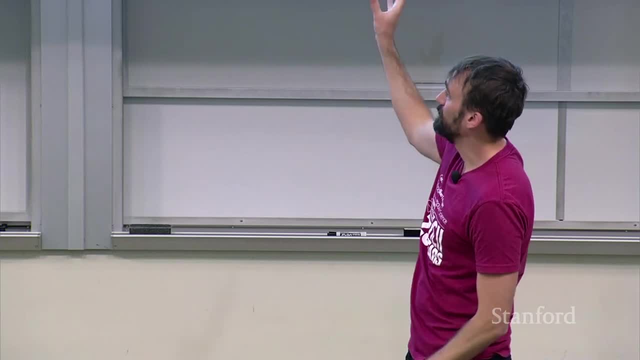 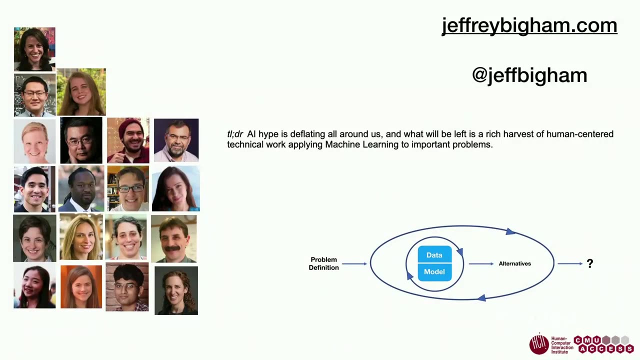 you can get data back from it And lots of other things- uncovering problems and all this stuff. So I'm going to end here. Thank you very much. Here's obviously a huge number of people collaborating on this and I'll take your 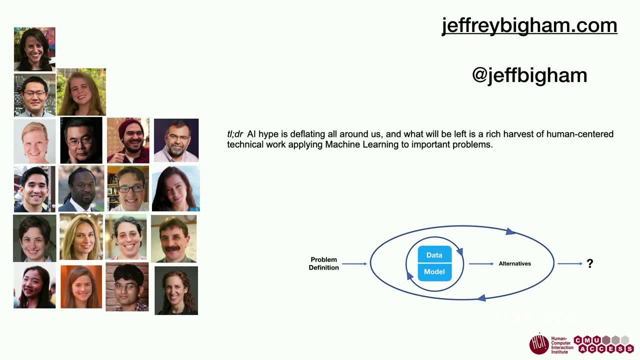 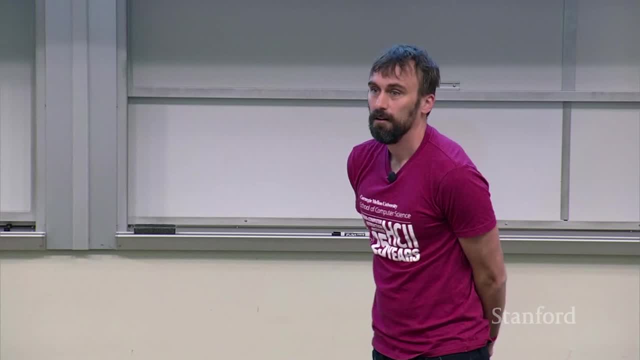 questions. Thanks, Yeah, Why do you think the large companies that make the products that you're talking about, the companies that you're working with, the companies that you're collaborating with, are making the products that you showed, from the iPhone to microwaves- are not devoting the 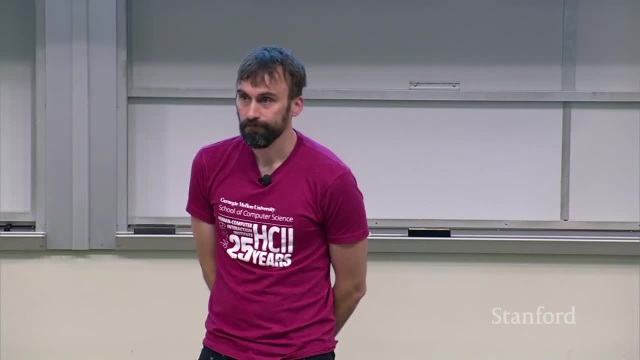 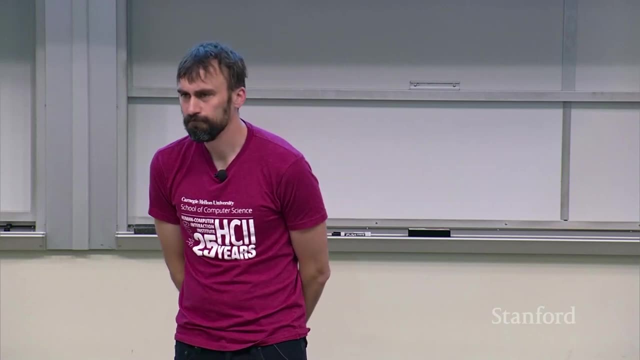 resources to develop it from the beginning, as you suggest? And is it a market? there's not the market there, or that they don't realize what the market is? And are there any companies that you think do a particularly good job or bad job of doing? 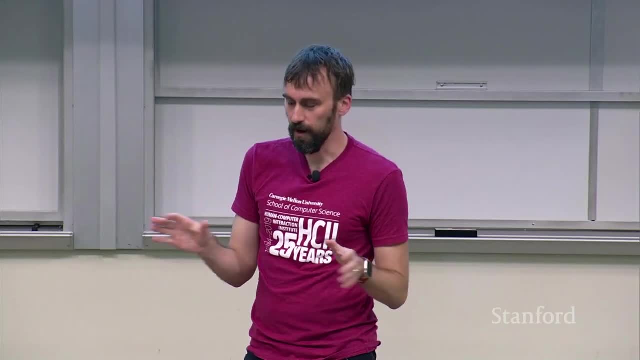 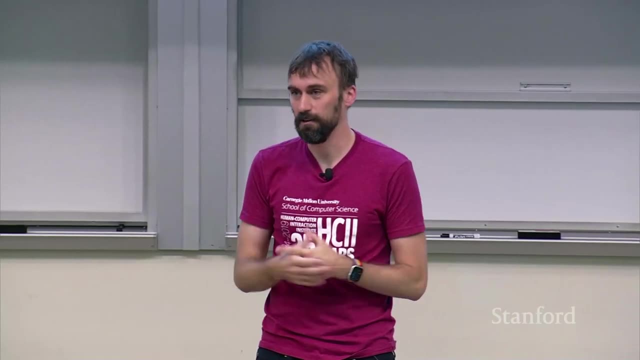 it? Yeah Well, I think it's a really great question. There's a lot of things going on there. You know I have a lot of respect for Apple. Apple has done a lot, So the iPhones are accessible to the degree that you saw there, although there's still 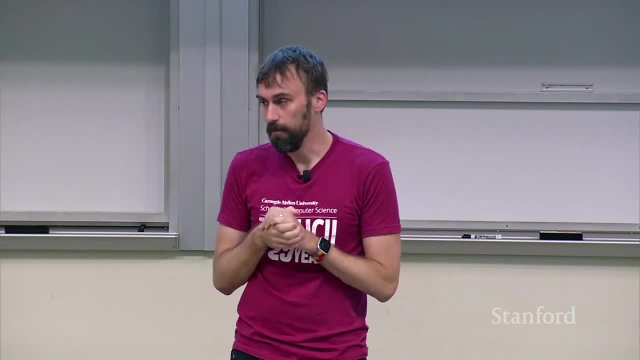 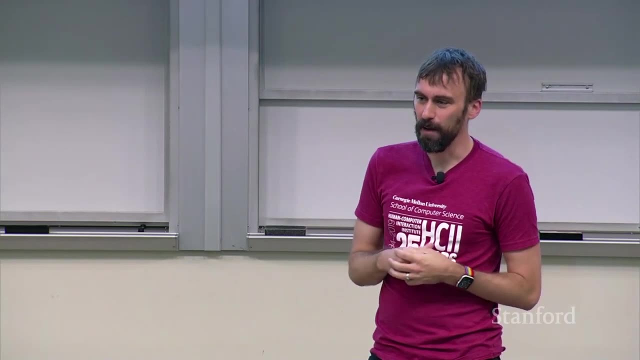 challenges, right? So ensuring every single app is accessible, all these things. As to why companies don't do more, I think there's a million different reasons, right, Although I did allude earlier back to this idea of is accessibility a value or not, right? 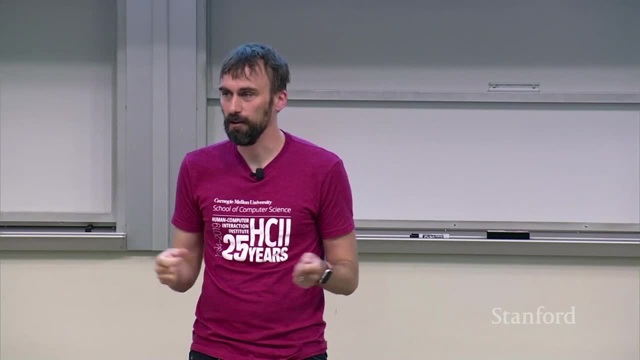 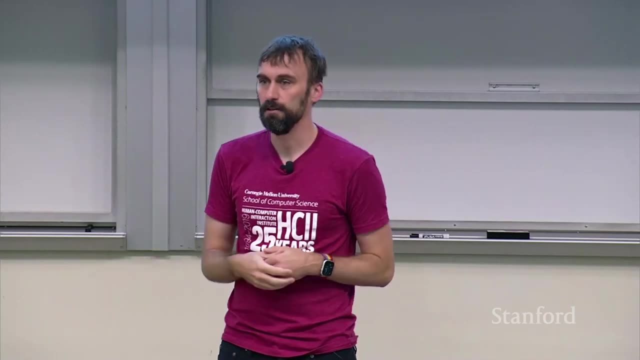 So it used to be kind of popular for people to make this economic argument. you know, you have a certain number of people with disabilities, you have people who are aging, who you know, in a variety of ways, would start to benefit from accessibility features. 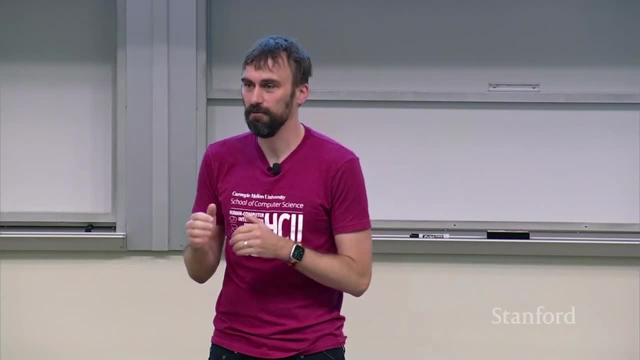 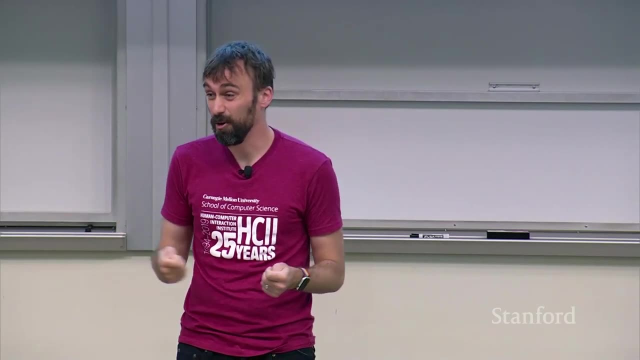 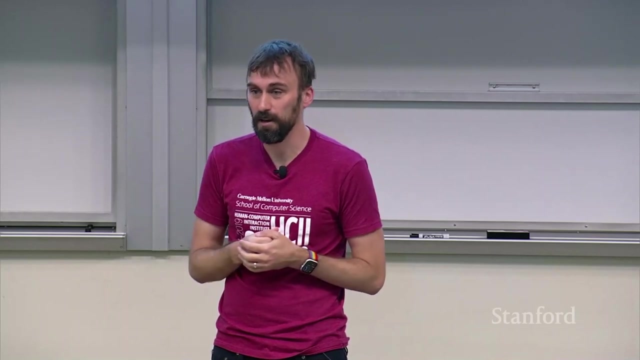 I am less convinced that that's the way to go. I really think it's. is this a value or not? There's certainly policy, legal reasons why people might want to ensure that their stuff is accessible. So you know, nothing that you would plan to sell to education markets will get passed. 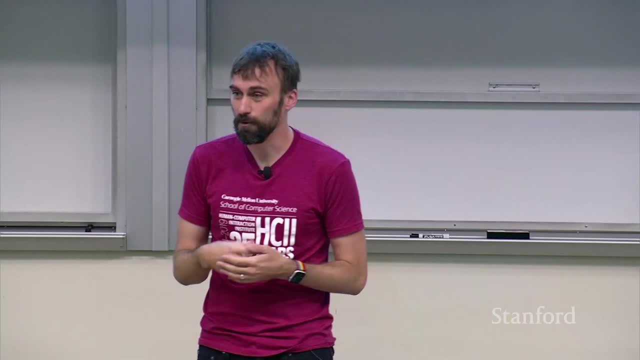 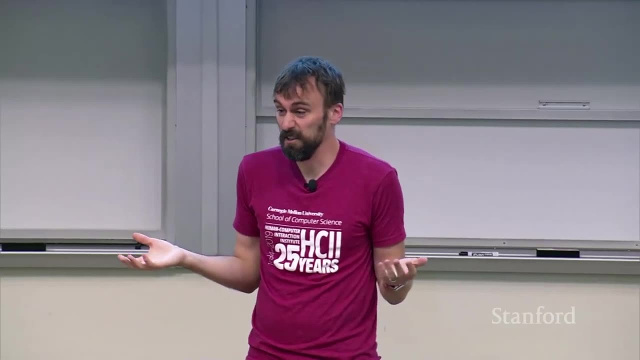 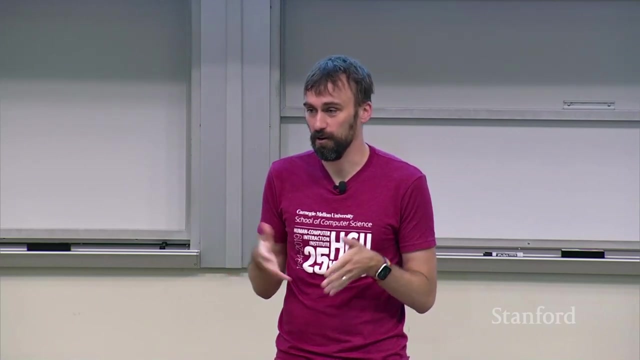 without being, at least in theory, accessible. There was this great example of, I think Amazon had tried to sell Kindles, You know, to all these universities and they didn't have an accessible experience or a plan or anything. And so the Department of Justice basically said: you can't use Kindles as your primary. 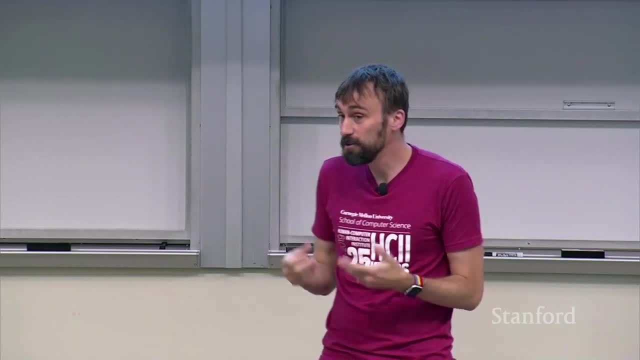 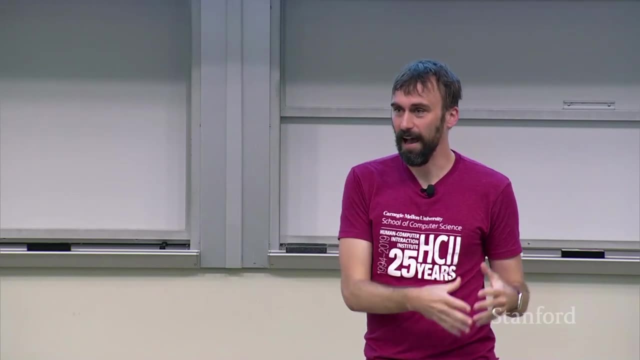 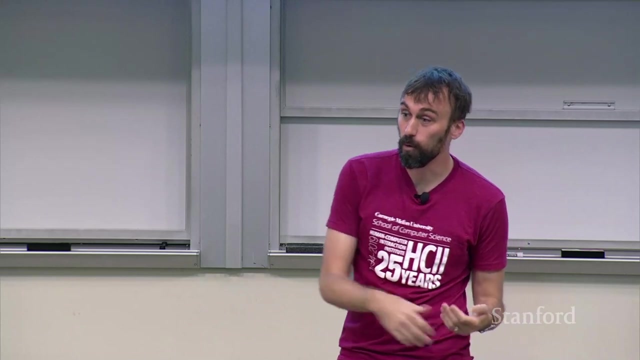 way of delivering textbooks. So there are those reasons, although it's amazing to me how people seem to really just resist this idea. So the Twitter example of you know hiding the adding alt text to an image down three levels of menus before you can even see that it's an option. 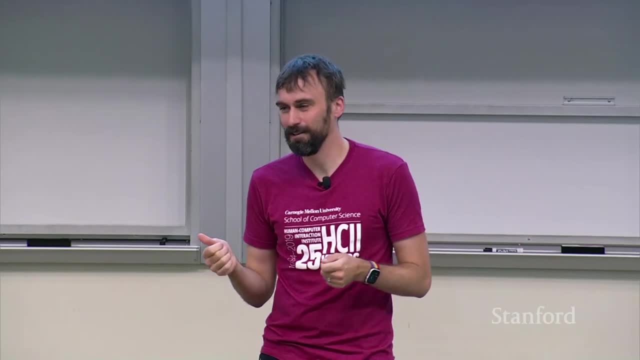 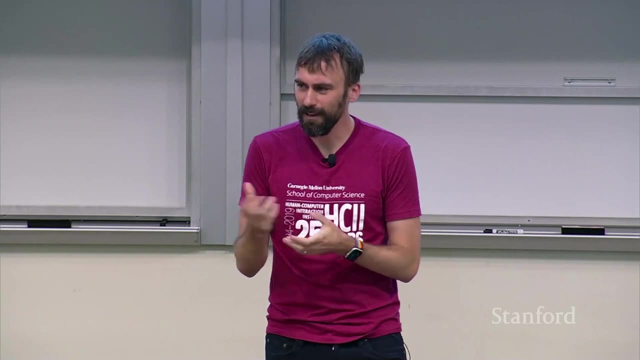 Or you know, recently- I don't know, I think it's Domino's Pizza. Domino's Pizza, you know, just fought tooth and nail against making their website accessible. And if you look, you know, if you look as a sort of reasonably competently technical, 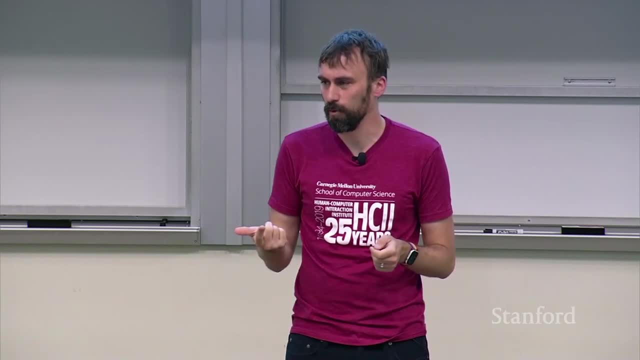 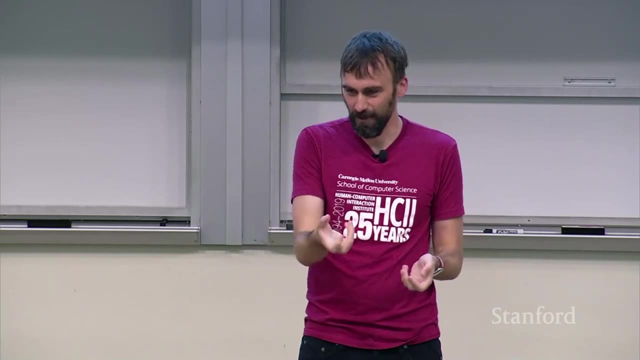 person. what they were fighting against was adding alt text and making sure that there were, you know, on click instead of on mouse down, because on mouse down assumes a particular input mode, like device, whereas on click can work on a mouse, or with the keyboard or with. 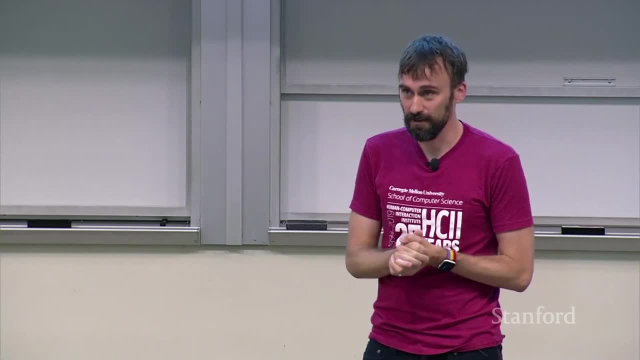 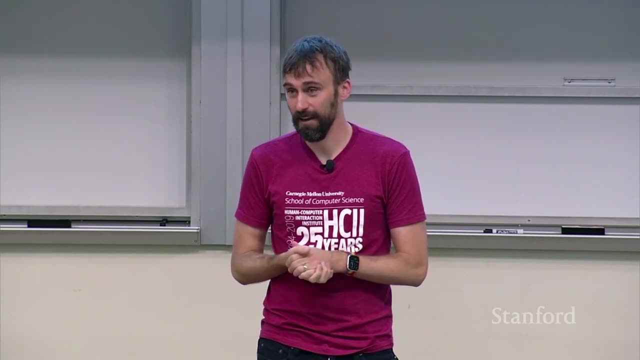 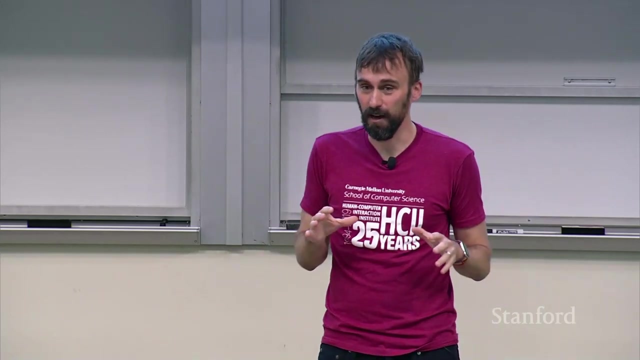 other things. So I don't know why that kind of resistance. It is certainly the case that it is way harder to do accessibility after the fact And so and it's not that hard to get this basic stuff right. Like I think it's fun like talking to lots of people about, like all these exciting new. 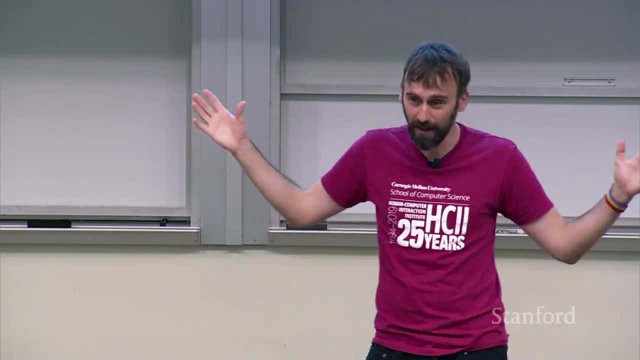 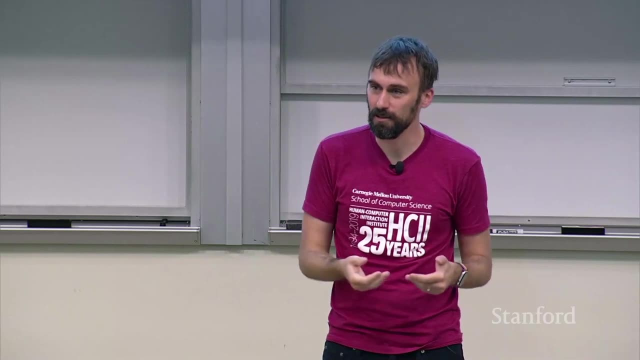 things we could do for accessibility. you know, like, what kinds of crazy new modalities could we expose? Like, what can we do? But like we don't have yet a reliable way to get people to put alt text on images. That's been a problem for 25 years. 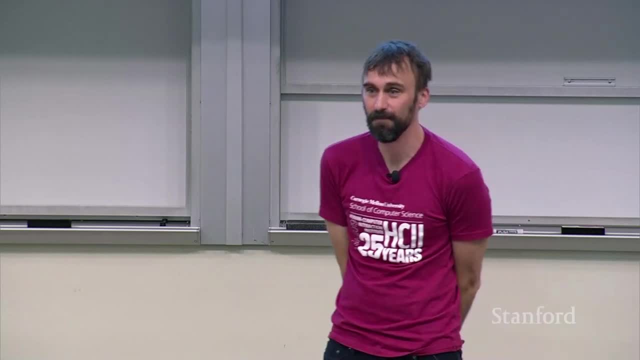 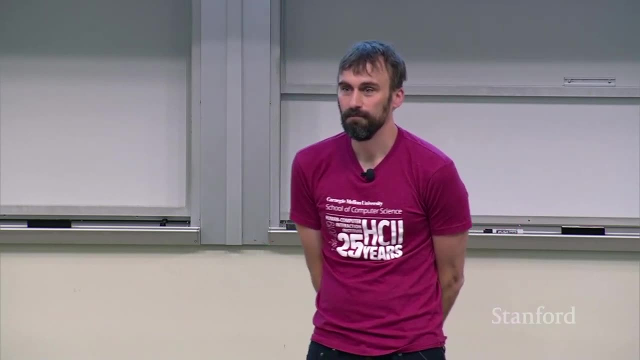 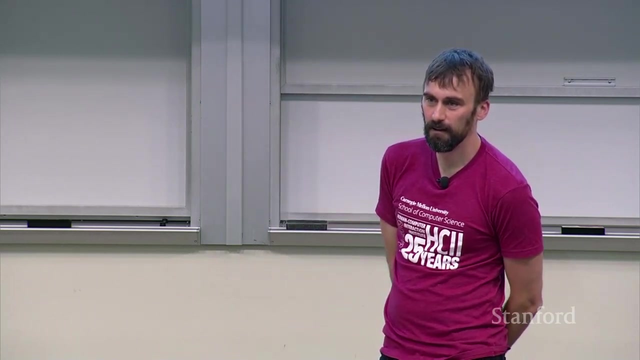 25?? Anyway, 25 years, So I'm not sure. Yeah, Related to that, what is your opinion- not as a lawyer, but as a professor or an Apple employee, or maybe not an Apple employee- of whether ADA requires this in interfaces? 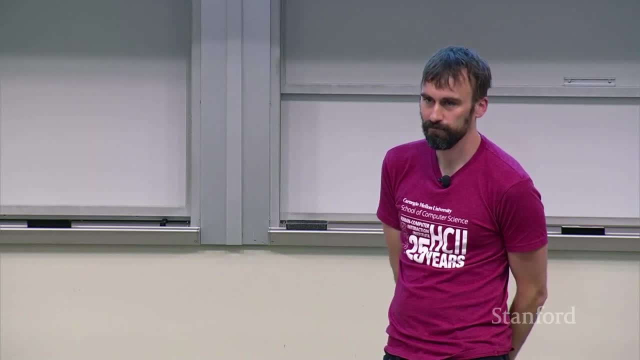 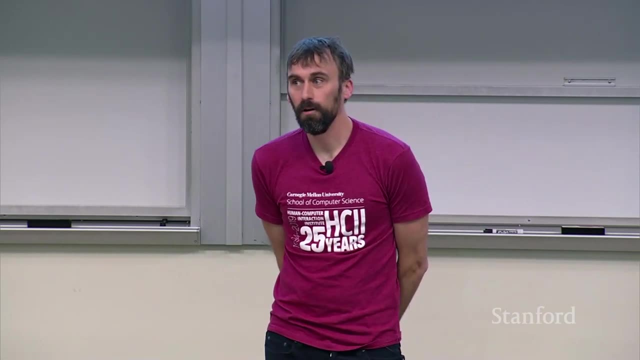 And where do you think this should be a legal requirement versus a value of a company? I know we had this discussion years ago, but I want to see. Wait, Yeah well, it probably doesn't surprise people that a lot of the legislation is a little. 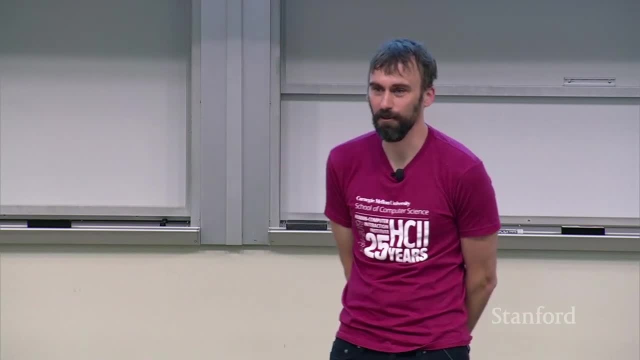 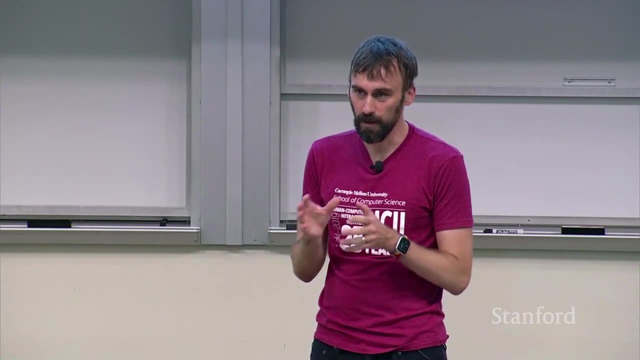 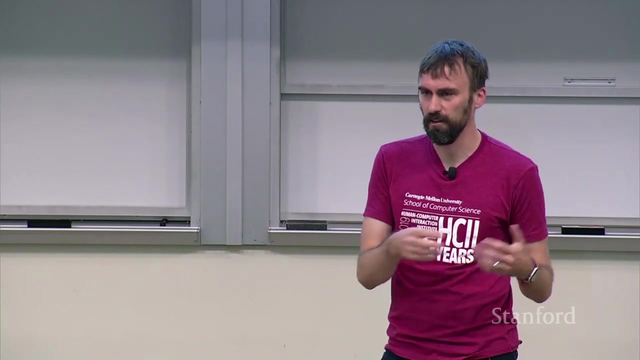 behind and probably hasn't completely grappled with that question. So there are. so Section 508 of the Rehabilitation Act says that government, anything used by the government, basically has to be accessible And that usually gets extended to, you know, public universities and other things. 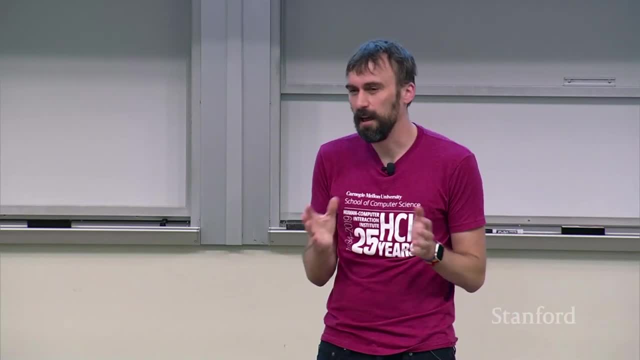 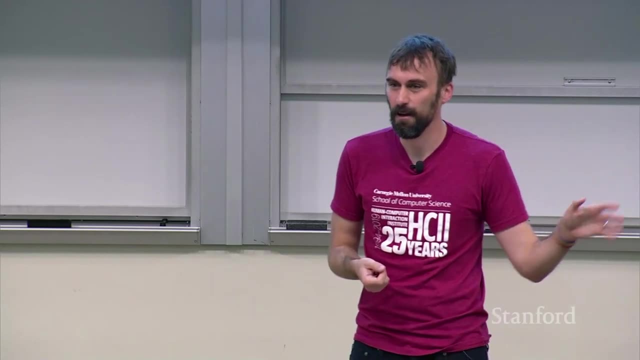 So anyone with contracts with the government, like what exactly that means to be accessible, right, Like it's always a little bit, you know, it's probably not that first-class experience that we'd love, right, But you have to have some way. 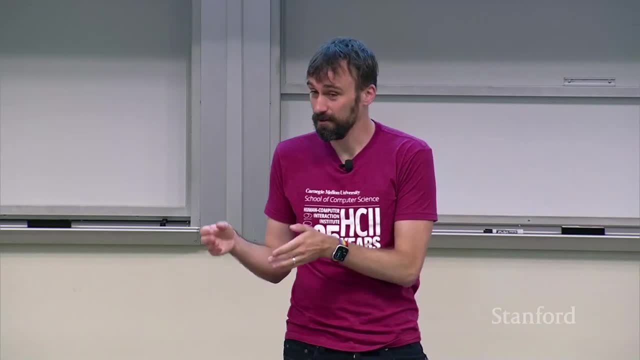 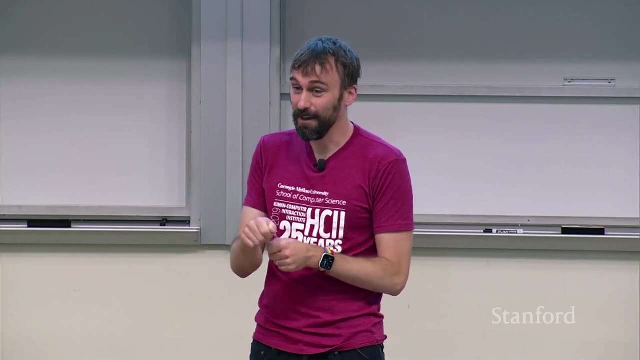 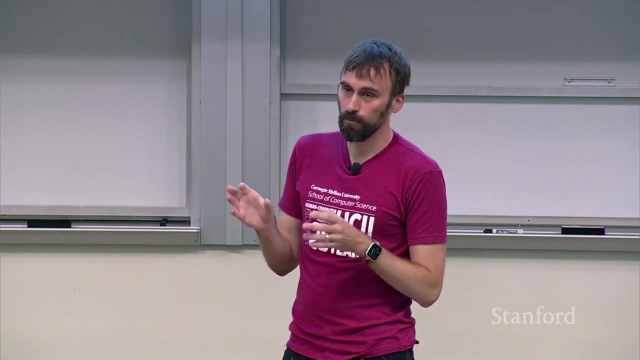 So that's one part of it: The private companies. so far, my understanding is that in the high-profile cases, where which have always been settled right instead of decided, which I think actually frustrates a lot of people- high-profile cases- it tends to be that the court will rule that the online 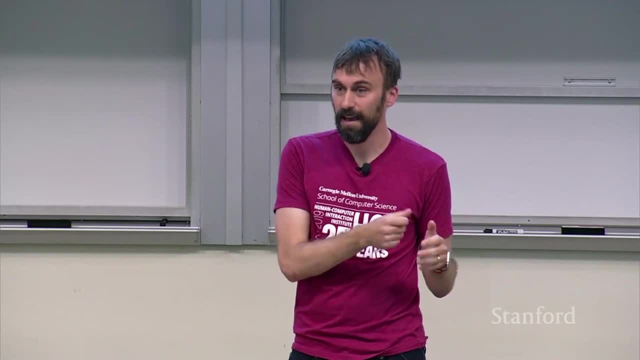 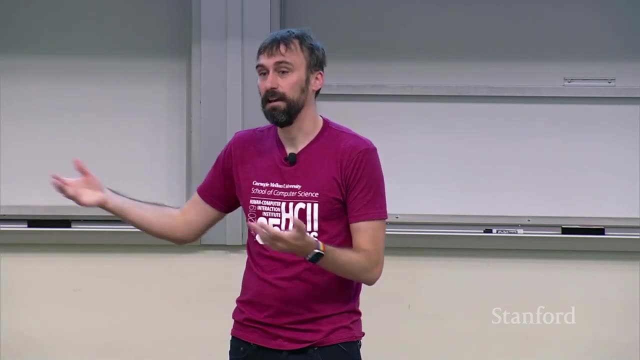 presence store or whatever else, is not accessible, Right Right, And that the online presence store or whatever else is an extension of something physical and therefore the ADA does apply. Once that happens, then the ADA seems to apply and you can't exclude people. 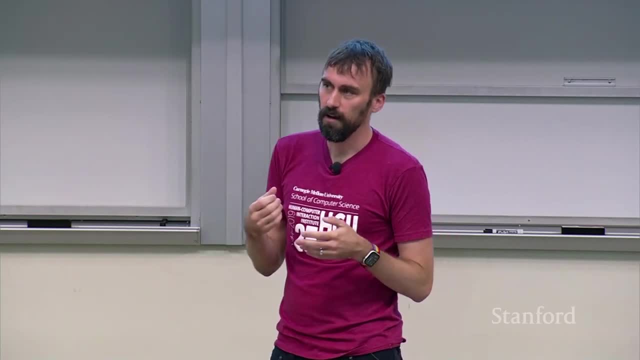 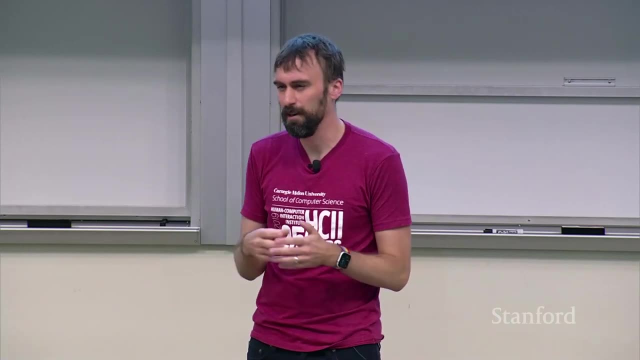 So I think in another high-profile case- Target in Target this is a few years ago- they had some offers that were only available on the website that I think you maybe had to redeem in the physical store. I'm not sure how it works. 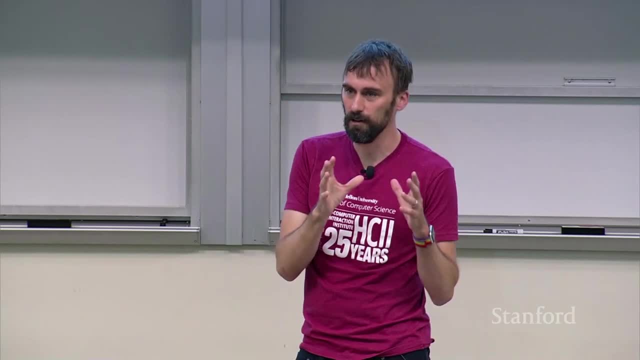 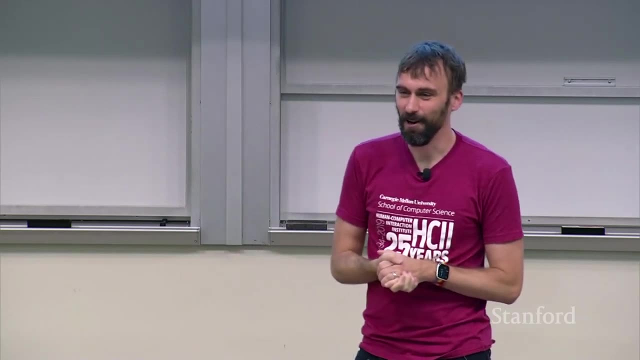 And then with you know, a pizza shop, it's probably pretty similar, right? You've got the online thing that connects to this physical pizza shop. There was a time when, you know, we thought that we would get some more clarity on this. 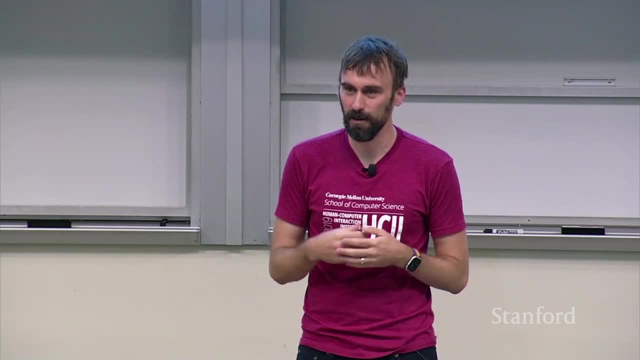 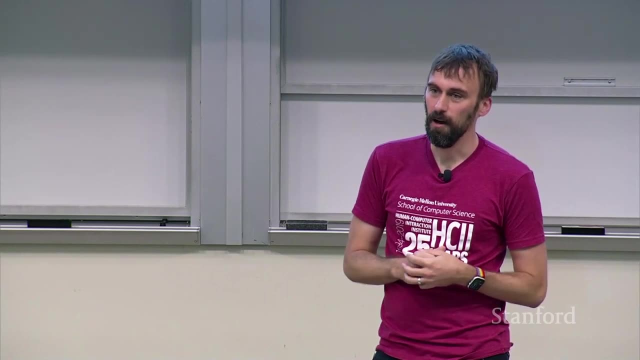 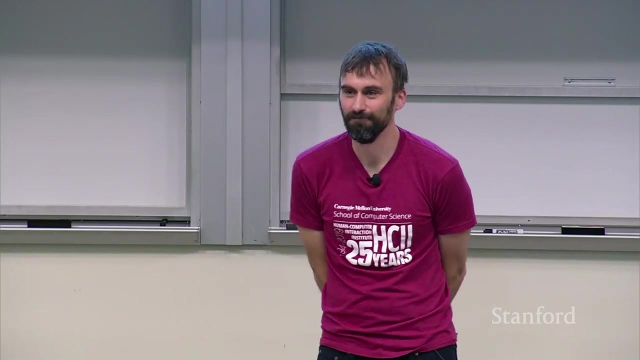 so in a prior administration there was a little bit more momentum toward the Department of Justice putting out some actual guidelines, but we haven't seen that yet. Is that the end? Is that? Did you have a second part? Is that good? 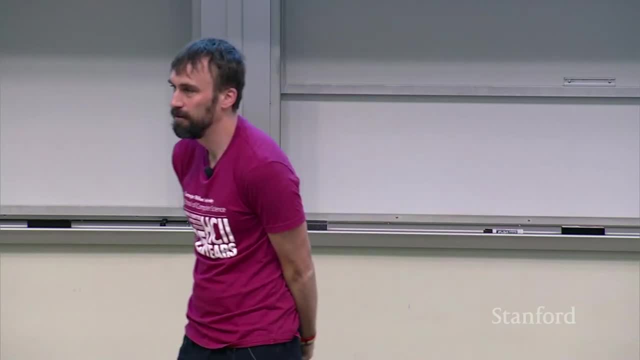 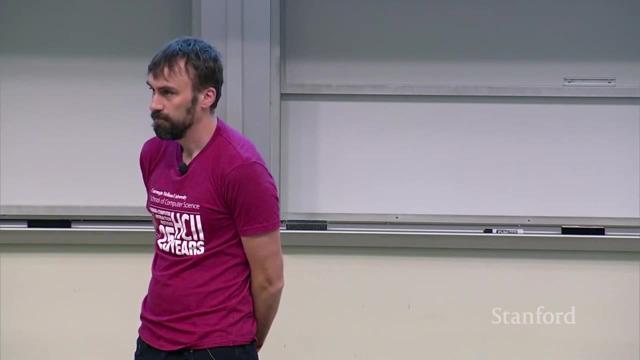 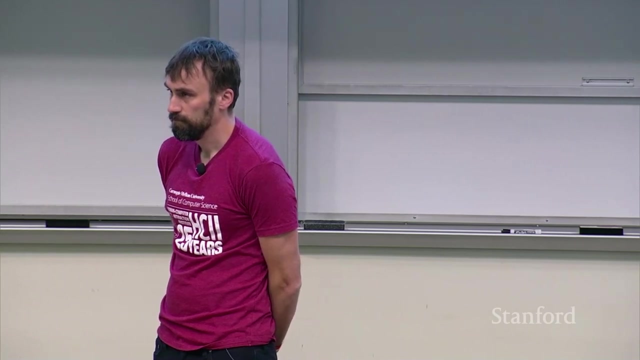 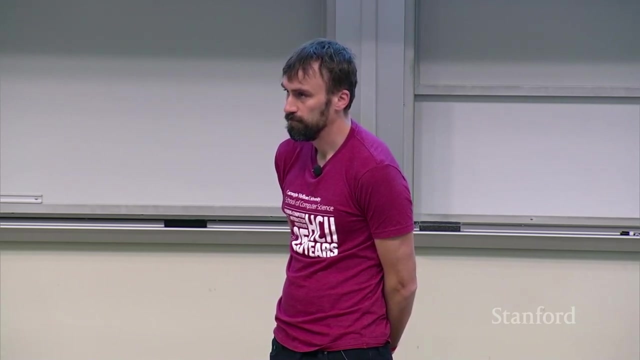 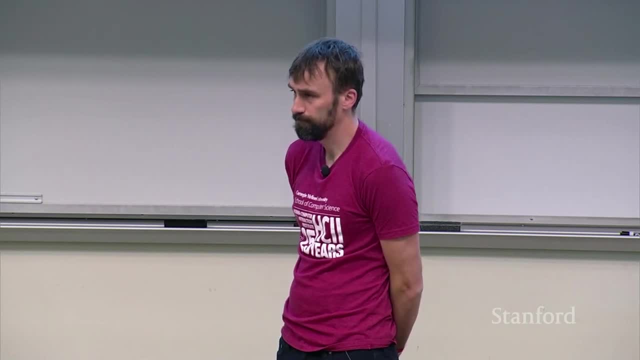 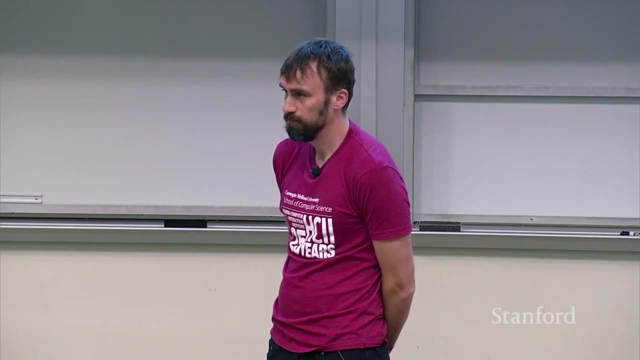 cultural understanding. so they're therefore very marginalized still, especially, you know, augmented by their lack of inclusion in technology. and how do you think that affects people's lack of adoption of that feature versus the technological readiness of its accessibility- below the picture, and how do you think technology can drive their inclusion or people's awareness of the need to? 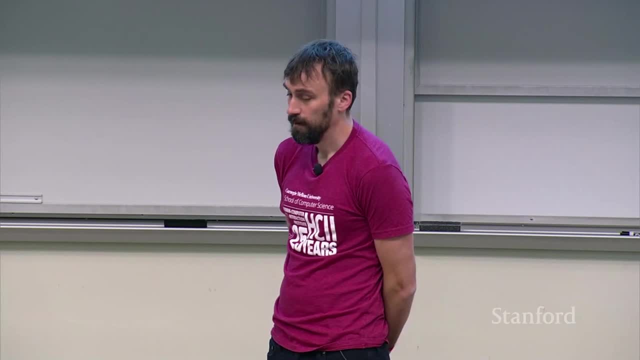 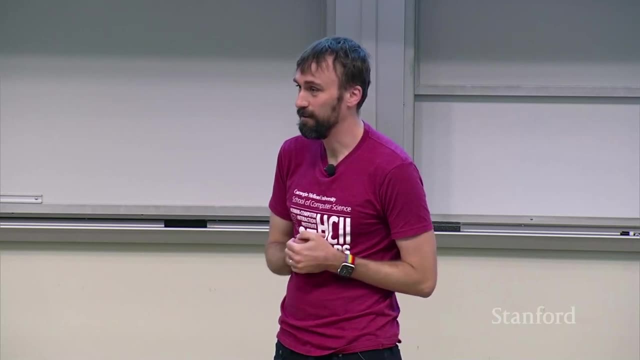 less marginalize that group. It's a really fantastic question. I will say that one of the great things about working accessibility is that I've gotten to work with a number of people who think about these issues much more deeply than I was ever prepared to do. 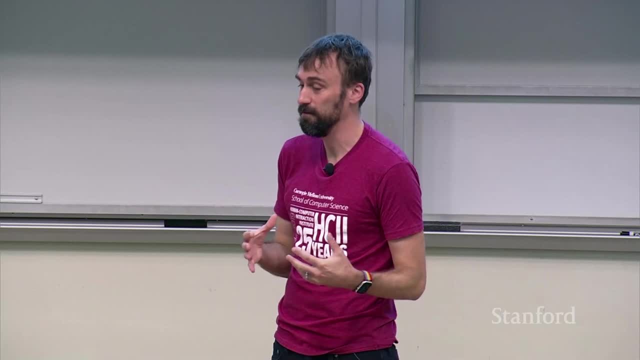 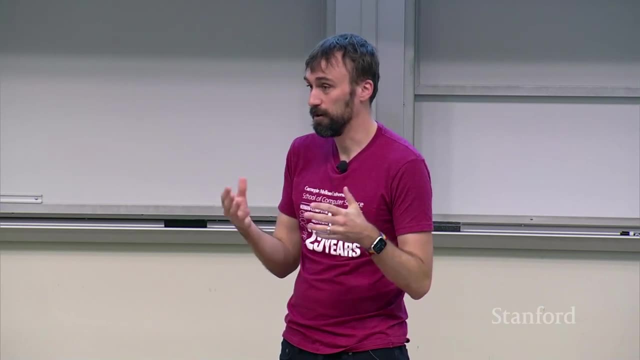 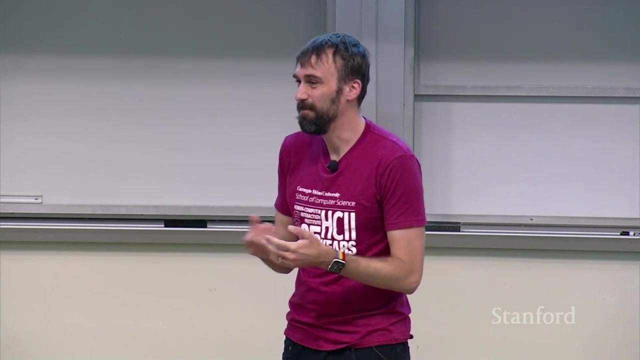 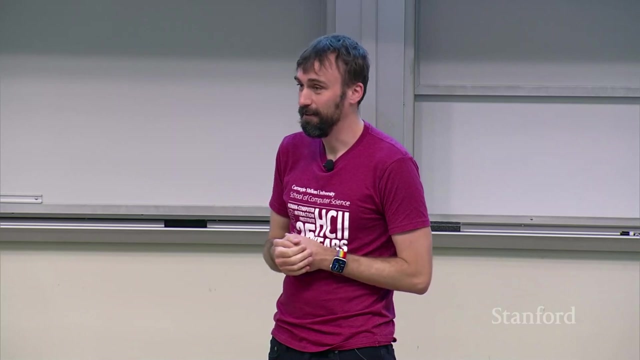 and so I think it's a really important part of that perspective. I definitely agree that one reason why it's not out there more is that people don't seem to know that this is a thing. It's amazing to me like I was once requesting accommodations for a student and you know we winded up talking to. 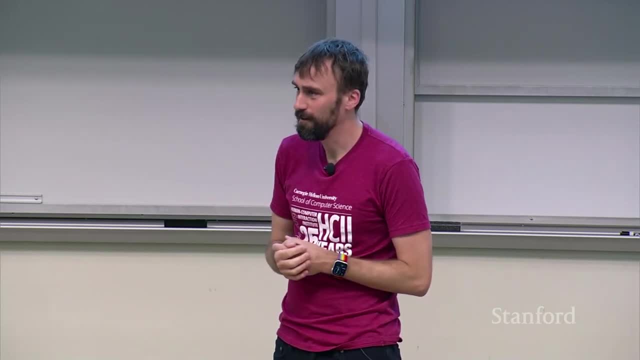 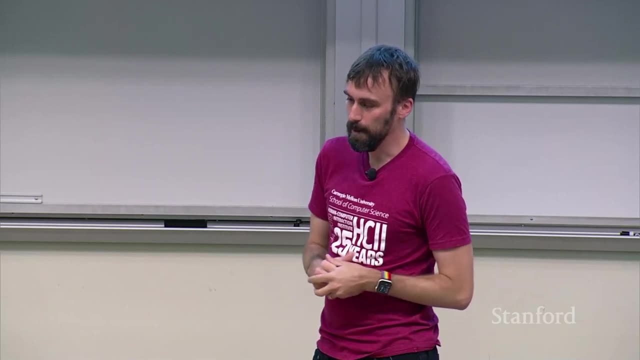 like a vendor and the vendors like, wow, no one ever asked me to clearly somebody. it was a big vendor. you know like clearly somebody else has had this problem but it's not documented, it's not somehow out there. I don't know how we overcome that, but I definitely agree. 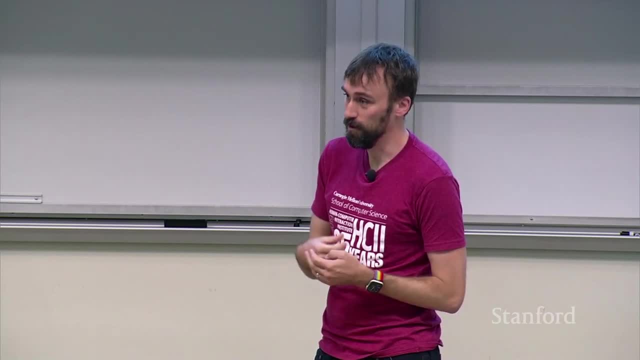 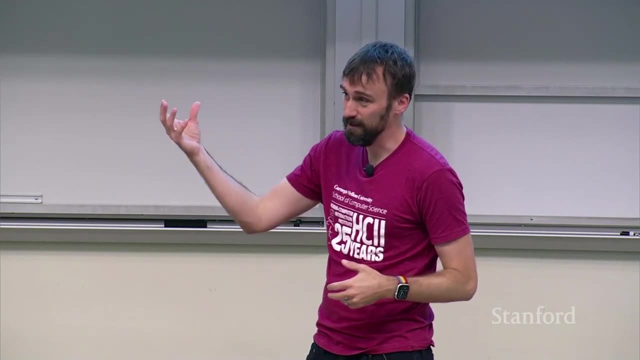 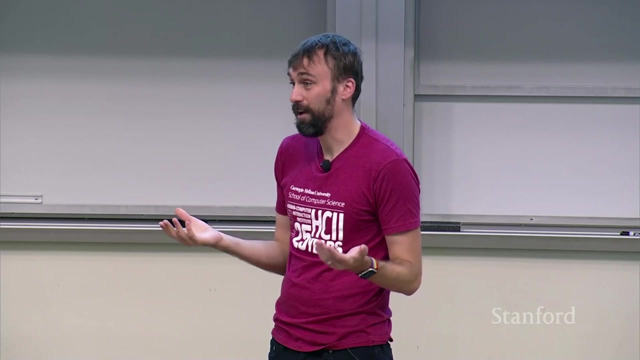 that it's part of the equation, right? so you mentioned kind of policy. you know I am very squarely in the technical side of things and I think advocacy is this, you know, the other kind of leg of the of the stool to make this actually work. but I don't have great ideas about how we do it. People do band together on social 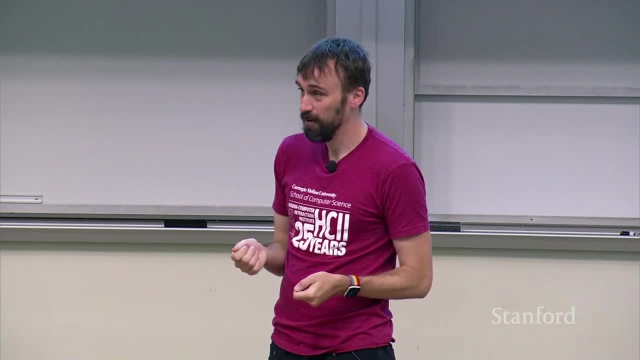 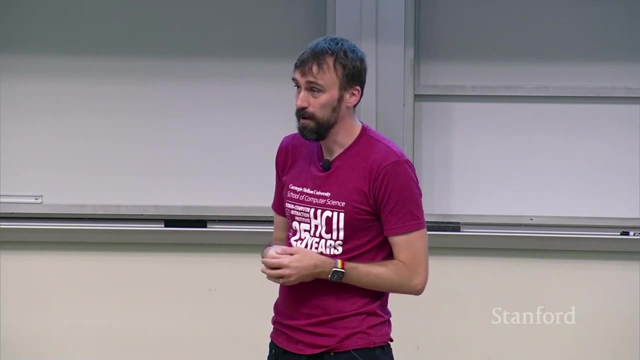 media. I think it's one of the ways you can kind of point at successes where you know you can get people that are more geographically dispersed to kind of come together around certain issues. but you know it certainly hasn't hasn't, you know, solved everything. 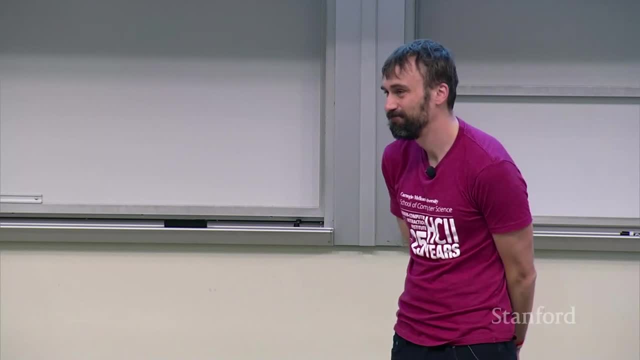 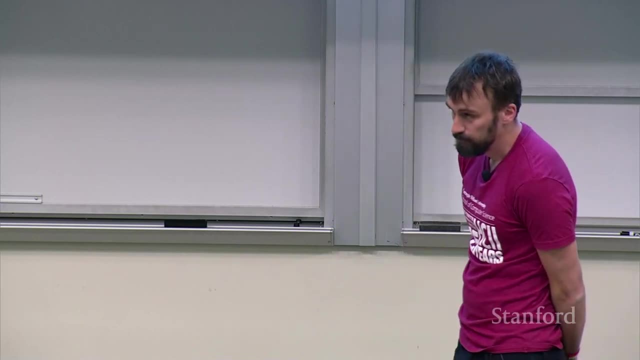 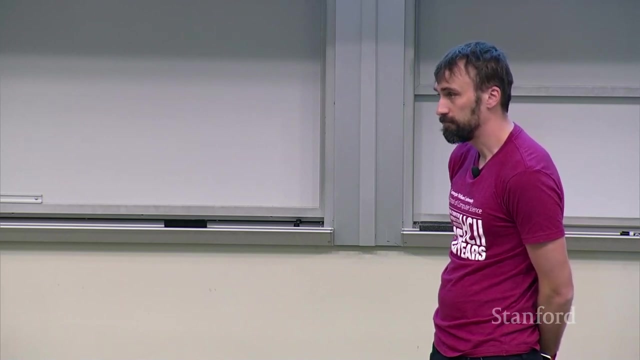 Great question, thanks, Yeah, Last question, Last question. So you did present a little bit of crowd sourcing as an alternative, where other humans are man in the middle or like human in the loop. Couldn't we like, Mm-hmm, like, make this more like? 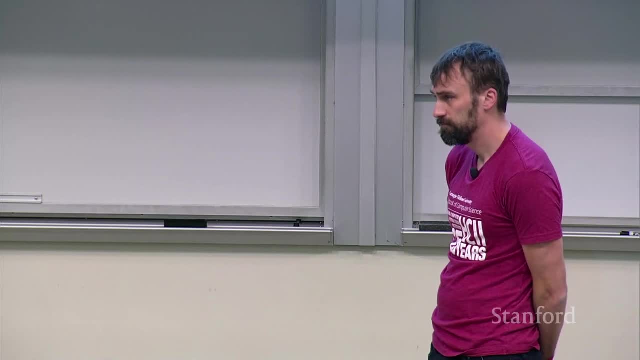 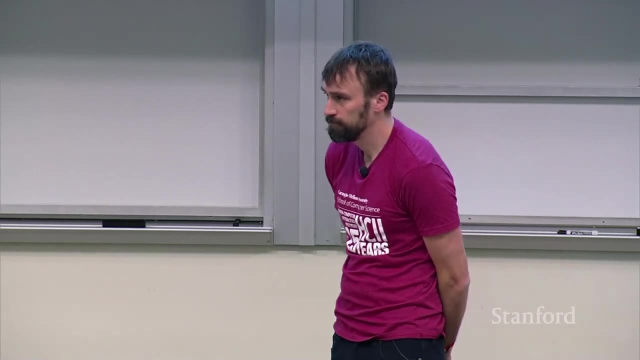 a social, like you know, discussion. I mean right now it's a machine- human interface discussion and that's important. but you know we live in a society with a bunch of people. should we start creating like systems where humans are more active supporting each other? and I'm not trying to imply anything. 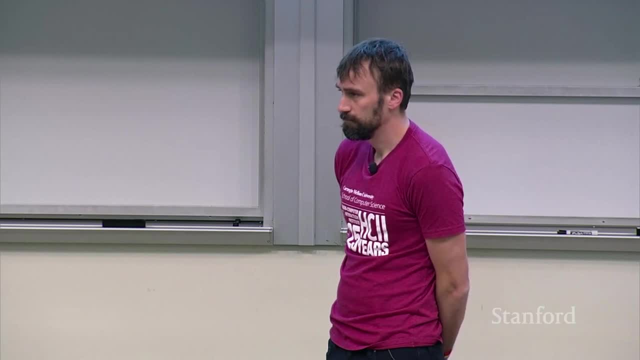 like. you know that anybody wants to do or not, but clearly we are always looking for support from other humans. and now we're basically in the machine. we're doing all these very complicated techniques to try to like avoid. maybe with a human on the side it would have been easier. so 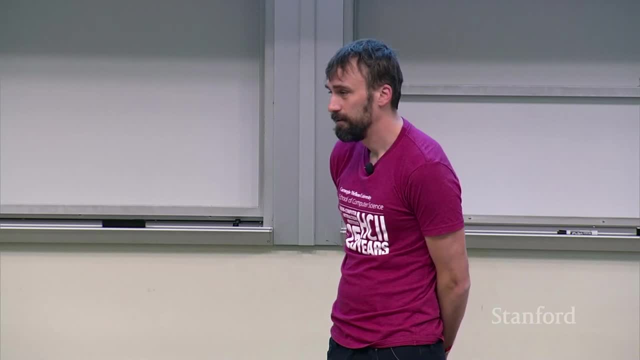 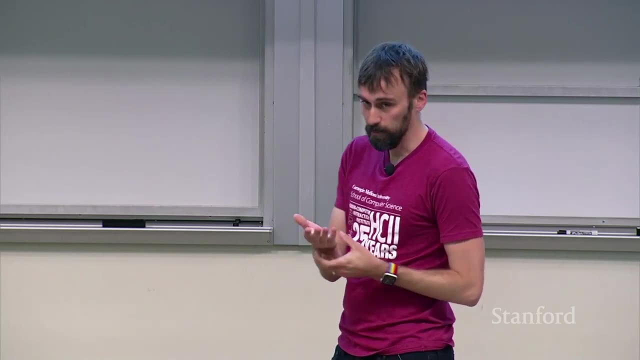 but I'm talking about a systemic approach, just like finding a kind soul that comes and helps us. yeah, I think it's a really great question. a lot of the work that St Michael was alluding to was very much oriented toward making those connections right and whether that's paid crowd workers. 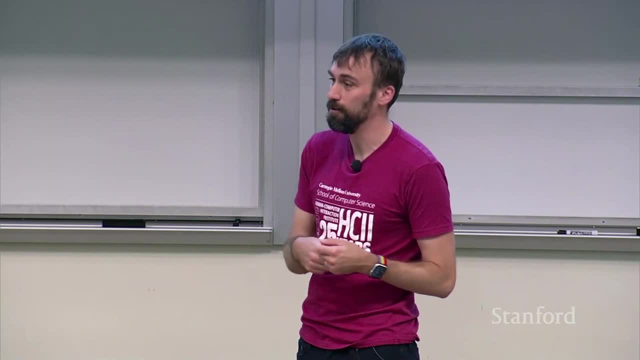 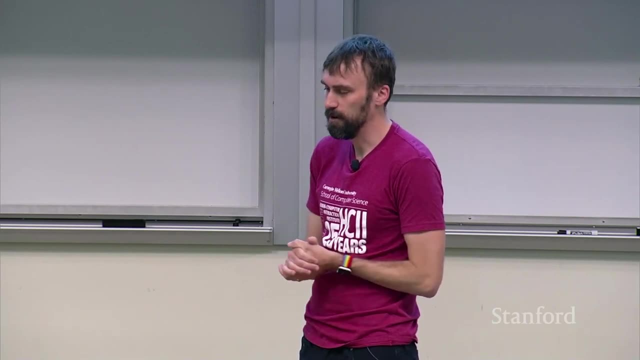 or we also had, you know, systems that would connect volunteers on Twitter to do different things that you could do remotely. one of the bits of recent work that I really like and I've taken inspiration from is from Cynthia Bennett, who is at University of Washington, actually at CMU with me and now as a postdoc.